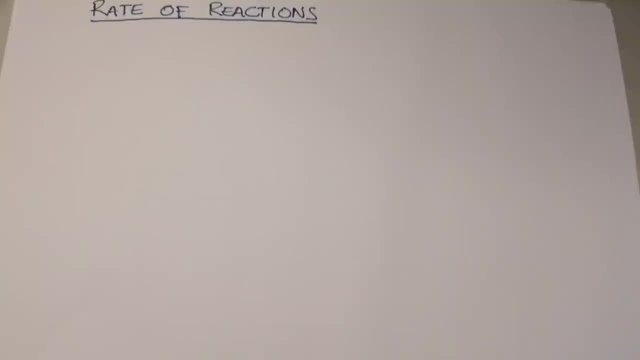 you Now my approach is going to be a little bit different today, as much as I want to go through the voluminous, you know, amount of explanations about the theory part and all of that. But I just realized that that could take us quite a while. So my thoughts were that I'll just cover the 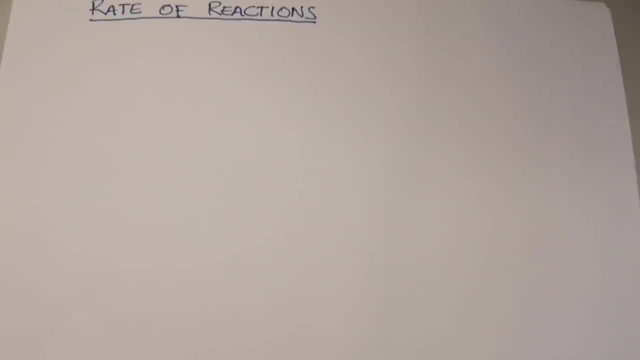 theory briefly, and thereafter just quickly just delve into the question. I don't want you falling asleep in the process of watching this video, So I hope that you enjoy it. Okay, if you haven't subscribed, please do so. Just make sure that you hit that bell button. 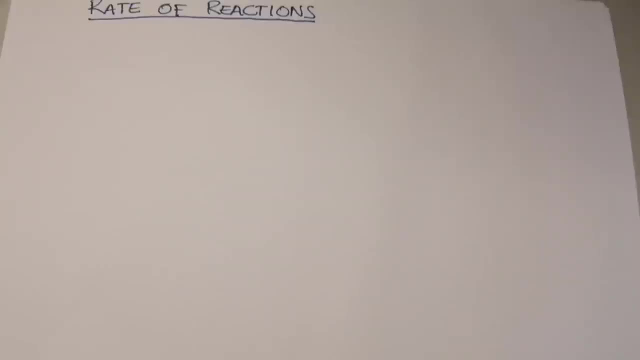 so that you can always get notifications when we've got a new video. that's coming. All right, ladies and gents, and if you need to get in touch with me, please, my email still remains. that's mlungisimngosi at gmailcom. that's m l u g m g i s i dot m for mary dot. 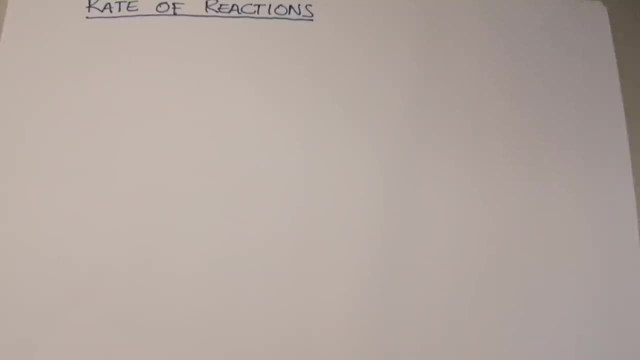 n k o s i dot com. All right, let's get into it. So, when we talk about rates of reactions, or rate and rate and extent of reactions, what exactly do what does it entail? So, first of all, I want you to notice there's just some things that we need to understand about what. 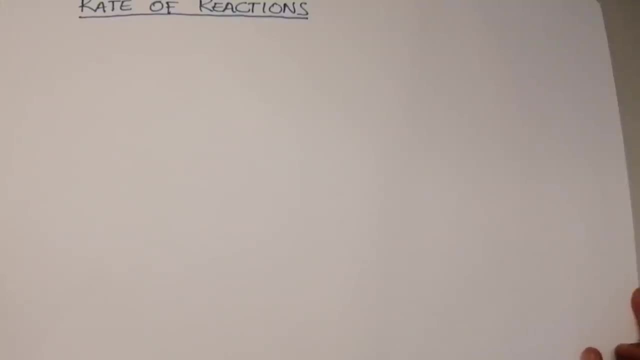 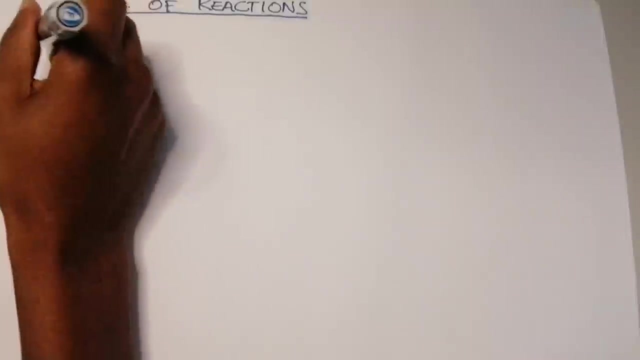 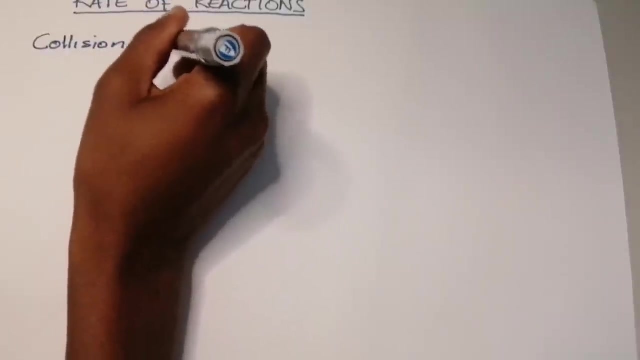 does it take for a reaction to take place? Right, so in this case we've got what we call the collision theory. Okay, and the collision theory simply states, or let's just write it down there: So the collision theory simply tells us that, in order for any reaction to take place successfully, 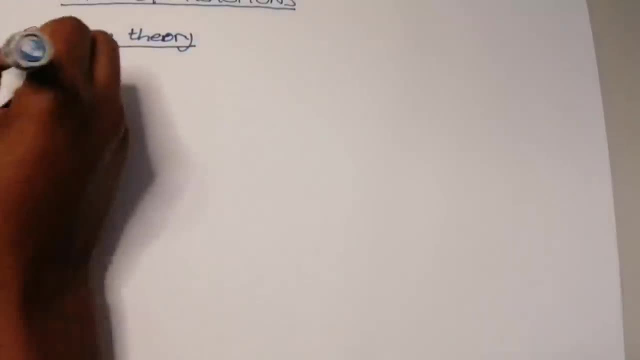 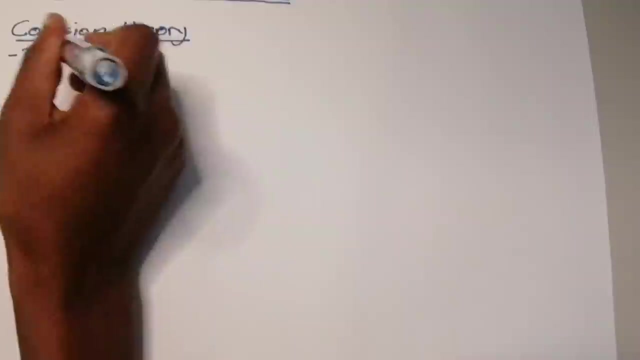 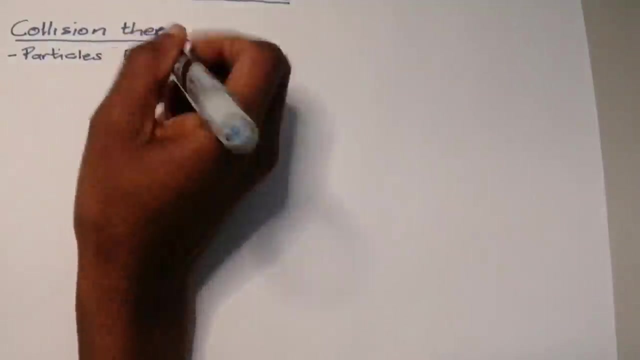 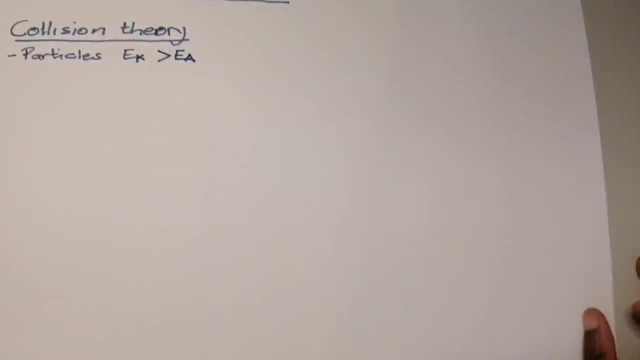 right, there's a requirement. First of all, particles must have sufficient kinetic energy. Particles must have. Now, what do we mean that sufficient kinetic energy? It means that kinetic energy must be greater than what we call the activation energy. Now, what is the? 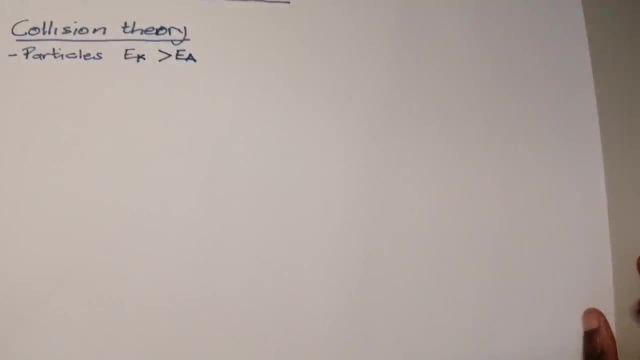 activation energy. That's the minimum energy required in order for a product to be formed, in simple terms, So that's the minimum energy required in order for a reaction to take place. So if we have a reaction to take place, So if we have a reaction to take place, So if we have a 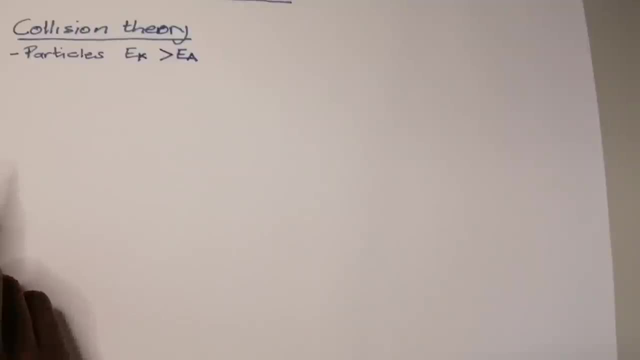 in this case. So, in order for any reaction to be a successful reaction, that is, in order for products to be formed, we must make sure that particles have got sufficient kinetic energy, That's kinetic energy that's greater than the activation energy. And secondly, we say that they 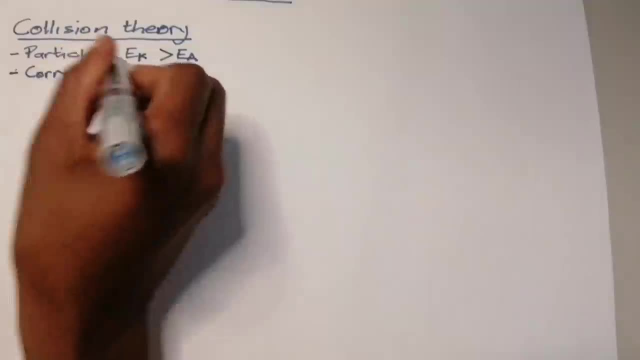 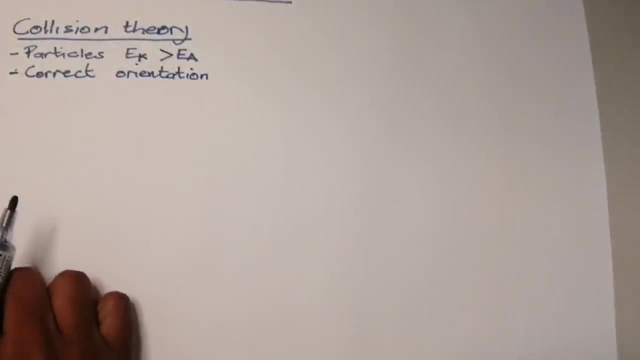 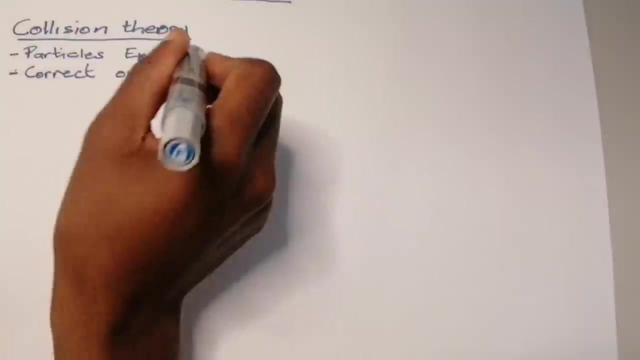 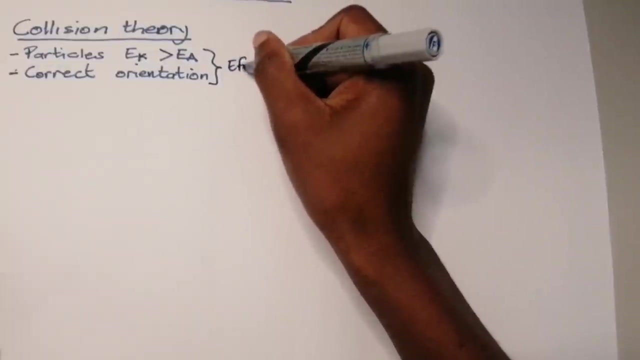 must have a correct orientation. Correct orientation: Okay, Right Now. if these two conditions are met, then we know that this results in what we call an effective collision. So a combination of these two together results in what we call an effective collision. What is an effective? 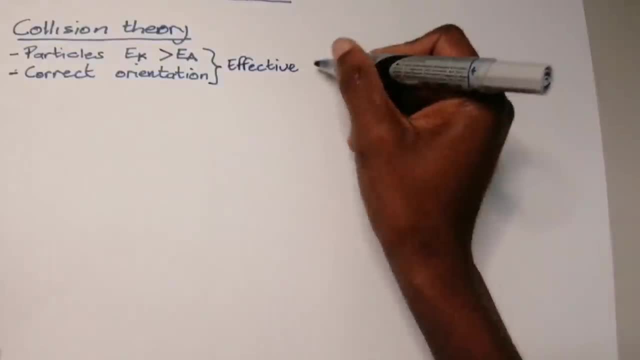 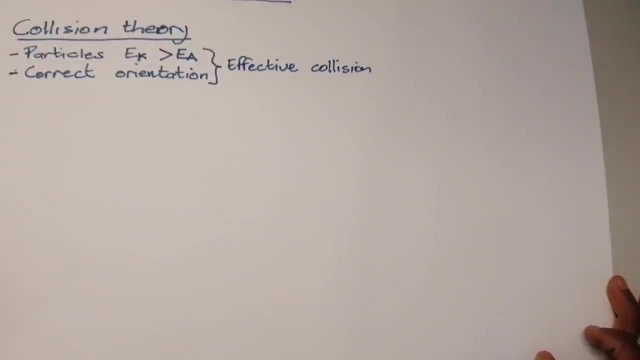 collision. Well, it's an. it's a collision whereby products are formed, or that results in products being formed, So an effective collision takes place Now In this case. So we say: this is what the collision theory entails, Right? So in a sense, we want to make: 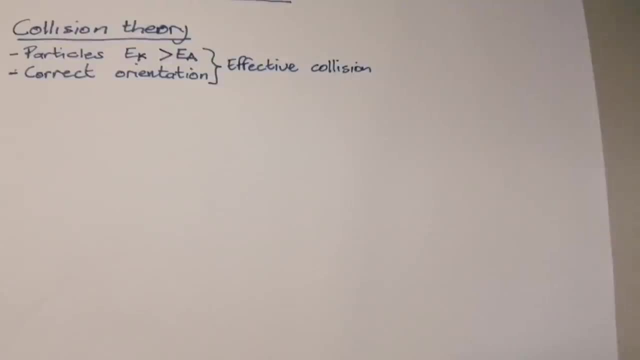 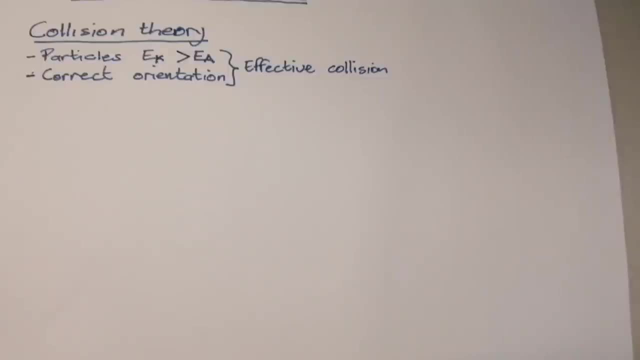 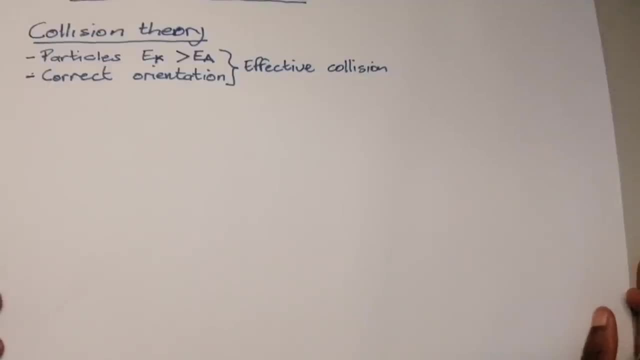 fact, what do we mean when we say rate of reactions? Well, we say: this is the number of moles, OK- of products formed per unit of time. Or you can say: this is the change in the amount of products formed per unit of time. or you can even use reactants, right, because, remember, you use reactants. 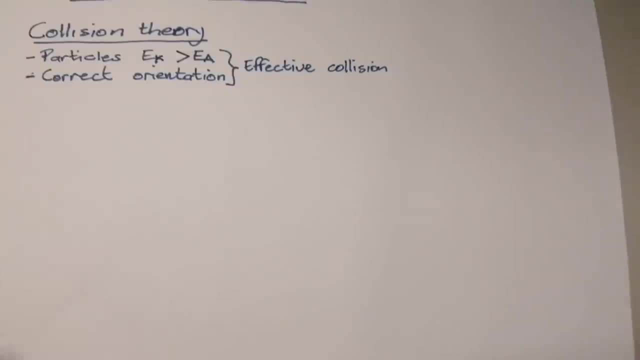 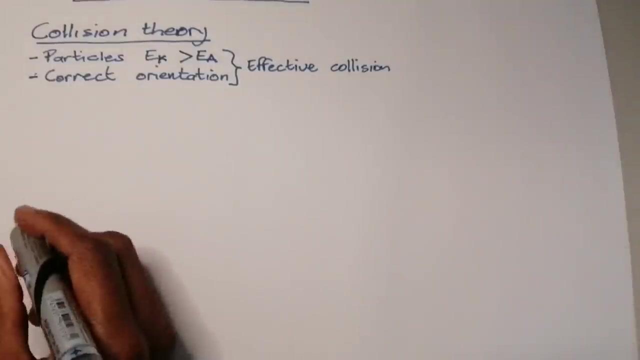 to form products. so it's. it could be also the change in the amounts of reactants used per unit of time. okay, so in this case, how do we improve the rate of a reaction? okay, so we say that there are five vectors that affect the rate of a reaction. all right, I'm going to actually exclude. 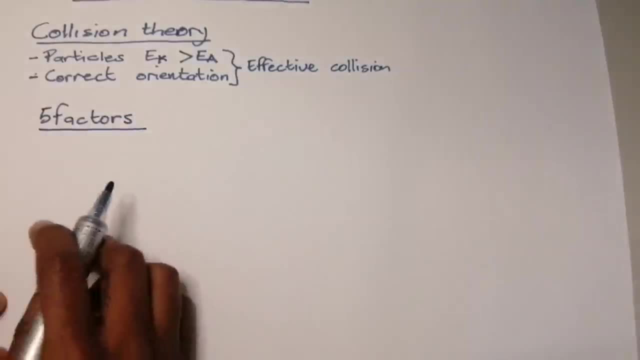 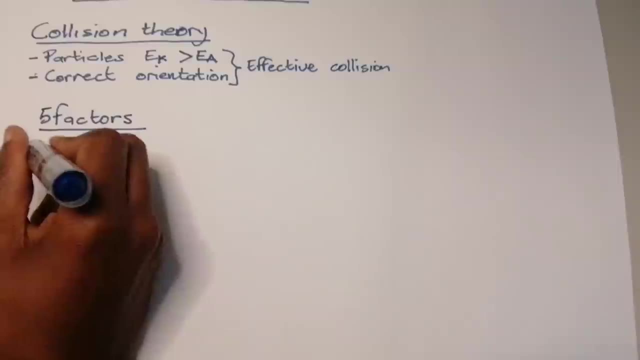 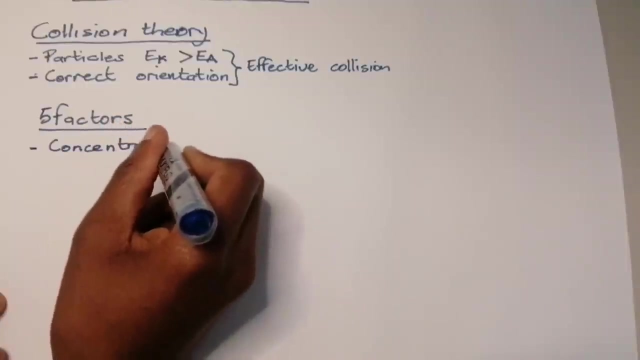 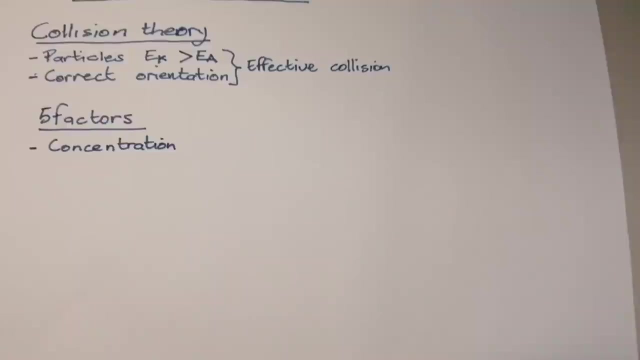 one of those vectors. okay, they don't ask about it much. so we say that there are five factors that affect the rate of a reaction. all right, so the first factor is concentration. okay, so right. so the first factor that improves the um, the, the uh, the rate of a reaction is concentration. all right now, if you. 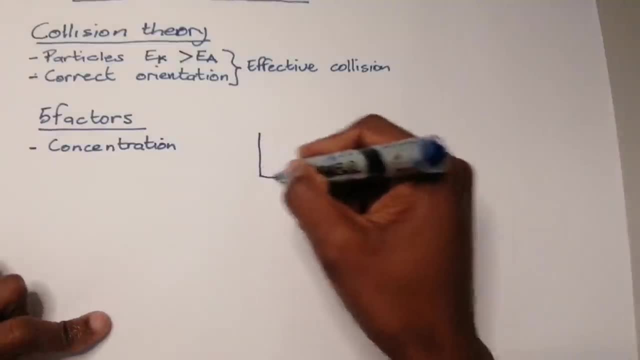 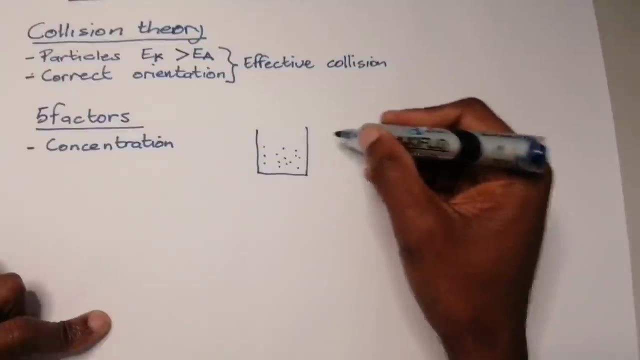 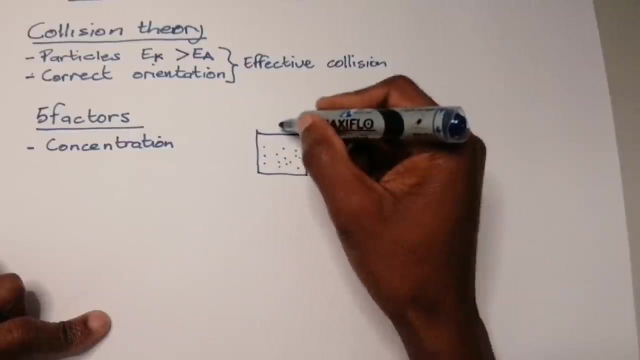 want to think about it. when we talk about concentration, we are talking about the number of moles. okay, that are the per unit of volume. so if you take, for instance, uh say maybe there's beaker a and beaker b, okay, so that's a, we close it there and we've got beaker. 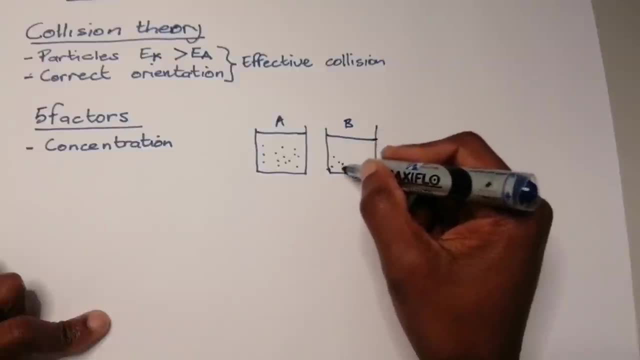 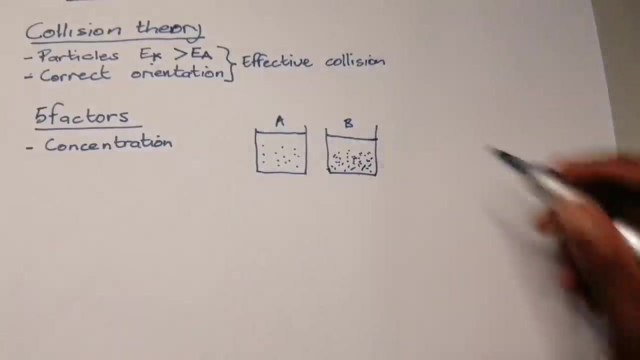 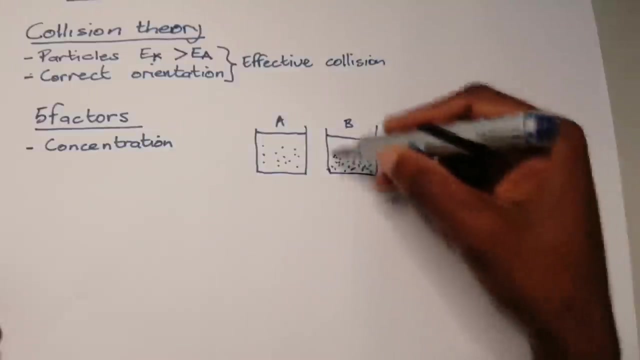 b, assuming that they are equal, right. so if i've got more particles of gas here, all right. within this beaker, in this case there is a higher concentration of um of that particular gas per- i mean per unit volume. so if the two volumes are equal, so in this case this is more highly concentrated, right. 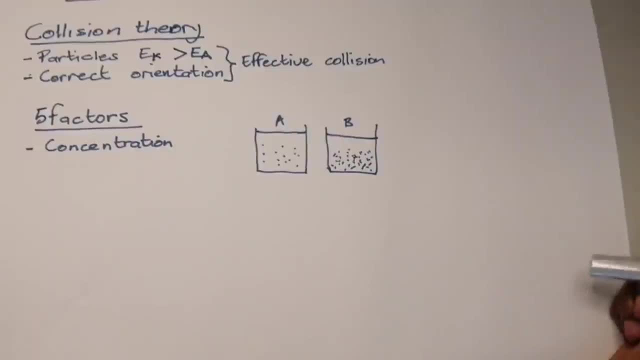 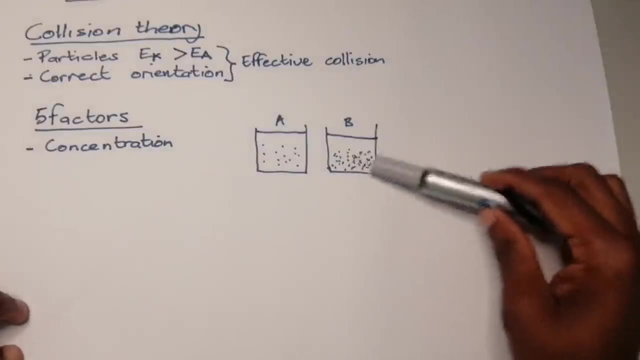 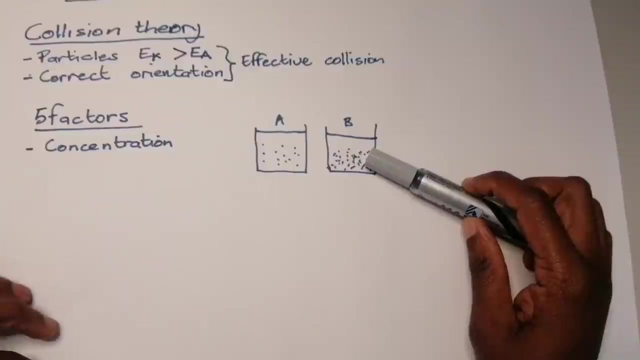 now think about it. why would concentration um increase the rate of a reaction? okay, so the higher the concentration, the more particles there are, right, the more chances of collisions taking place per unit of time, isn't it right? so it means more collision take place, right? so in this case it. 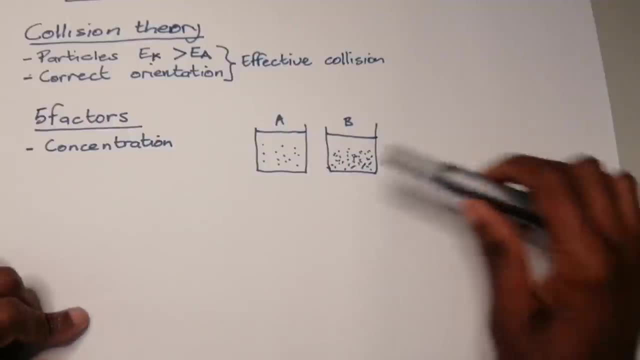 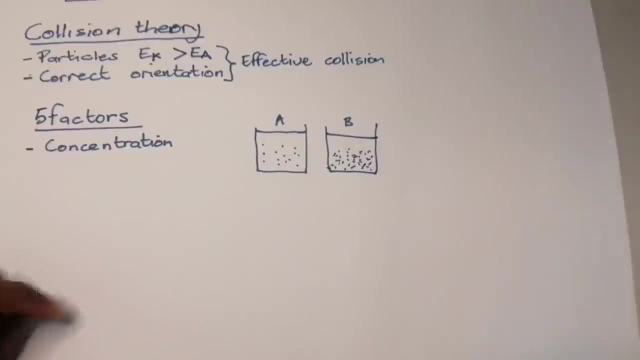 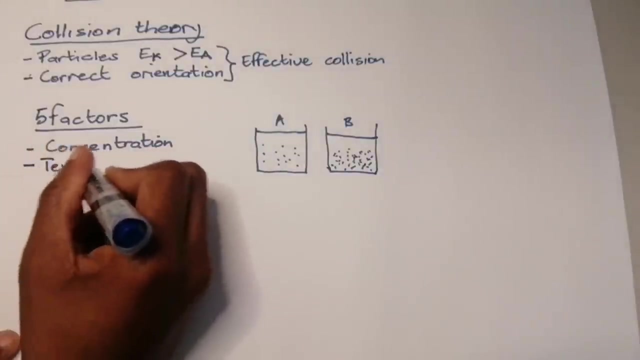 would result in, uh, the rate of a reaction. so, obviously, collisions, that more collisions are taking place, there'll be more chances of effective collisions taking place right per unit of time. and then the second factor: we say it's temperature, right, so, um, the next factor that affects the rate of a reaction. 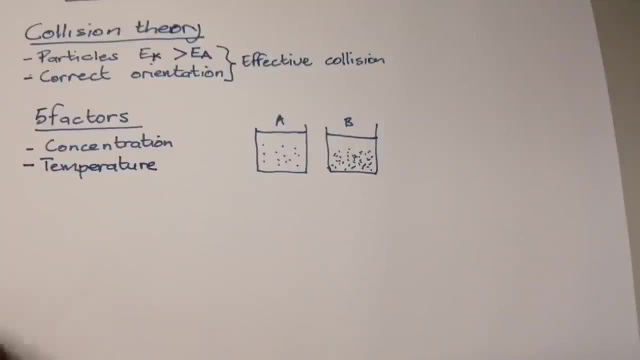 is temperature right now. what is temperature? it's the measure of the average kinetic energy. now, think about it. in any particular reaction, it's the measure of the average kinetic energy now. um, so in this particular uh uh for any reaction to take place, we said that the 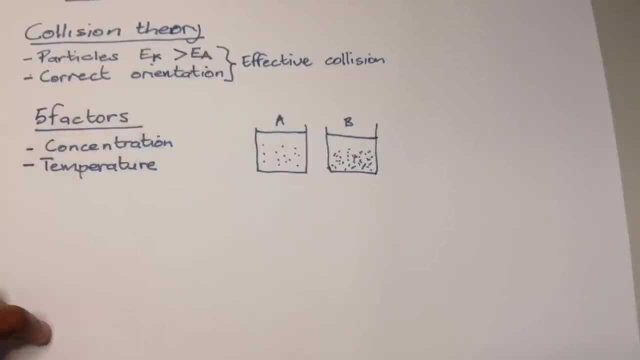 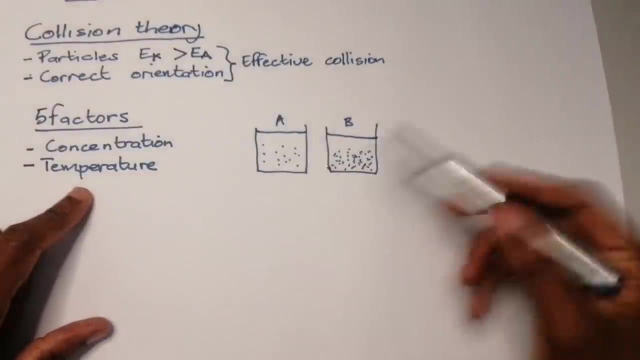 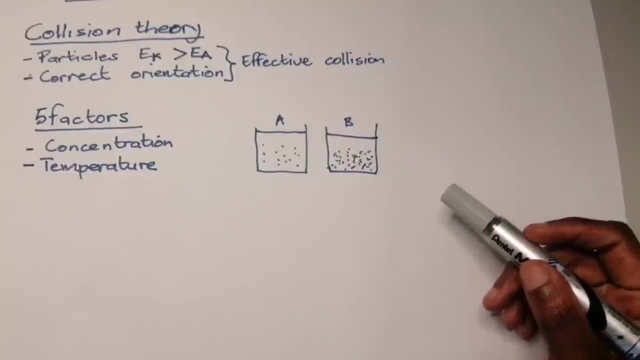 particles must be moving, isn't it? so in this case, they must be moving with the kinetic energy that's greater than the activation energy. so what we're simply saying: when you increase the temperature, you are causing them to move even more. right, it means their average kinetic energy now becomes: 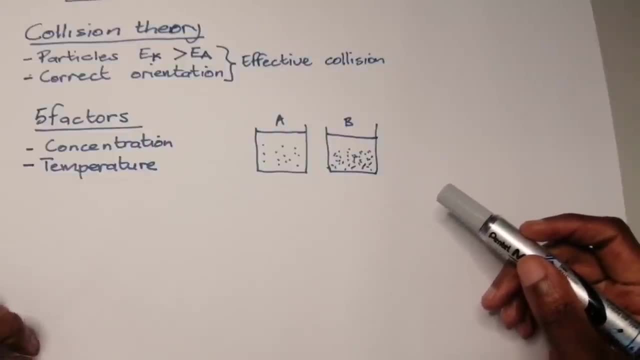 higher and, as a result, because there's more movement, then in that case there's more collisions per second and, as a result, a 24 minute slide than 50Rich light internets and they might increase or decrease the energy differently than 100 before, 20 apiece up or under the content. then after 5 years, 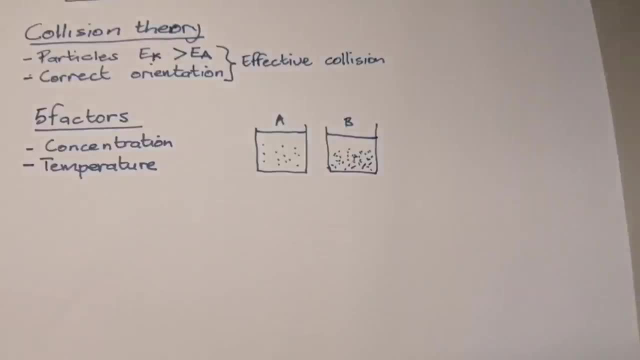 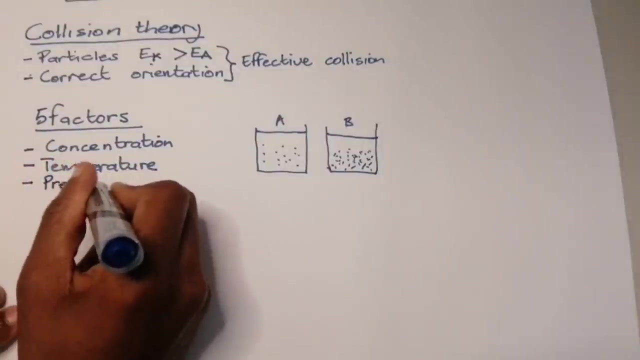 that would increase the rate of the reaction. I hope I'm summing it up quite nicely, right? and then the next one. we say that it is so. we said its concentration, its temperature. well, the third one is pressure. okay, now, in pressure, I want you to think about it like this: would this, would actually 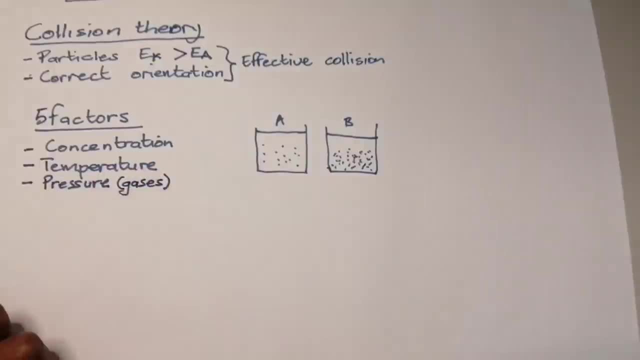 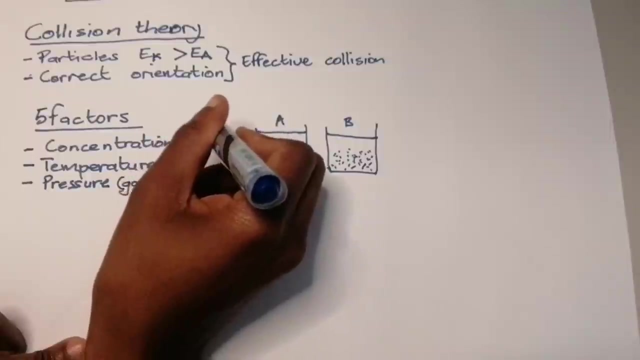 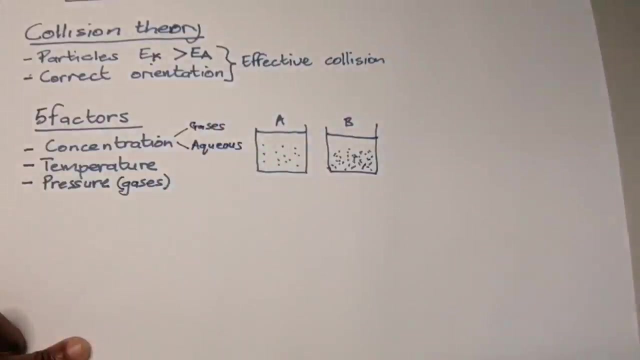 affect gases. okay, just remember that. and, by the way, can I just say this whilst I'm at it: when I talk about concentration, remember that concentration only is applicable when it comes to guesses and a cure solutions. a cure solutions, right? so in this case, once it's a solid, remember that you cannot define it in. 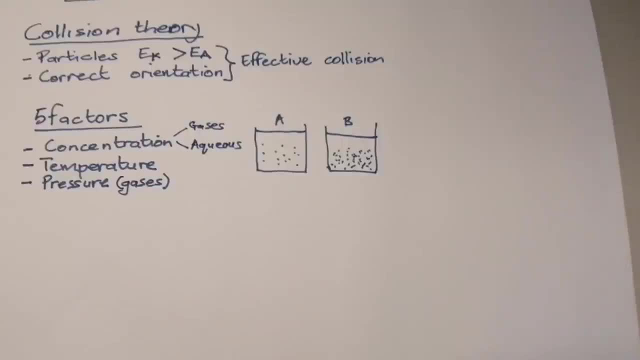 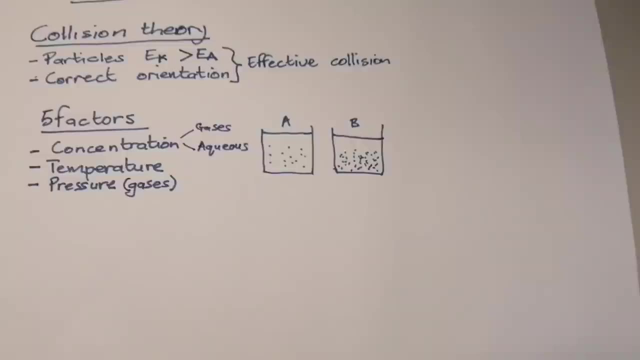 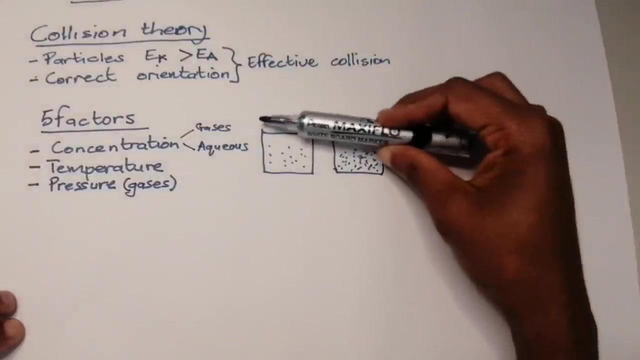 terms of concentration. I want to get into those details but, as I said, I don't want to bore you too much. I want to get into past exam questions as quickly as I possibly can, right? so in this case, when we talk about pressure, so when I increase the pressure, what am I doing? I'm actually decreasing. 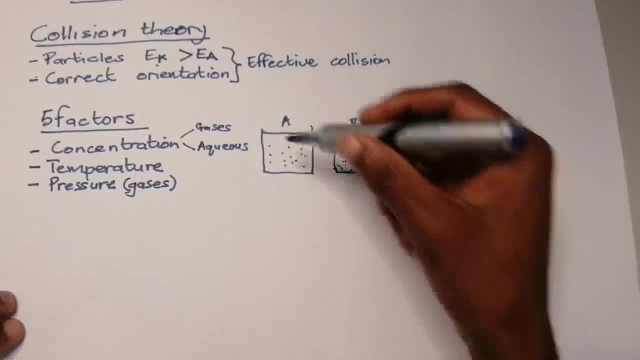 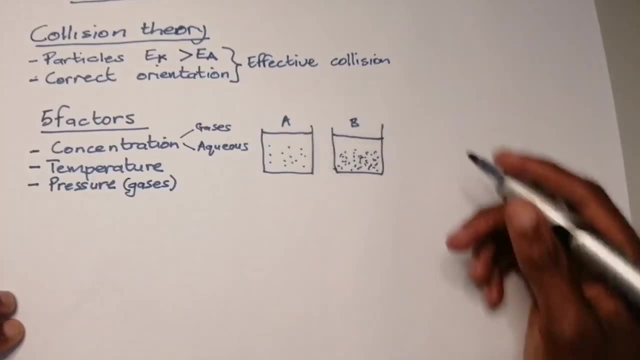 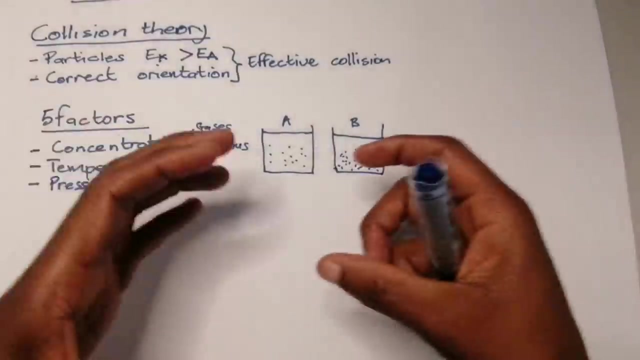 the space and say maybe this was my container. and now I increase the pressure. what am I doing? I am going to now decrease the space that is there. so what happens? the particles get closer together. and right and think about it now. the closer they are to each other, the same thing. 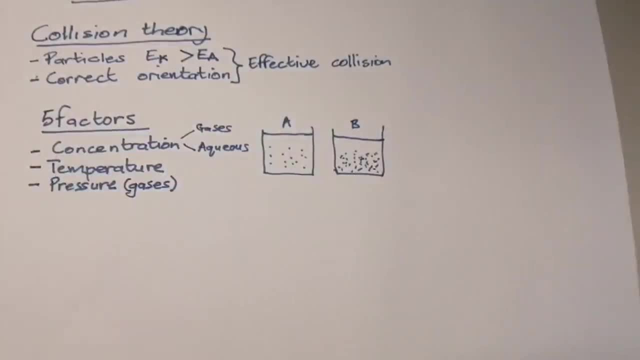 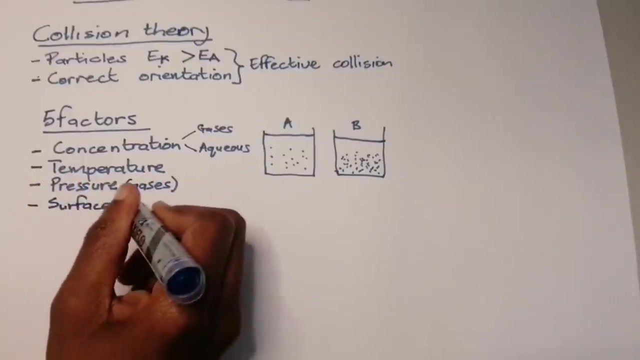 would happen when we had a higher concentration right. so the closer they are, the more frequent the number of collisions take place per second and, as a result, the rate of reaction would also increase. and then we also have surface area. okay, so surface area, or sometimes they talk about the state of division. 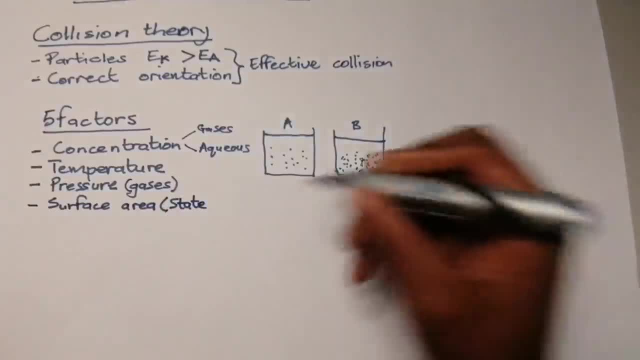 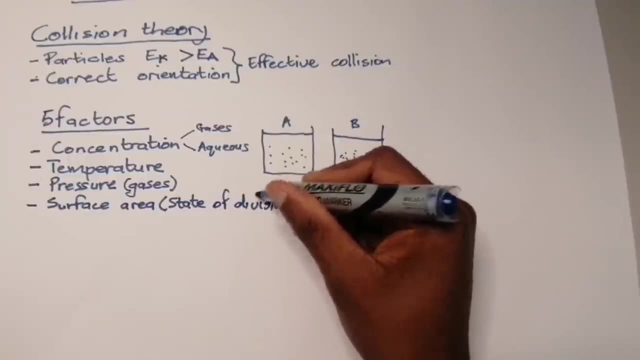 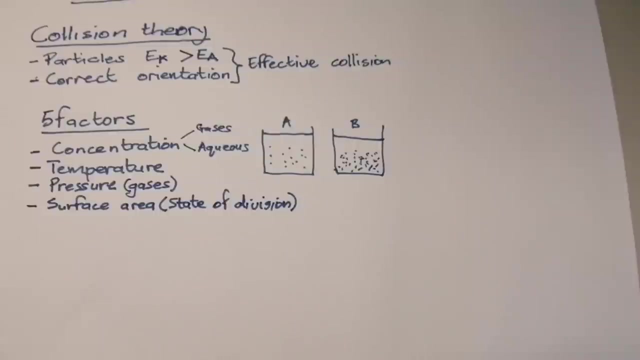 right, so, once we have reached the point where the particle radius of the just distance, okay, that would happen when we break something down into smaller pieces. right, so, when we have a very large about dollars 작업, in this case, when we would consider creating a usable 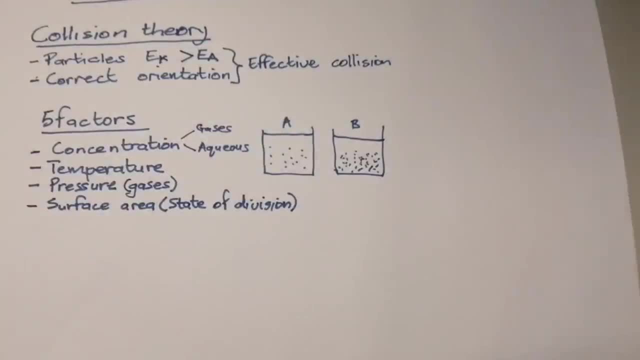 distribution. look, especially in the case of machines video last time. okay, technology, or what I call animation, where I can. in nature this is just a visualization, right? so whatever theечение of found in this part, I take something words, or imagine the uptake, andON Say it'll be, make a one line. that's kind of very easy. I do. I take the chance you're going to need a great. i've get it and in the final, 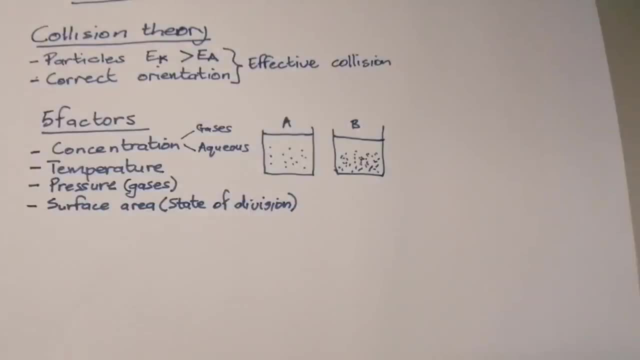 you know an amount of water and I wanted to dissolve. right, of course it would dissolve over time. but now think about it. what would happen if I were to crush it before I dissolve it? okay, right, you agree with me that it would actually dissolve faster when I've actually divided it more, right? so in this case, 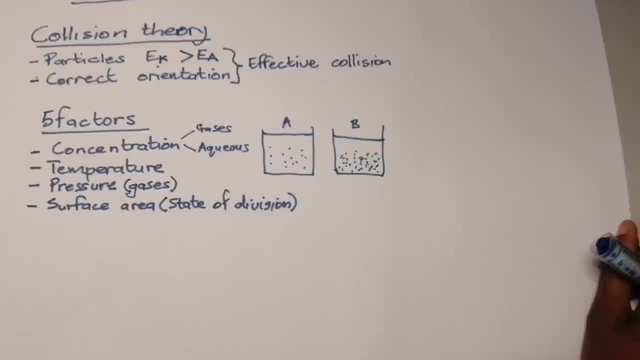 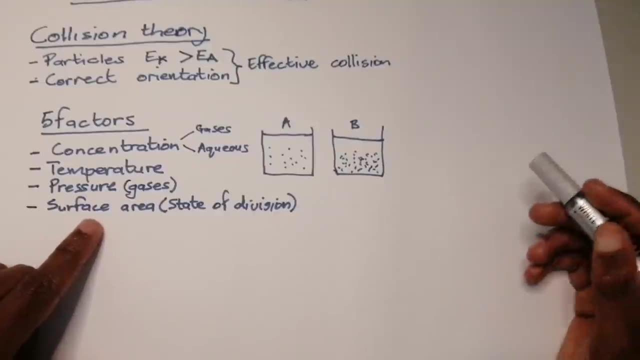 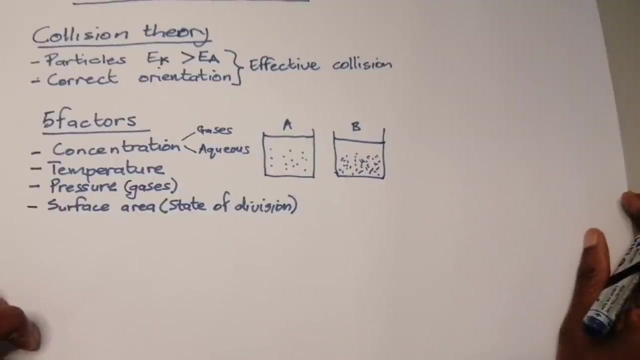 when you break something into smaller pieces. in this case, what it does is that it tends to increase the rate of reaction, right, even when we talk about surface area, this is when we are talking about usually. those would be reactions that you know, that are in a state of, that are in different states, right? so in 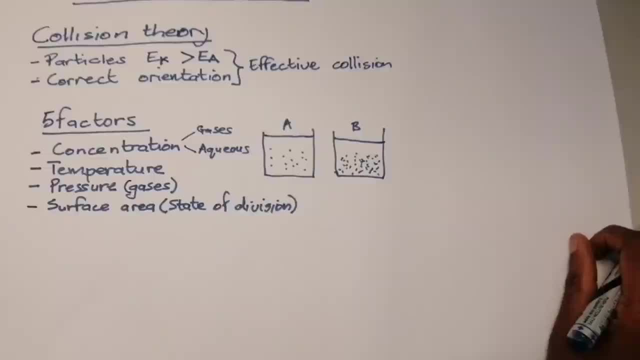 in this case, if I were to take something that is perhaps in a solid state- and you know, liquid- there's a word I'm looking for- it's just slipping my mind right- something that's in a liquid state, in a solid state, in this case, the one that is solid. if I can make it to spread it out a little bit, more, okay, it. 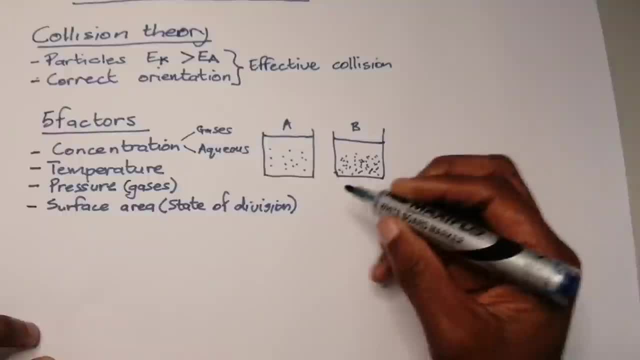 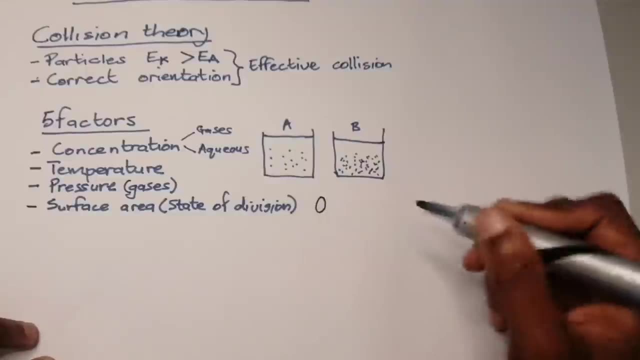 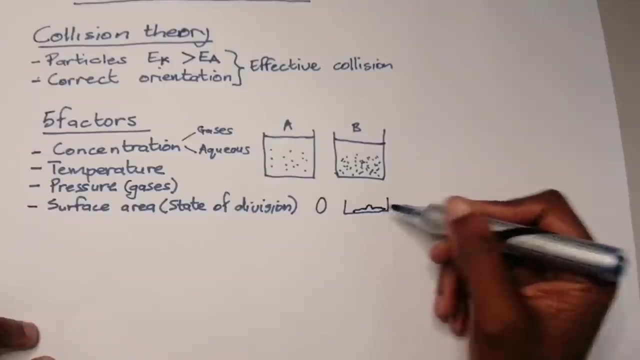 would increase the rate of reaction. in fact, I want you to just think about it normally when want to cook an egg. right, if I were to take an egg and I boil it in water, versus an egg that is fried, okay, I don't know how to draw an egg, so 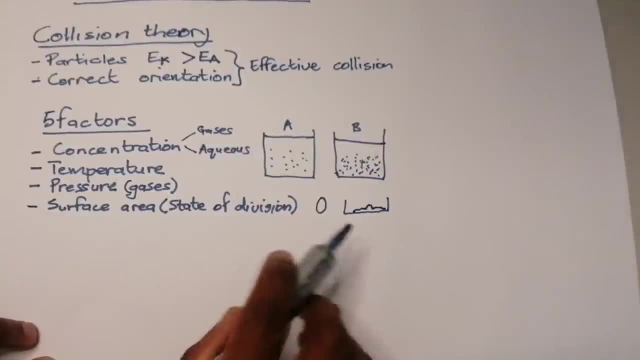 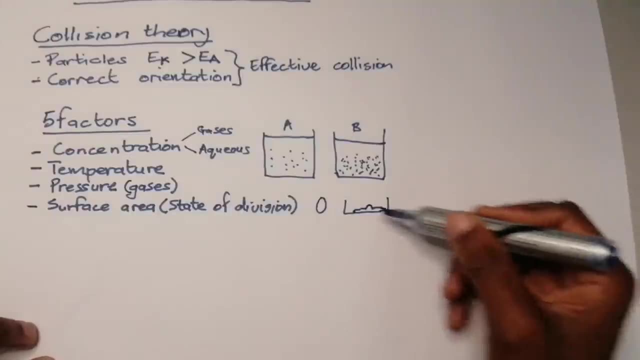 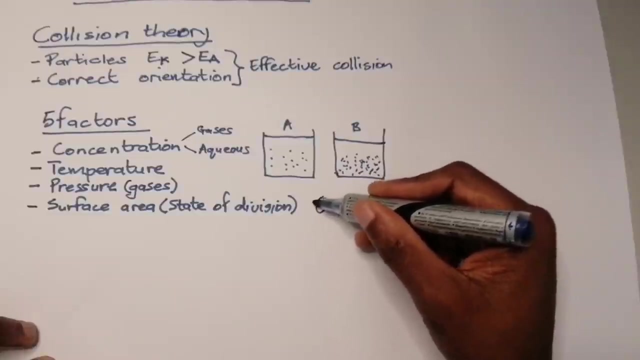 there's a egg away to fry it right. which one cooks faster? definitely it would be the one that is fried right, but why is that? because this one is actually more spread out, so heat tends to reach more of the egg quicker than this one, that is, that is boiled right, because heat can only be only on the 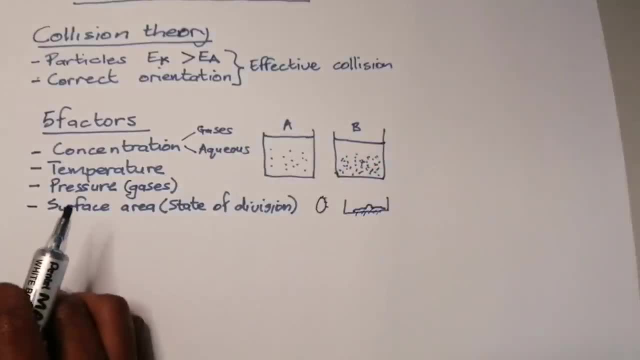 outer surface and it can go in, uh, gradually. so in this case we say that surface area does increase the rate of reaction. all right, okay. and then the last one, it's the addition of a suitable catalyst. okay, now, ladies and gents, we've got um two types of catalysts. okay, we've got what we. 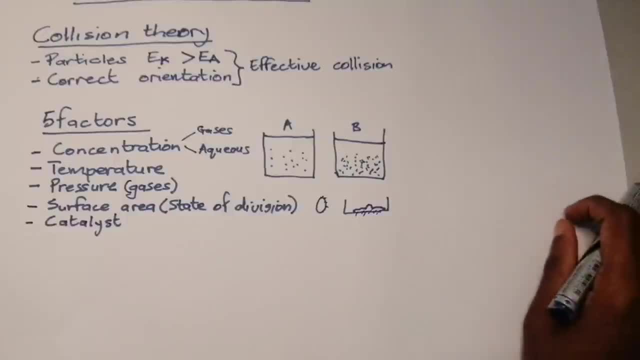 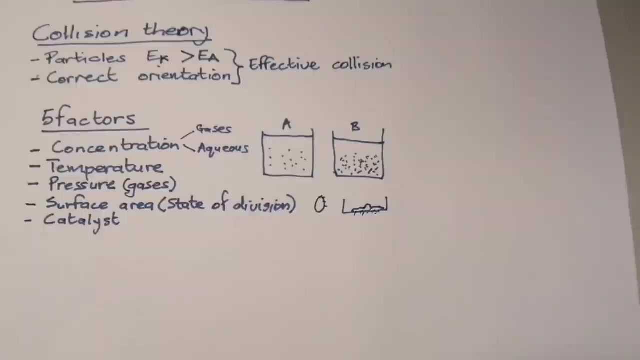 call positive catalysts, and these are catalysts that speed up the rate of a reaction. okay, um, so in this case, when you add that catalyst, uh, what is a catalyst? let's, let's start there. okay, so we say catalyst is a substance that speeds up the rate of the reaction without 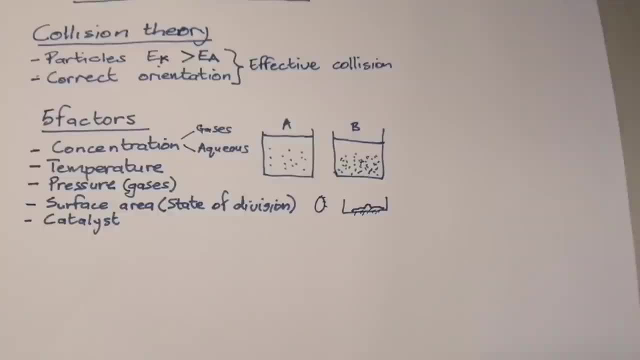 itself undergoing any permanent change. right, so, um, a catalyst can, can, speed up the rate of a reaction without necessarily participating, uh, in the reaction per se. okay, so it doesn't undergo any permanent change. okay, so it doesn't undergo any permanent change. okay, so it doesn't undergo. 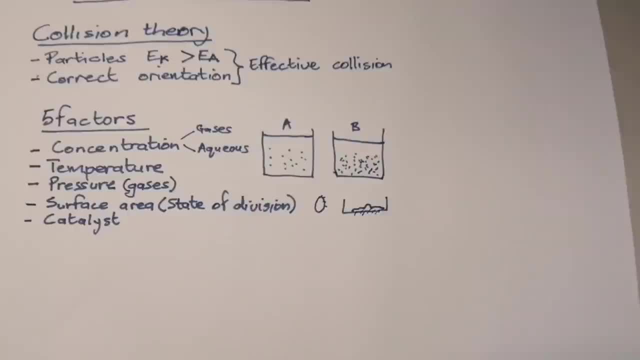 any permanent change, or it does not undergo any chemical change, for that matter, right? um, and then we've got another type of catalyst, which is a negative catalyst, which is, uh, called an inhibitor, right? so what that catalyst does is that it slows down the reaction. okay, and basically, how? 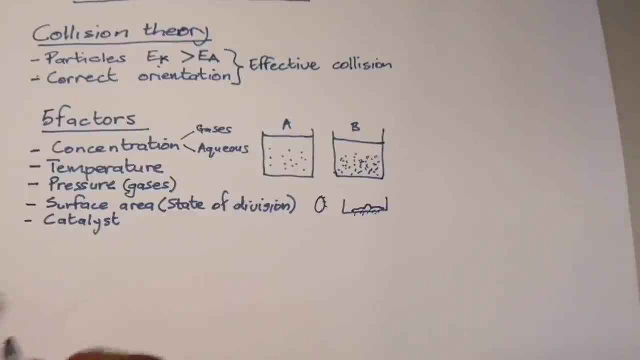 does a catalyst actually work? what it does is that a catalyst would lower the activation energy of a reaction. okay, now i want you to imagine this, okay, um, so if, if, if, we lower the energy that is required for the reaction to take place right now, all of a sudden, it means that 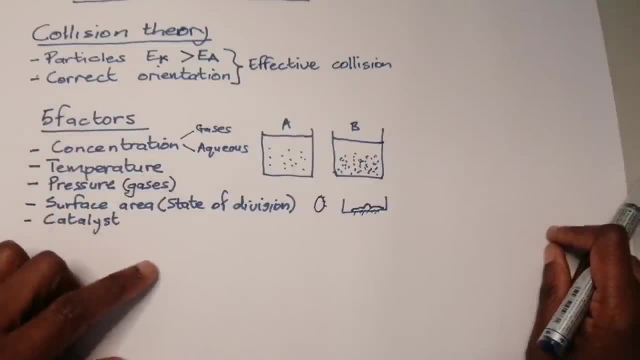 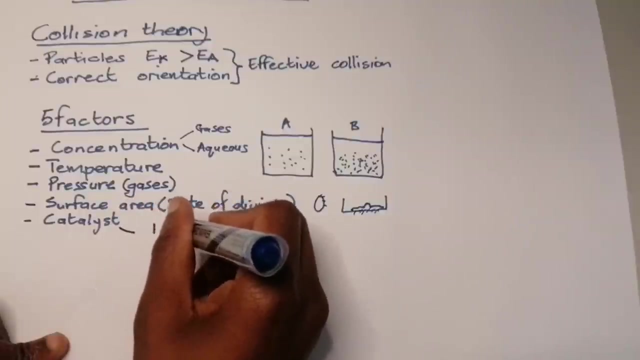 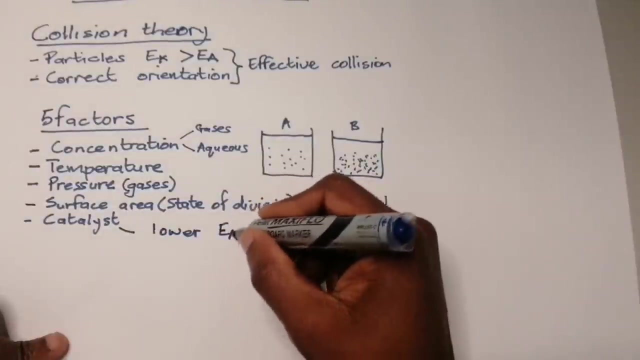 more particles now possess sufficient kinetic energy and therefore, uh, it means that more effective collisions would take place. okay, so what we're going to do is we're going to use this as our catalyst. right? so what a catalyst does is that it lowers the activation energy- i want you to remember that- right? or it decreases the kinetic energy, all right, so it lowers, sorry. 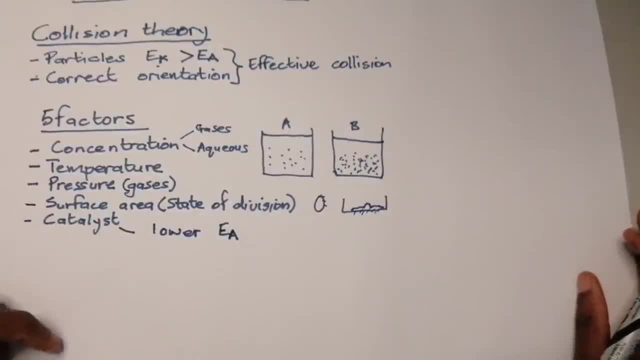 the activation energy. did i say kinetic? but it lowers the activation energy of a reaction, so it lowers the minimum energy required. so i want you to imagine this. if, let's say: um, they said we are a club right and people are going on trial, um, you know they are, they are going to um. 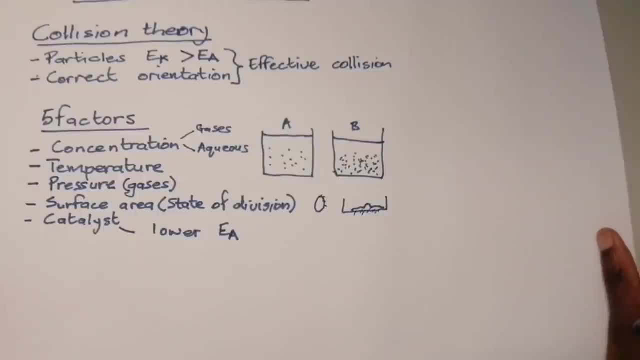 to try out for, you know, entry into the club. if they say, okay, um, it's a running club, let's say, for argument's sake, we want top runners. and they say, in order for you to qualify to be part of this club, you have to run a hundred meters in less than 11 seconds. okay, i'm just making an example, right. 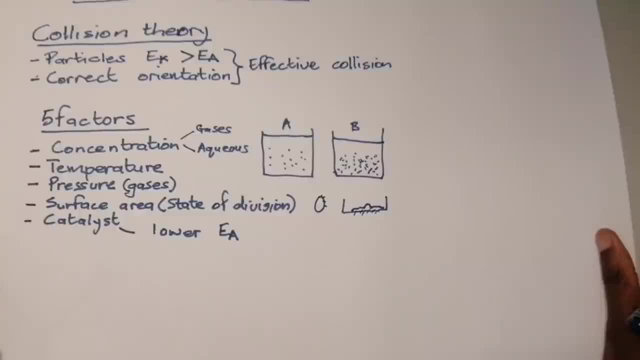 you agree with me that not too many people would make it right now. what if they now lower their minimum entry and they say, okay, in order for you to be accepted, you have to at least run 100 meters in 15 seconds? you agree with me that, because they've now 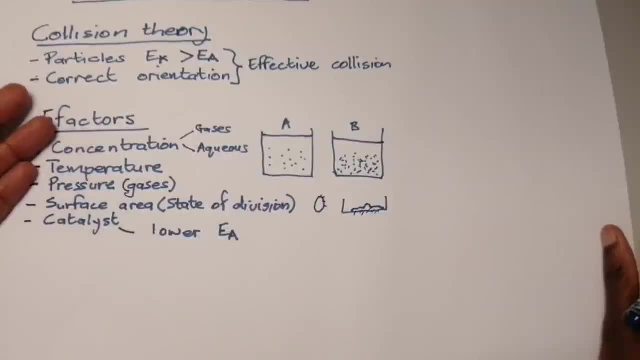 lowered the bar. it means more people can qualify, isn't it right? i want you to think of it this that way, about a catalyst: what it does is that it lowers the activation, the minimum energy required, so that now, more reactants now would possess sufficient kinetic energy, and so, as a result, it means that the number of effective collisions. 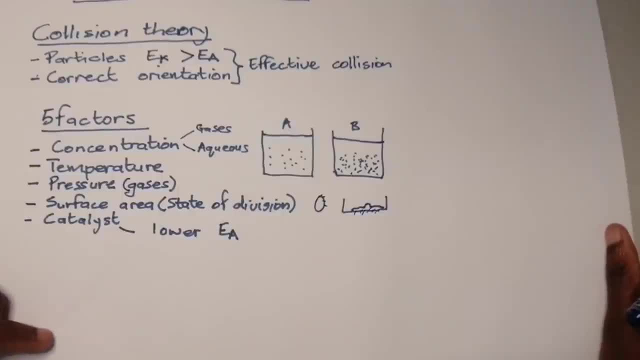 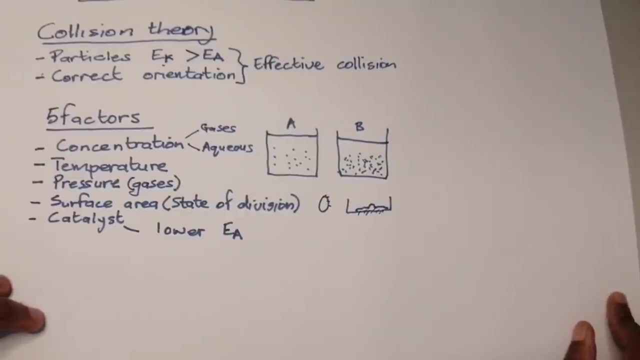 would take place. all right, uh, it would increase the number of effective collisions, and so that is how the rate of reaction would be increased. okay, right now, ladies and gents, what i quickly want to talk about are some of the graphs that are required um for rates of reactions, because 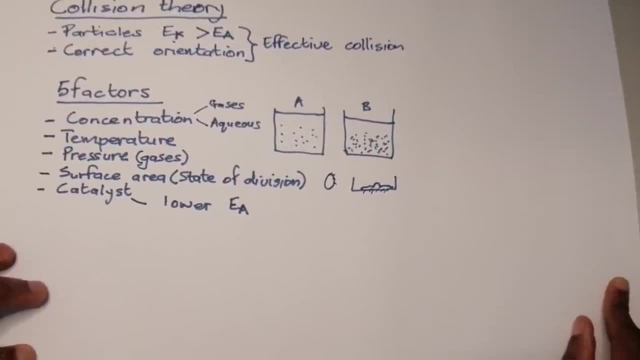 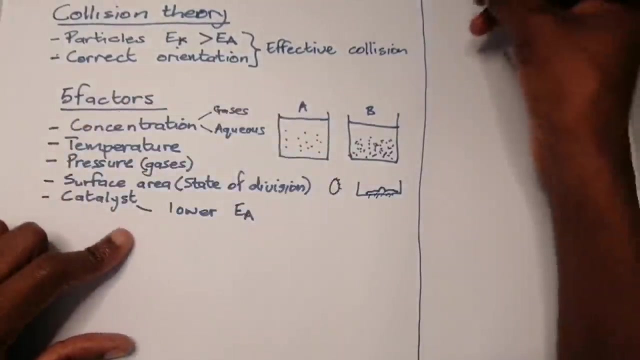 one thing or the other. you will always encounter those questions. okay, so now, um, we've got two types of reactions that take place, okay, um, all right, maybe let me just write it over this side here. okay, we've got reactions that are referred to as endothermic. okay, endothermic reactions. right now, in an endothermic reaction, i want you to just 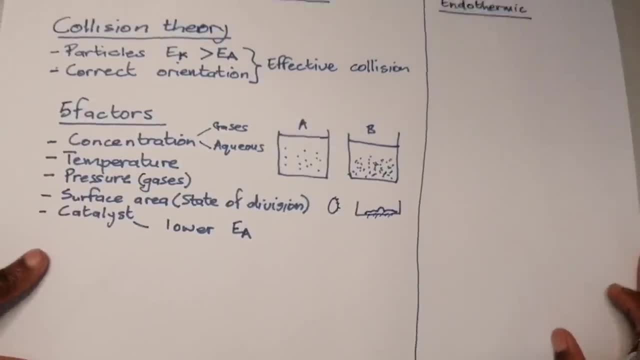 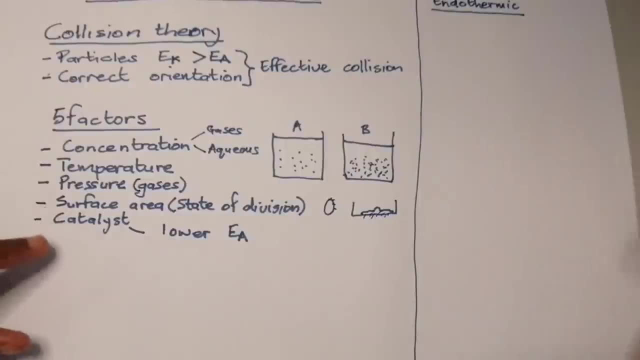 notice the type of graph that we are going to have: an endothermic reaction. sorry about that. okay, let me just bring this down a little bit. right? so in an endothermic reaction, what type of a graph am i expecting? right, so we've got a graph. 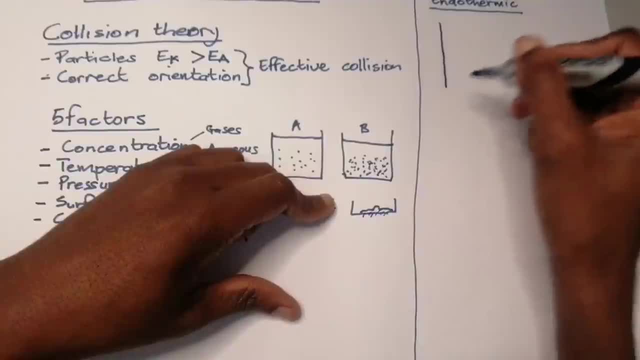 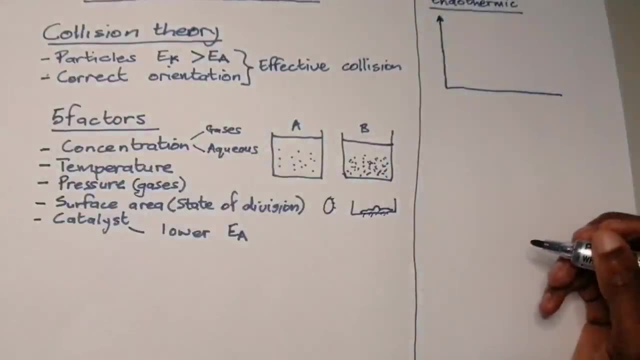 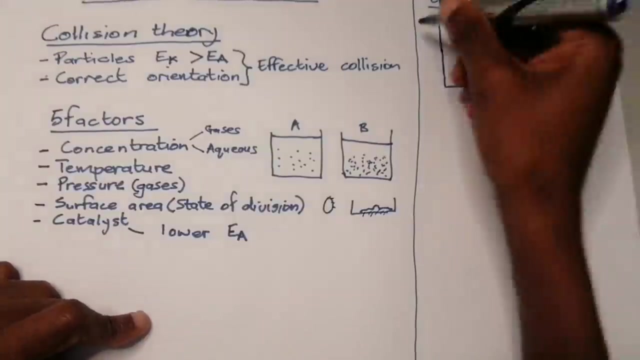 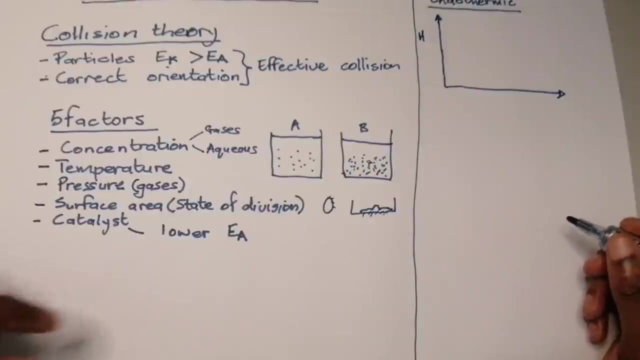 that shows us. now notice, it's going to show us the the heat of the reaction, or the enthalpy of a reaction. okay, against what we call reaction coordinates or the extent of the reaction. okay, so this would be the heat of the reaction, or the enthalpy or the energy of a reaction. okay, um. 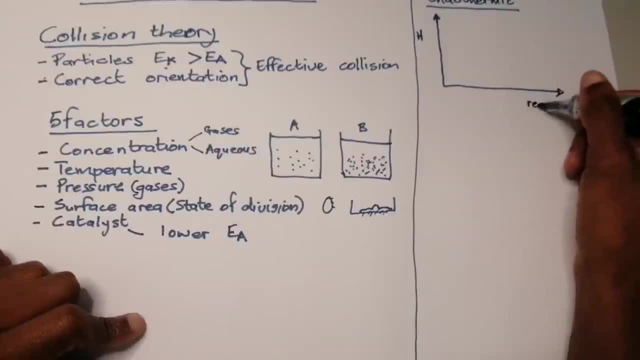 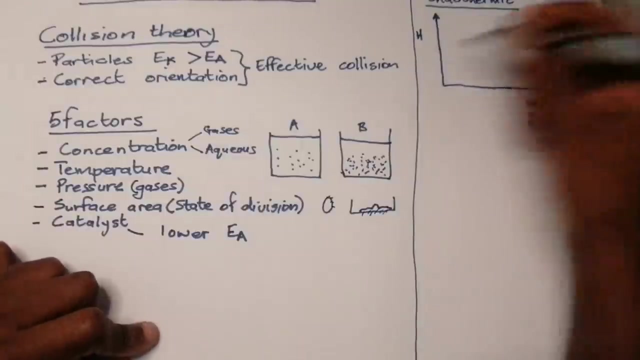 versus uh, in this case what you call the reaction coordinates. okay, um, reaction coordinates, so uh, sorry, uh, coordinate- ah goodness, i'm just making a holy mess here. coordinates, there we go right, so, um. so in this case we're saying for an endothermic reaction. how would you? 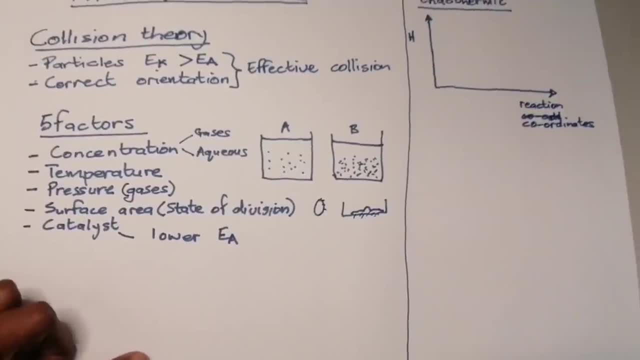 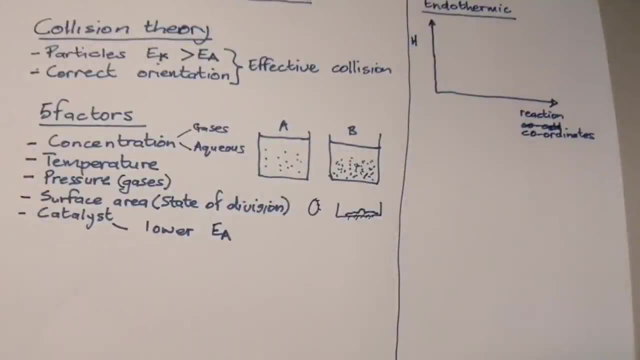 realize that now, as i said, ladies and gents, i really don't want us to go too much into the extent of the reaction for me. all i want you to do is just possess just that minimum that you need for now, and then, um, we'll go, we'll delve into more questions. 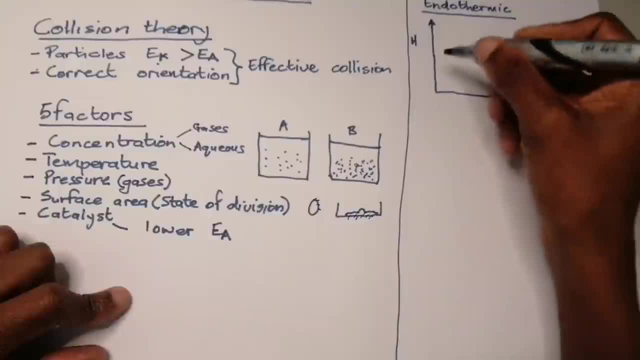 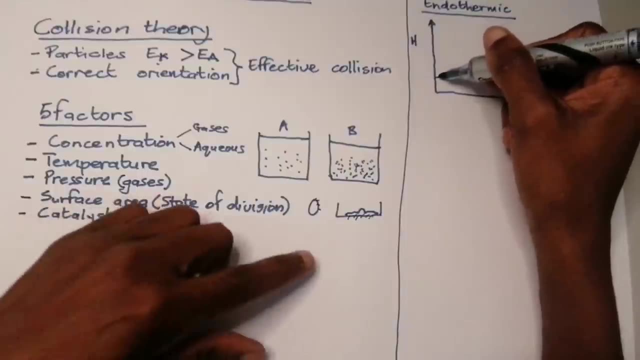 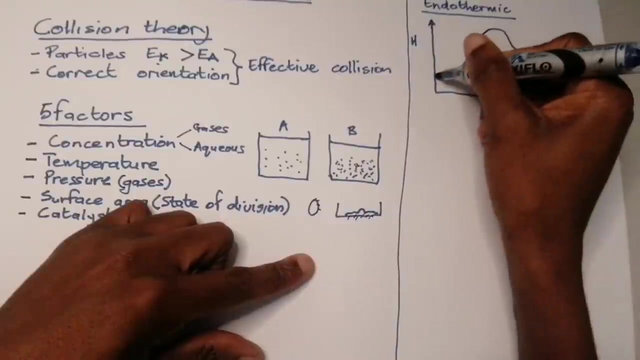 as we answer our past exam questions right. so, for an endothermic reaction, what happens there? and then we go, we're going to have, normally for an endothermic reaction, we're going to have a graph that looks like this: okay, so, whereas this is showing us, 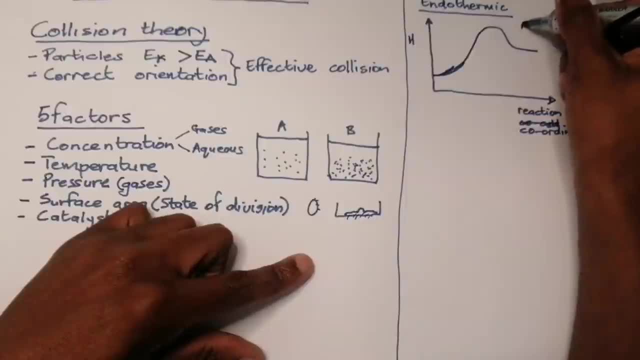 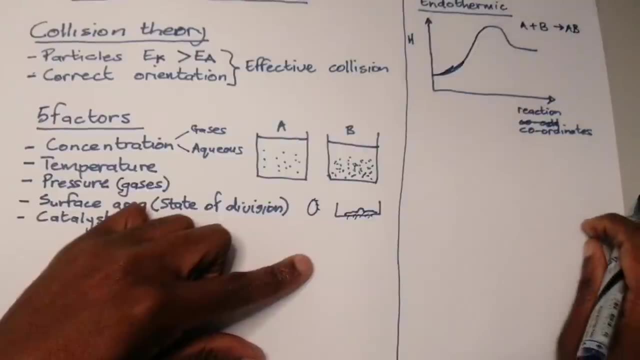 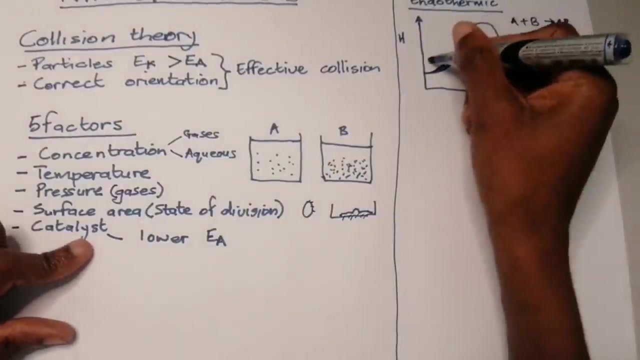 okay, let's say this is a reaction between two things, we're going to have a plus b giving us a b, right? so if this is a reaction between two things- a plus b giving us a b- this is the part where we've got a plus b as reactants. now you can tell the energy here. 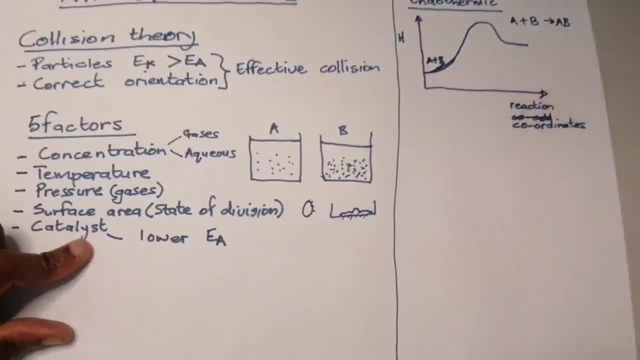 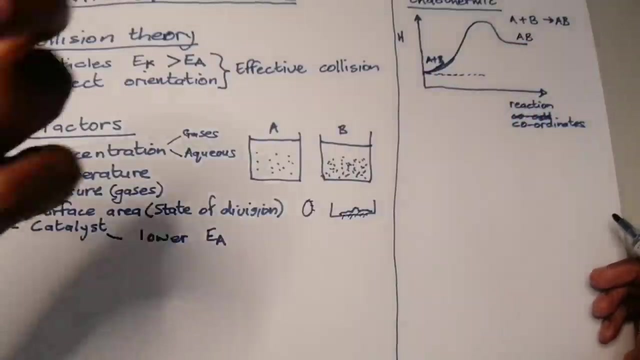 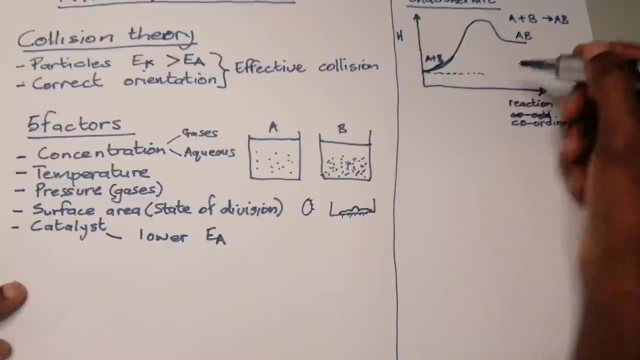 right, is lower than the energy there. so this is the portion where now we've formed products. okay, so in an endothermic reaction, it simply means that, um, we now, or rather the, the products- need to absorb energy in order to form products. okay, so the reactants need to absorb energy in order to 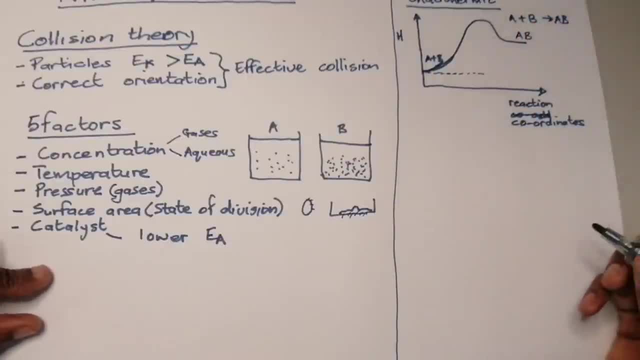 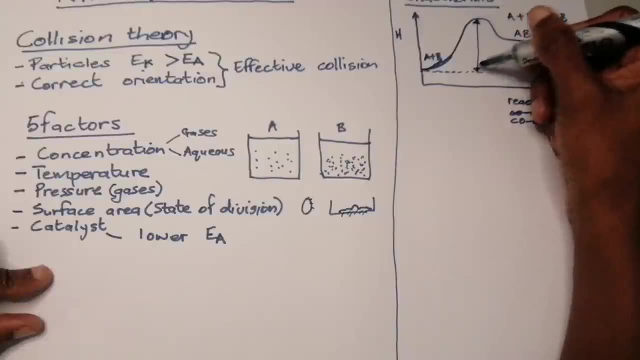 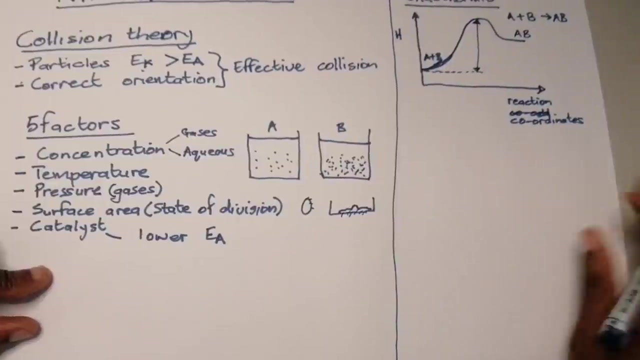 form products. now, several things that i want you to note in this graph. the first thing that i want you to note is that this energy here, okay, so, between the reactants and what we call the activated complex, okay, so, this is the temporary state and it's it's an. 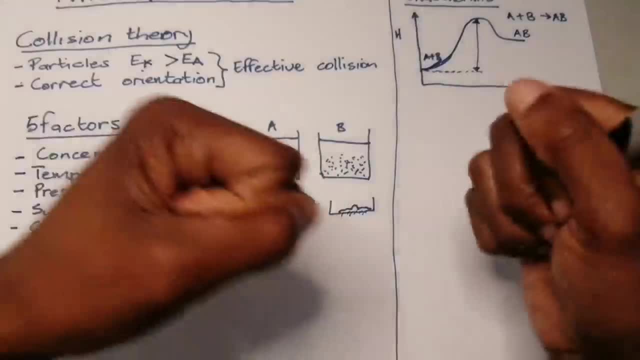 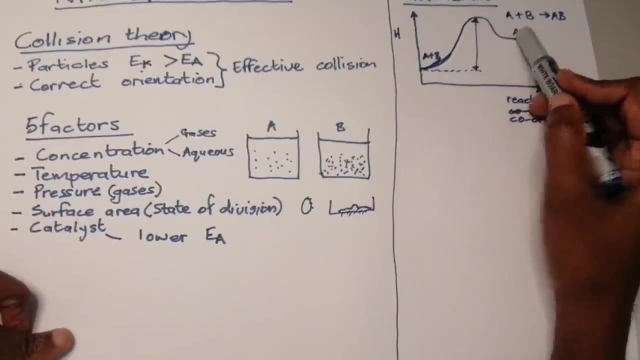 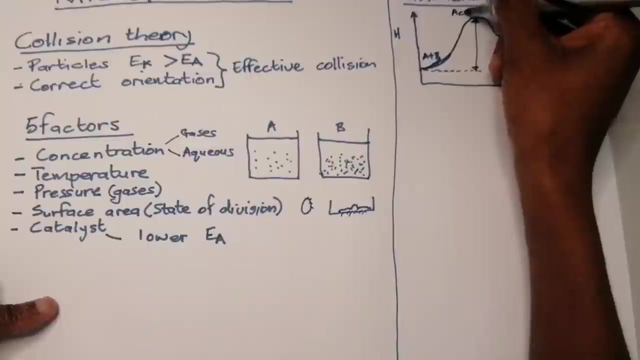 unstable state. so this is when you know, after they are colliding, they have high energy and they are temporarily unstable just before they form products, right? so at this state here. so we call it the activated complex. okay, so this is the activated activated complex, right? this is the state there. 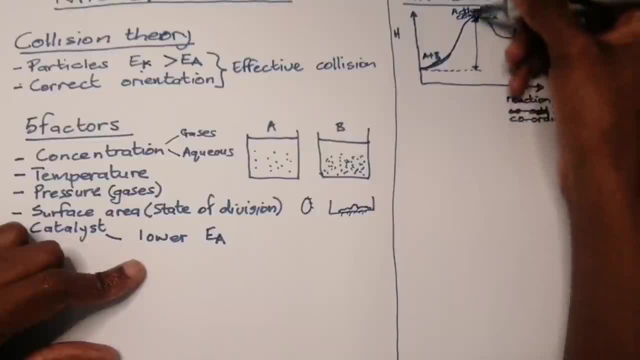 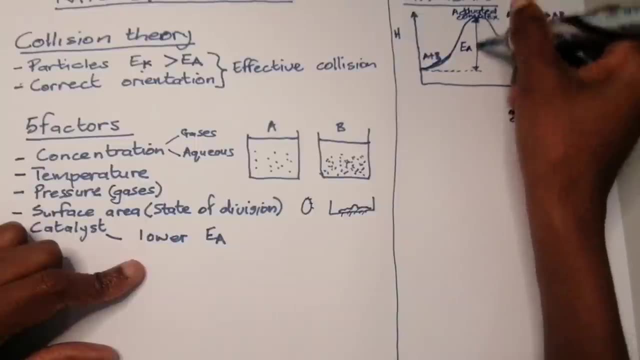 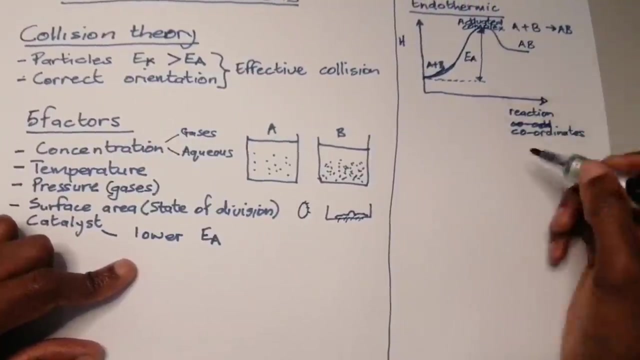 so we're saying, in order to get there, we need to put in a high amount of energy. so this is the activation energy for the forward reaction. can you see, for an endothermic reaction it would be a high amount of energy that's required, isn't it so in this case? um, so this is the activation energy for. 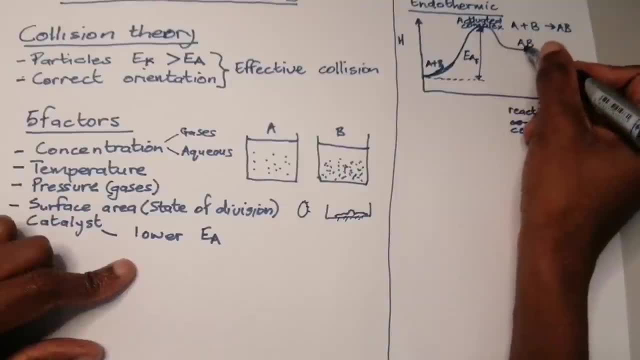 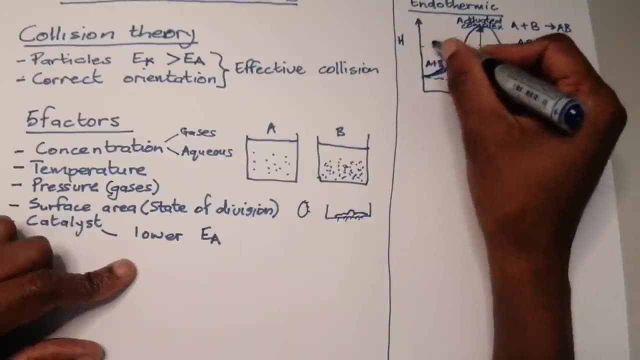 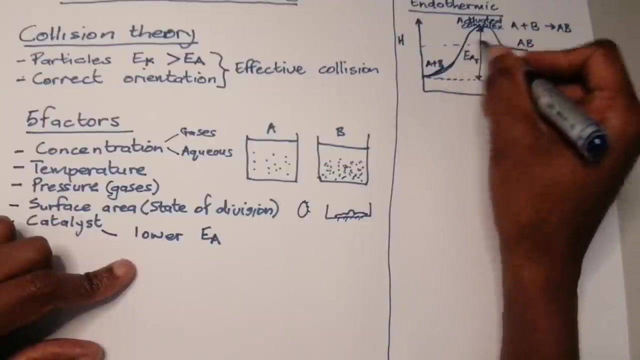 the forward reaction. and then you look at this. so we say, okay, this is the energy of the products. okay, i'm getting somewhere with this, right. so this is the energy of the products. now you can see, for an endothermic reaction, the energy of the products would be higher than that of the reactants, isn't? 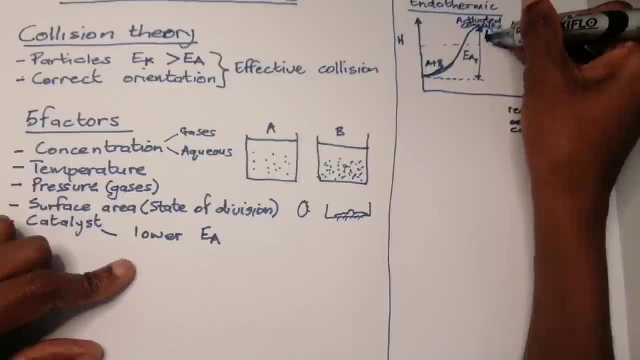 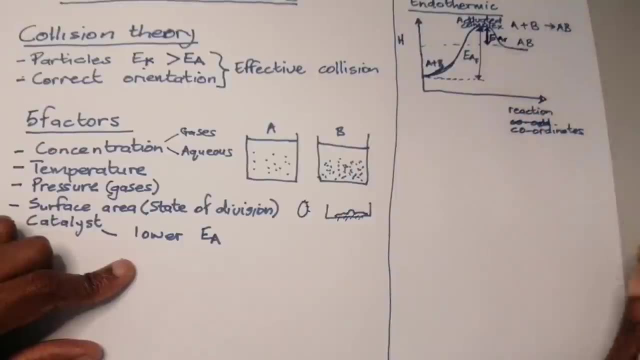 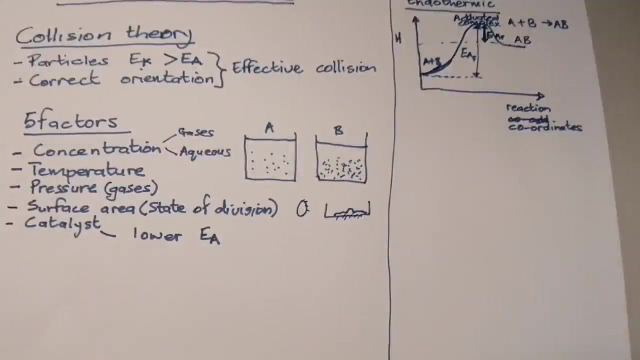 it. so, um, where do i get the activation energy for the reverse reaction? so this is e a r okay, so i'm just going to designate it e a r there. sorry about the mess that i'm making right? so, uh, in this case, we're simply saying that is going to be the activation energy for the reverse. 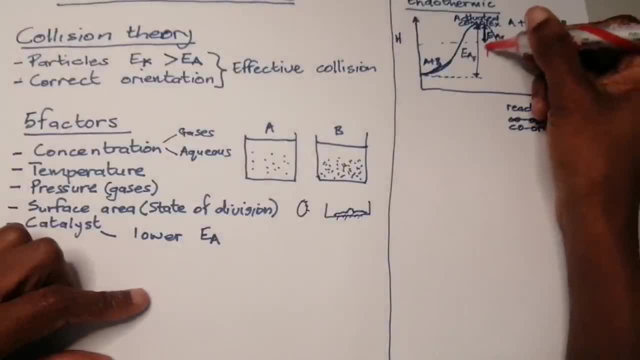 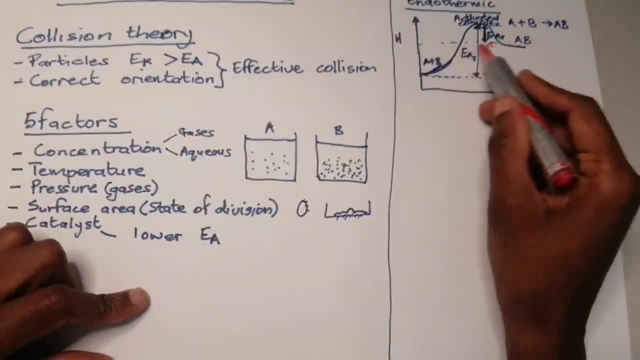 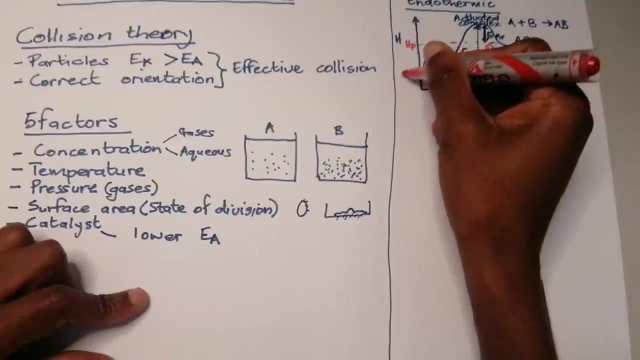 reaction. now, ladies and gents, i want you to please note: why am i showing you all of this, right? so now we get to this part here where it's the energy of the products, right? so this is the energy of the products, this is the energy of the reactants. uh sorry, this is the energy of the reactants, right so? 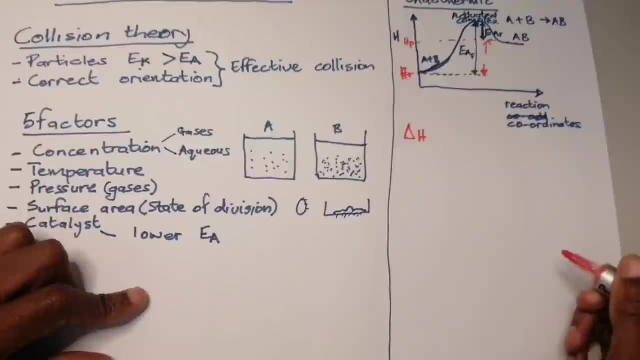 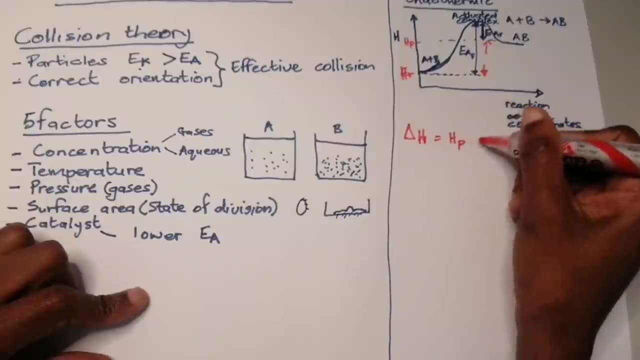 then we start defining what we call the change in enthalpy, delta h. right, so we say change in enthalpy is simply going to be the energy of the products minus the energy of the reactants. right? so i want you to please notice here we've got a higher value. whatever that value would be, right? um, let me just 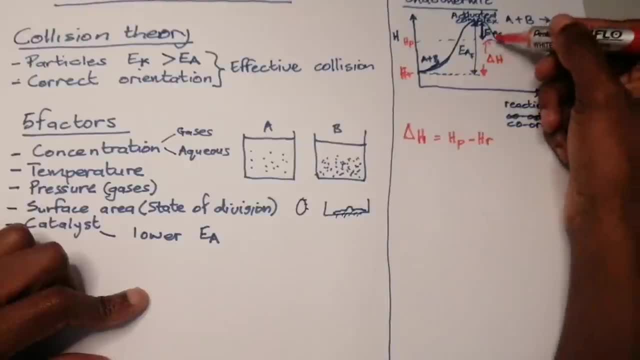 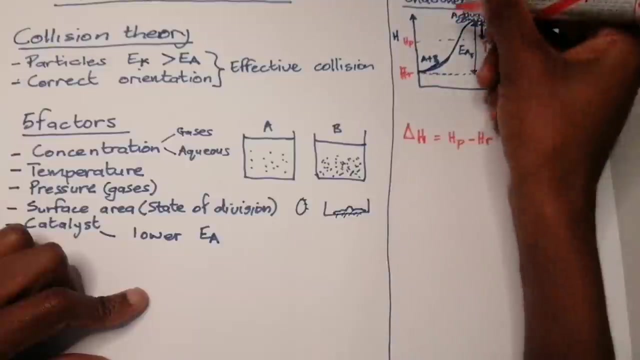 show you that this is delta h there. so, whatever this energy would be, you agree with me, is higher than it, is higher than that, uh, that energy there. so, um, this value minus that value, it would always give you a positive result. okay, so for an endothermic reaction, you've got delta h. 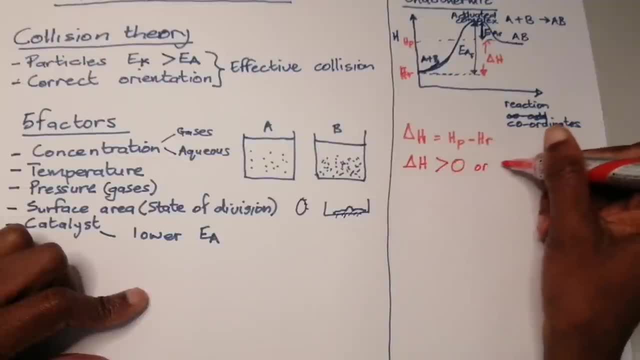 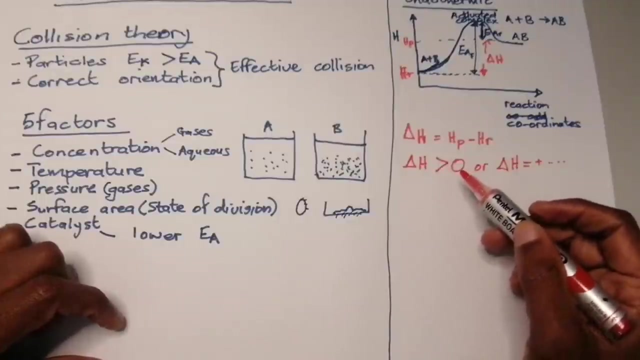 that is greater than zero. or you can just simply say delta h is positive. so they may give you: delta h is equals to positive, whatever the value may be right. so immediately, when you see that delta h is greater than zero, what it's simply telling you is that the energy, or rather the reaction, absorbs. 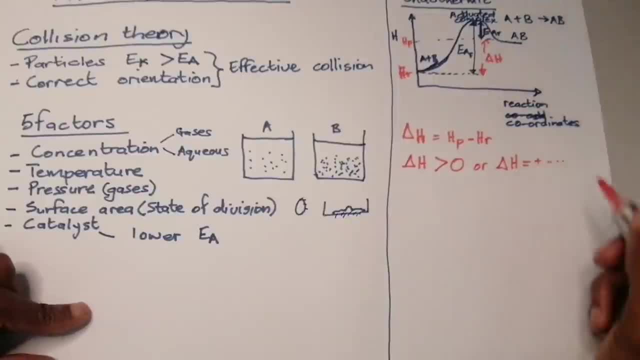 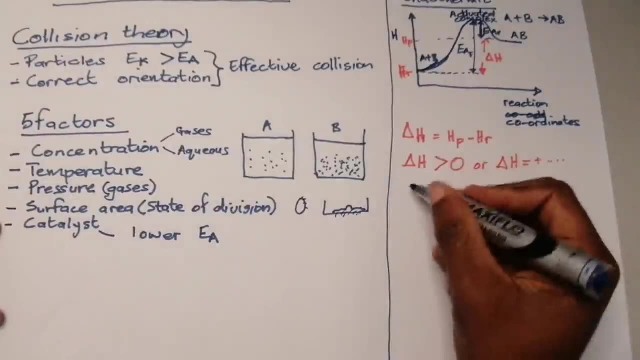 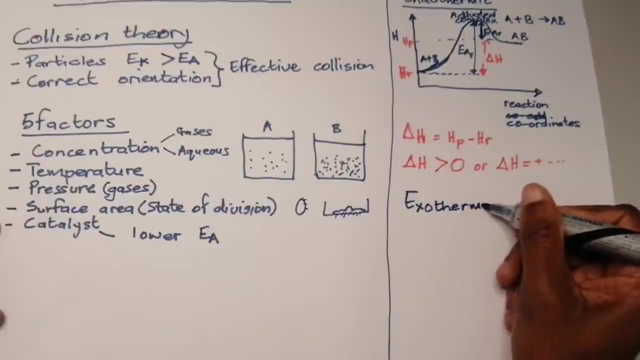 the reactants rather absorb energy in order to form products. okay, right. so, um, then we've got what we call an exothermic reaction. okay, i'm just going to write it down there. you can tell i'm trying to rush as much as possible, right? as i said, i don't want you getting bored before we get to the 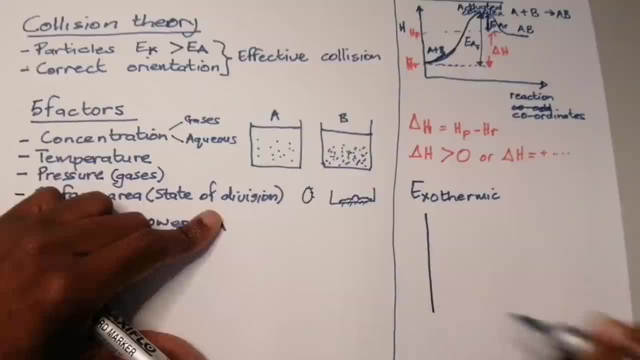 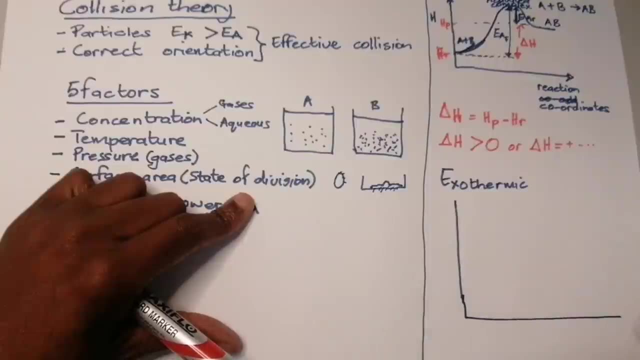 crux of it. okay, i'm just going to open up a little bit more space here, okay, right? so, uh, for this reaction, what we have is that for an exothermic reaction you would have something like this: okay, so let's say we've got another reaction, a plus b giving us. 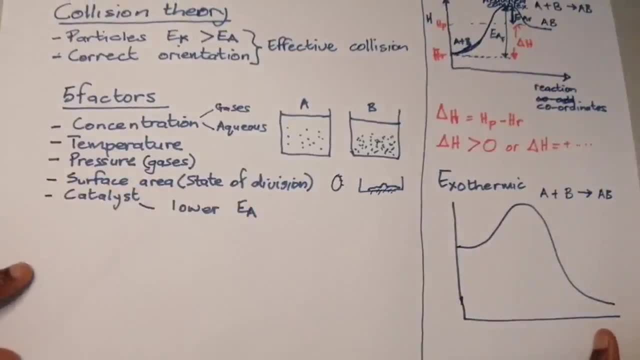 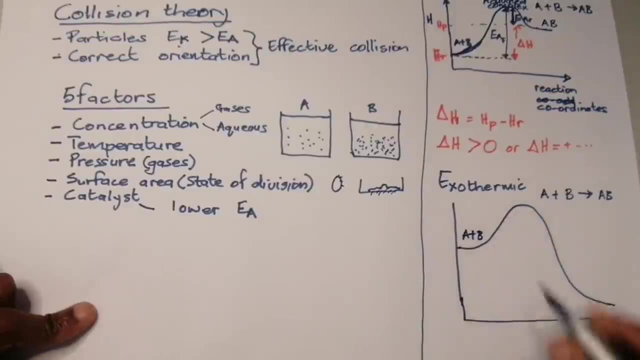 a, b, okay. so for an exothermic reaction- i want you to please note, this is where we've got a plus b, so this is going to be a reaction, a reactance there, all right, and then look at this: the activation energy that you require, okay, is actually less than when you compare it. let's say: 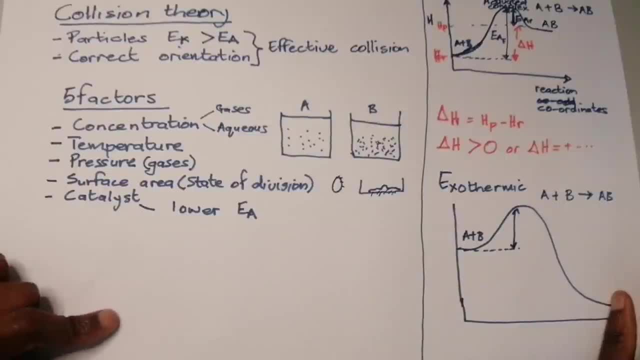 with a um, with an endothermic reaction. so this is the activation energy for the forward reaction, right? and then this is when you've formulated react products. and then what do you notice there, all of a sudden? um, this is the activation energy that you require in order to form um, or rather, 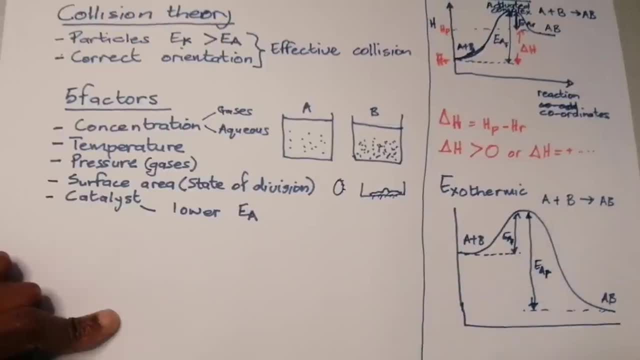 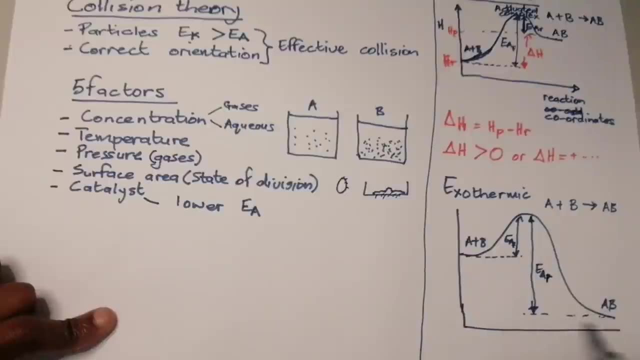 this is the activation energy of the of the reactants. okay, of the reverse reaction rather. so in this case, look at this: the products have got a less energy than the reactants. okay, so what we are simply saying in this case we're simply saying: in an exothermic reaction, you find that there is a net loss. 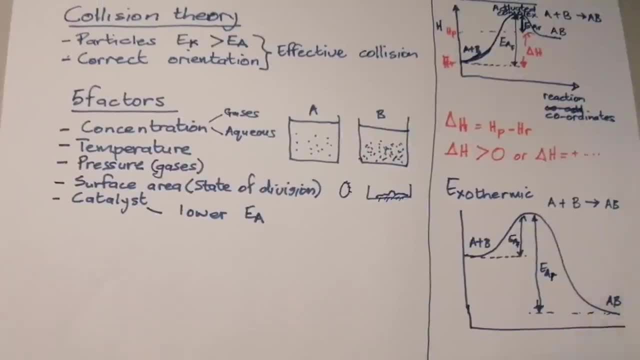 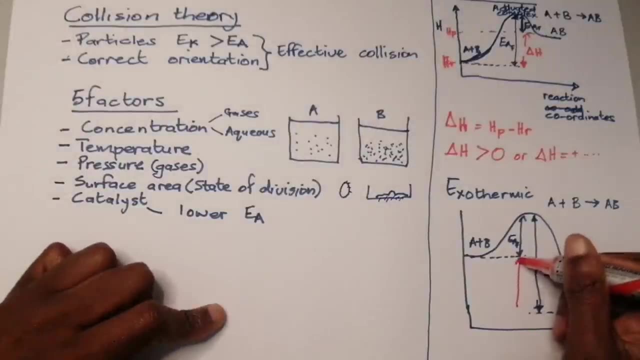 in the amount of energy in the reaction. okay, so as a result, what do we notice? we notice that, again, if we calculate that delta h value the energy of the product minus the energy of the reactants, so that's delta h, that's the change in enthalpy. right? so we find that if 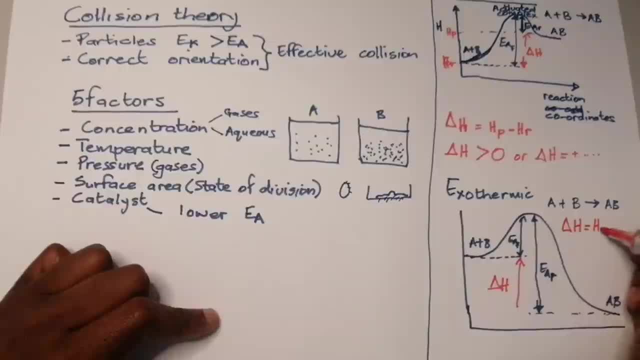 we find delta h. okay, it will be the energy of the products again, minus the energy of the reactants. okay, so what do you notice? products have got less energy. so it's a lesser amount minus a greater amount. so, yes, that sets us up now to get a negative result. so 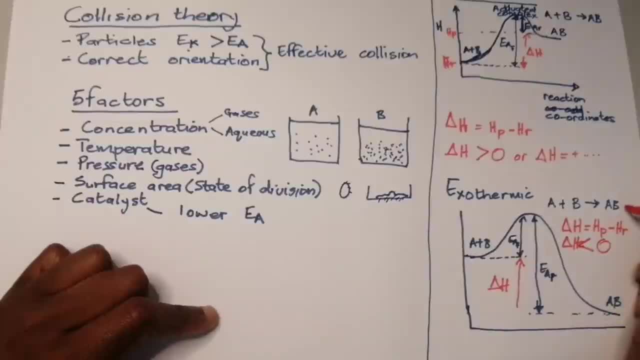 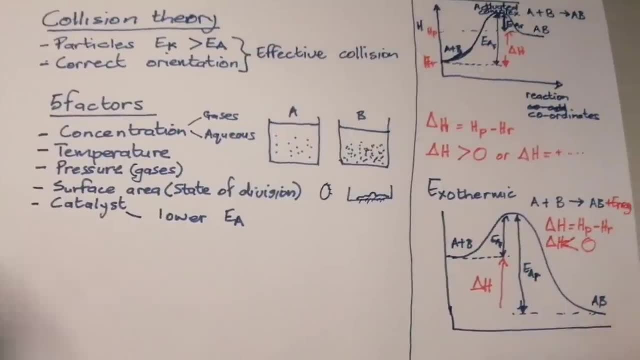 that is why we'll get delta h less than zero. so it means that what you'll find in this um, in this re, uh, in this reaction, so when it's a it you, you find that energy is released. so when it's an exothermic reaction, say maybe um, if you were conducting this reaction, uh, you know. 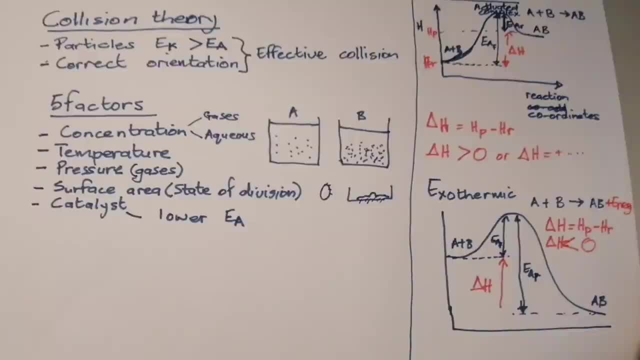 one of the examples is that of a- um, you know, combustion when, when, when, when you start a car, right? so, uh, after a while you'd feel that the engine of the car gets warmer, isn't it? but why is that? because when the octane in the car, all right, reacts with the oxygen, right it forms carbon. 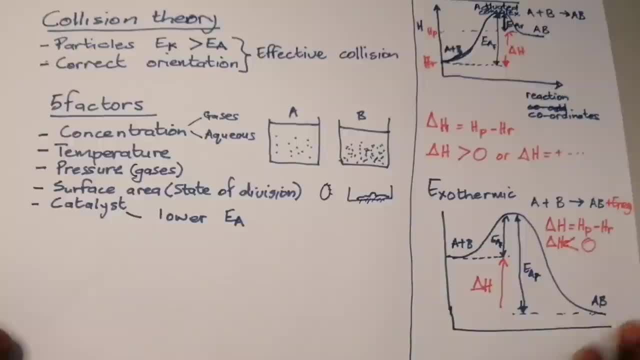 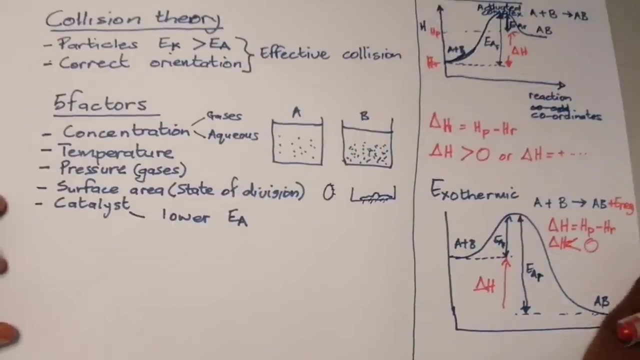 dioxide, it forms water, but it also releases energy. all right, so that is why you find that the engine ends up, uh, being warmer, of course, besides all the other factors, mechanical factors which i won't talk today. So the net result of that reaction releases energy, and so that is why it tends to get warmer. 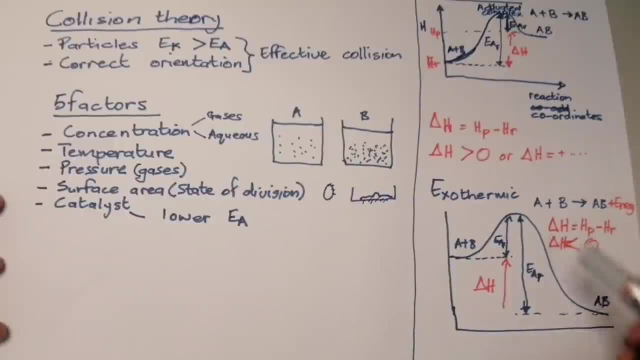 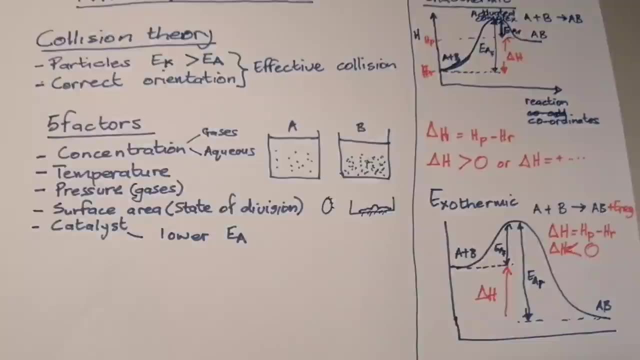 It's energy that is released together with the products. On the other hand, for an exothermic reaction, it's energy that is absorbed. So you'd find that when this reaction takes place, you know the reaction as it takes place, the container or the vessel in which you are. 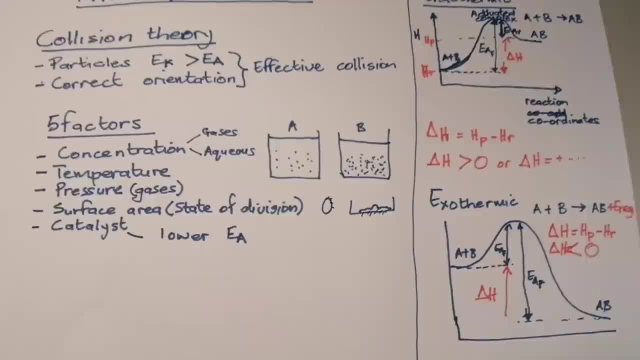 conducting the reaction in gets colder. So why is it getting colder? Because it's actually absorbing energy from the environment. okay, So, as a result, we know that it is actually an endothermic reaction. okay, So those are the factors that affect. 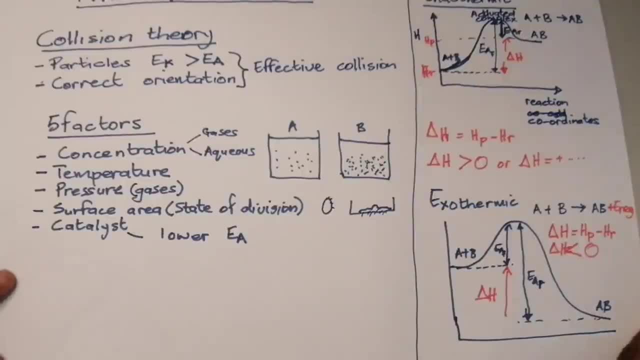 the reaction. you know the rate of a chemical reaction. Now, just one thing that I want you to notice, ladies and gents. So what happens in these reactions when we now add a catalyst? You remember what we said a catalyst does. We said it lowers the activation energy, right? So in this, 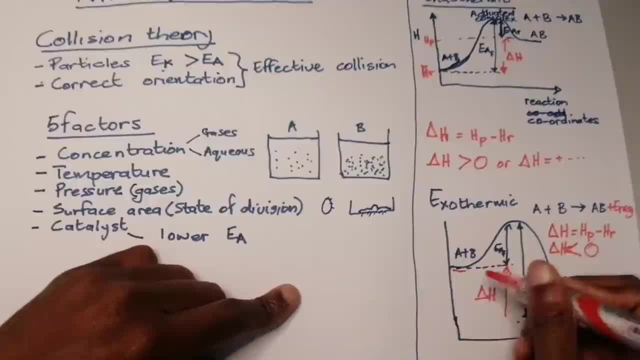 case when I add a catalyst, I want you to note, we'll still get the same graph, but you'd notice that the actual peak, the activation complex, takes place at a lower peak. Now I want you to note this red graph is a graph that shows us when we've added a catalyst. So when I add a catalyst, 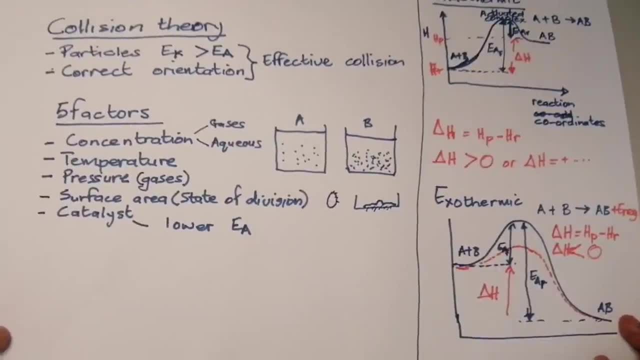 by the way, I'm going to say use catalyst generically, but when I say catalyst, I mean a positive catalyst in this case. okay, Obviously a negative catalyst would do the opposite. but all right, let's not focus on that much. 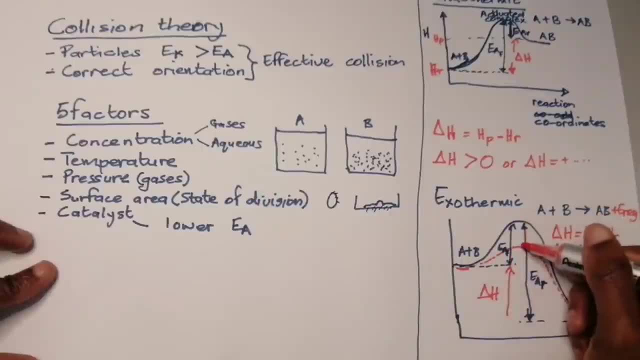 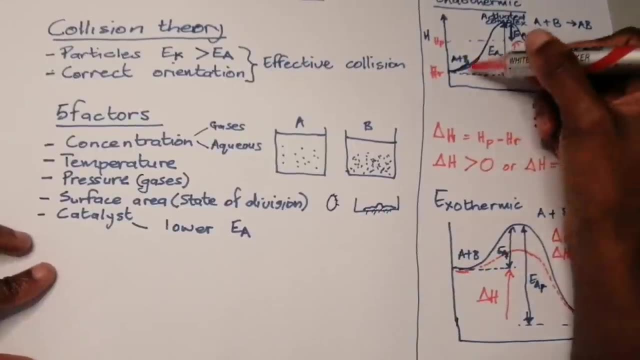 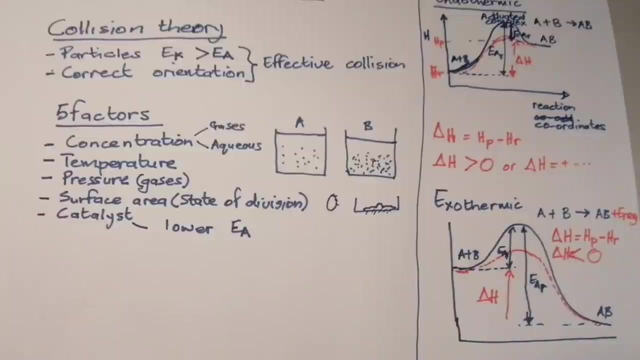 So when I add a catalyst, it's going to lower that peak there, so that the activation energy now is much lower than what it was. The same thing happens even for the endothermic reaction. right, When I add a catalyst it lowers that activation energy. okay, so that that peak. 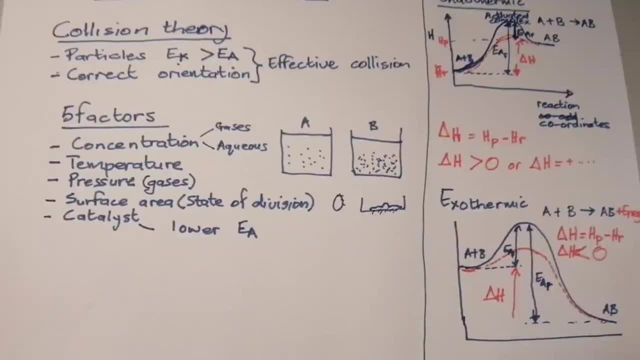 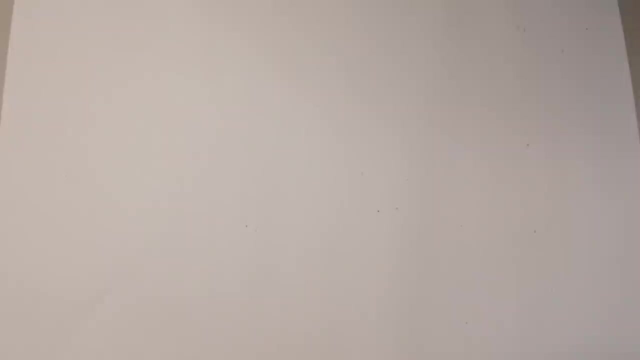 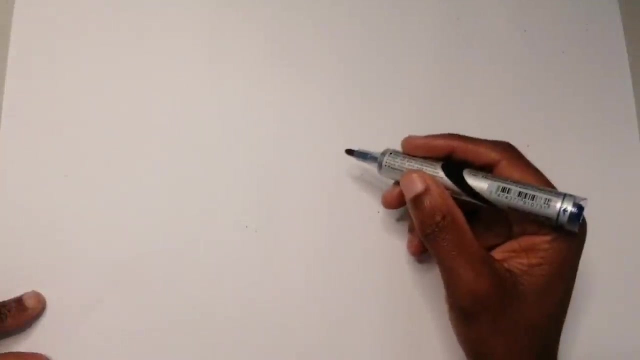 is much less okay, Right, so in terms of the theory, okay, I still want us to continue. all right, Now let's move on to something else. So we have what we call the Maxwell-Boltzmann distribution, right? So just to explain that quickly, ladies and gents, so this is a graph. 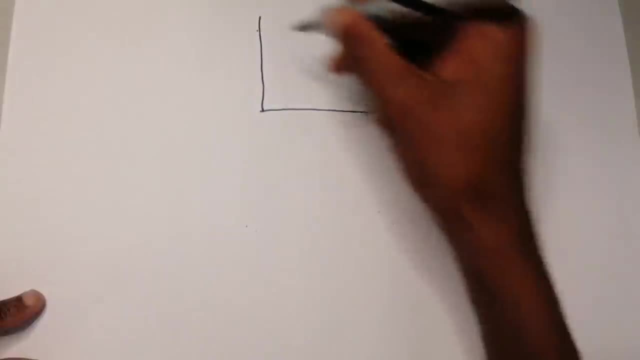 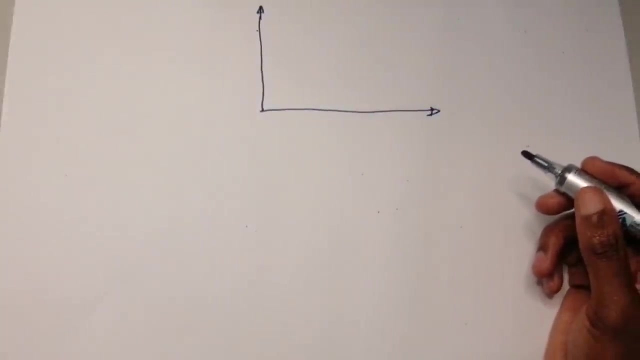 that shows us. okay, let me just try and draw that graph quickly. So this is the graph that shows us the. in a sense you want to imagine. you know the number of particles, So imagine in a reaction, you know so many collisions are. 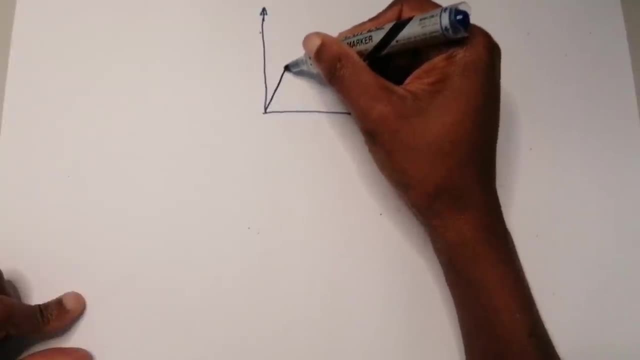 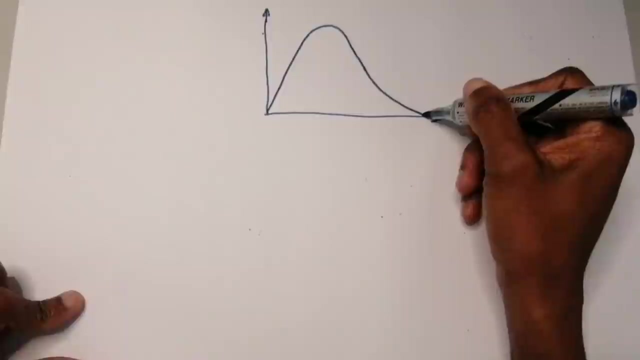 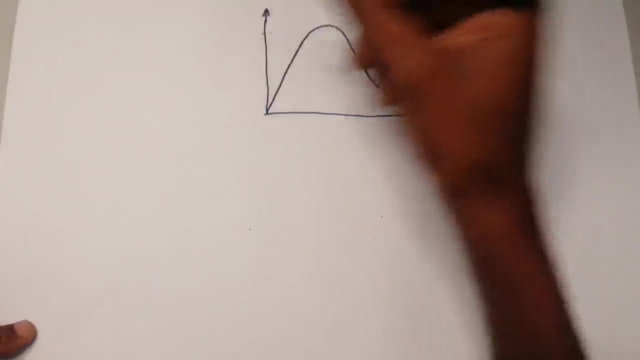 taking place. So it shows us the number of particles that are colliding, in a sense, okay, against the kinetic energy of the molecules. Now just something I want to. okay, so this is the number of particles. So number of particles. 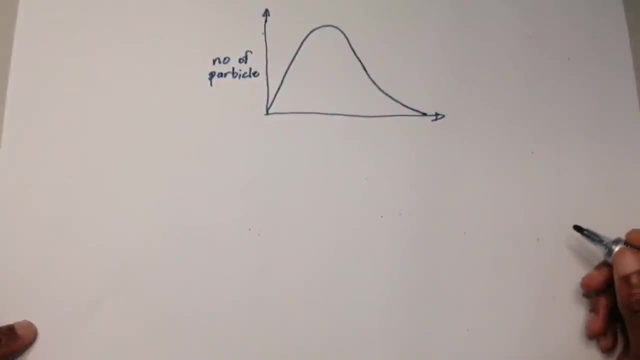 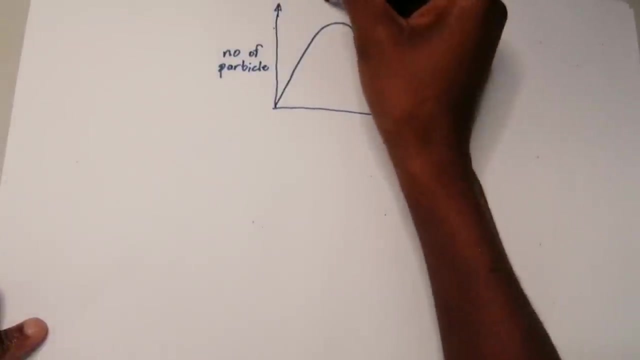 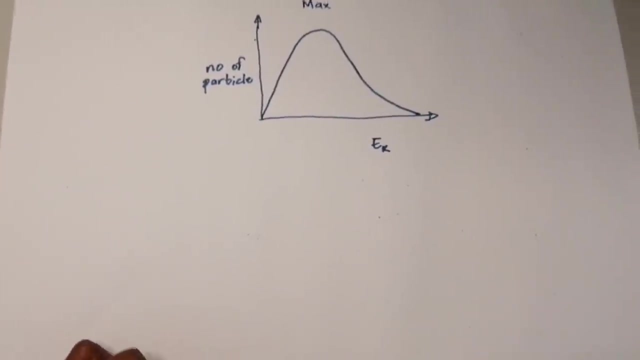 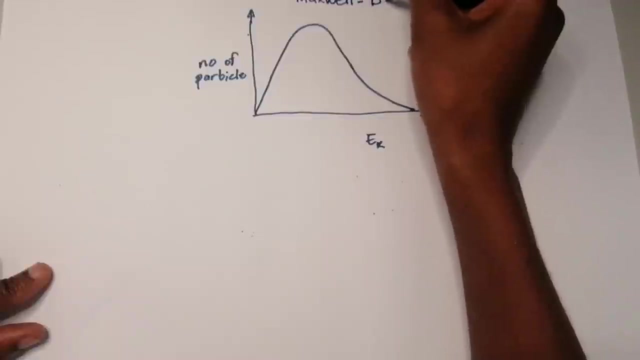 um that are colliding, okay, um against their kinetic energy. So this is what we call the Maxwell, okay, uh, all right, let me just adjust that a little bit. okay, So this is the Maxwell-Boltzmann distribution- Boltzmann. 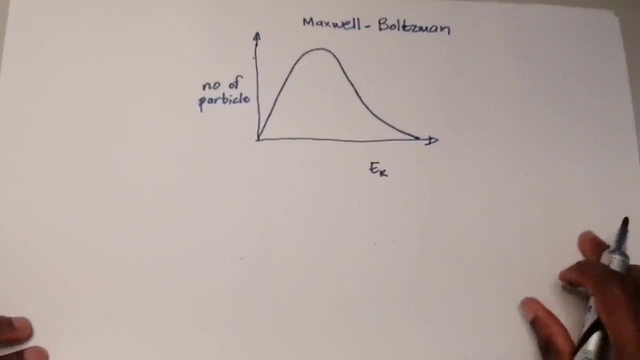 Okay, right. so this is the Maxwell-Boltzmann distribution, right? So this distribution is actually a statistical distribution curve. For those of you who've done stats, okay, you'd see this is a bell-shaped curve, right? Um, just to make you understand quickly what's happening on. 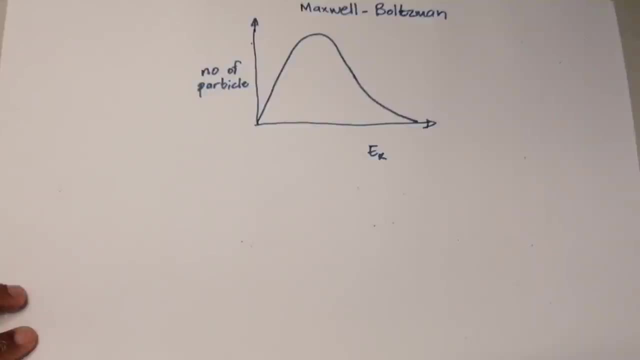 this curve right. So, if you think about it, we spoke about temperature, right Being the uh, average kinetic energy of a molecule. Now, let's say these are particles that are at temperature, at a particular atmospheric temperature, the um, uh, let's say the. 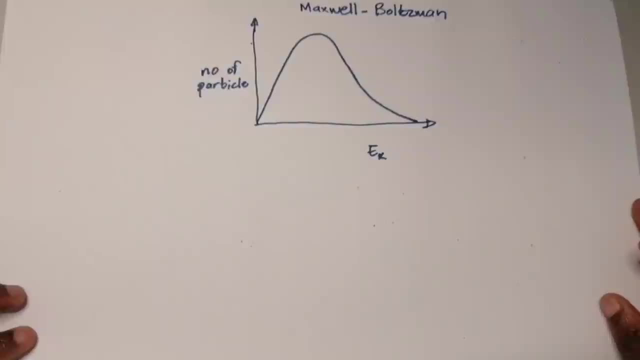 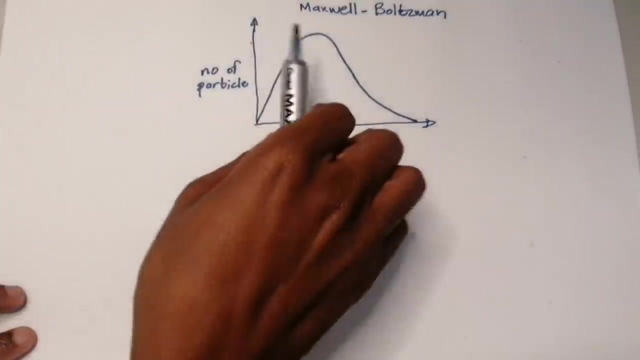 the, the, the temperature around. uh, say it's 25 degrees, right, But what you'll find is that the number of particles that are there have different kinetic energies. Now you'd see, uh, you'd find that there's less of them that have a lower. 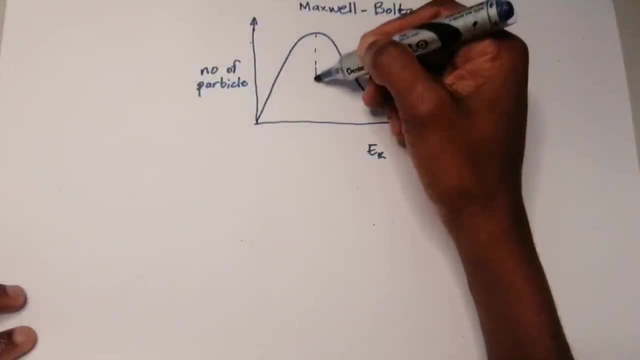 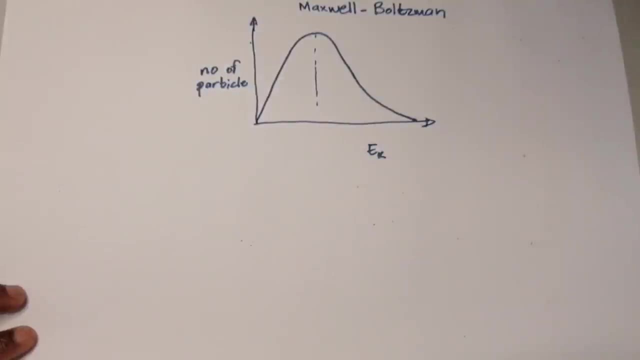 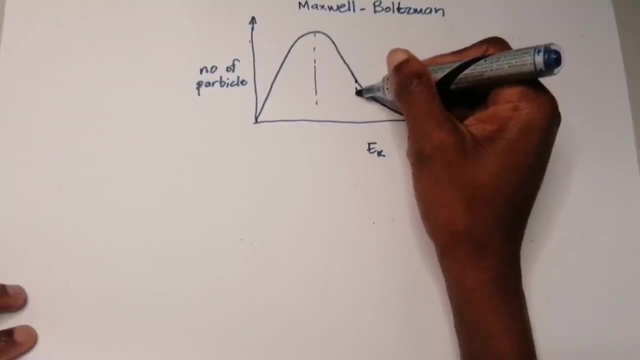 uh, kinetic energy, all right. So this one shows us the average kinetic energy. You remember? uh, we said that, uh, temperature, right, shows us the average kinetic energy. so that would be the average there. But let me just quickly get to something. So this one here is what we call the 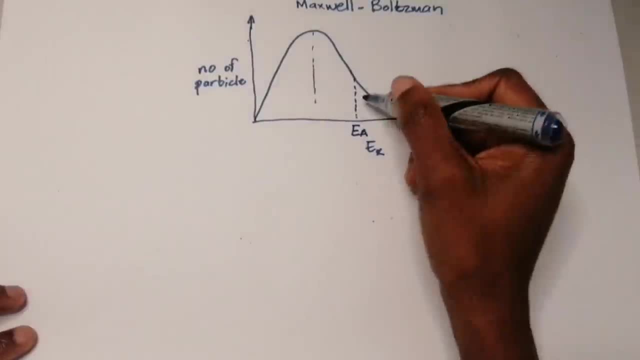 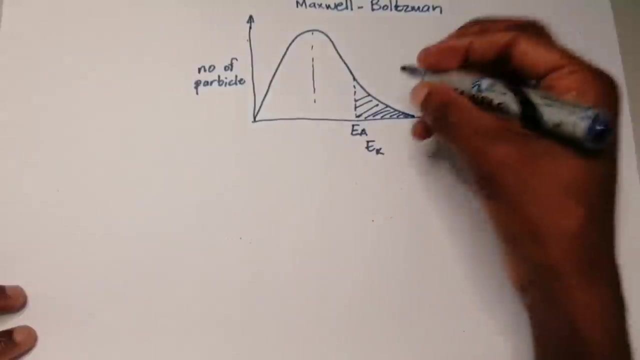 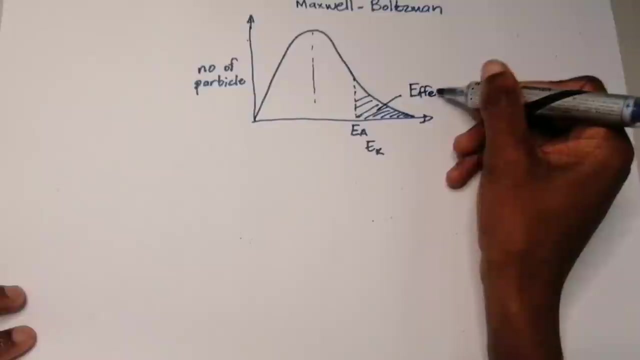 activation energy. Now let me just explain quickly. So it means any number of particles that have the energy, their kinetic energy, greater than this minimum here. anyone that crosses this line would then be able to form what we call effective collisions. So all of the 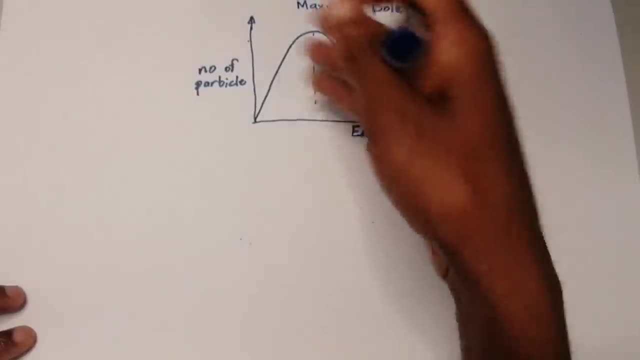 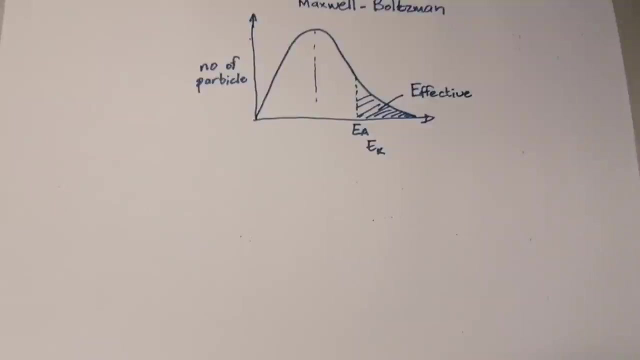 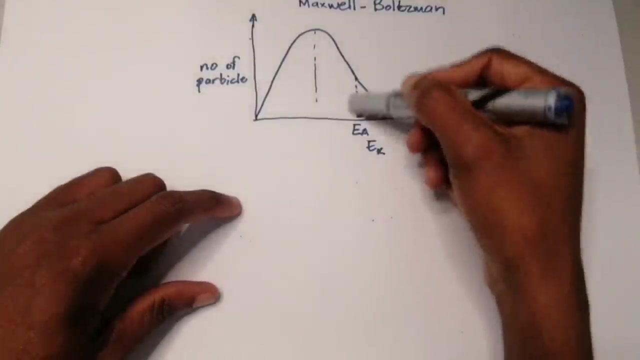 particles that are below here are not able to form what we call um effective collisions. So it means they're able to. it means they're able to collide, but they're not able to collide, So those collisions don't result in products being formed. It's only these ones that have this. 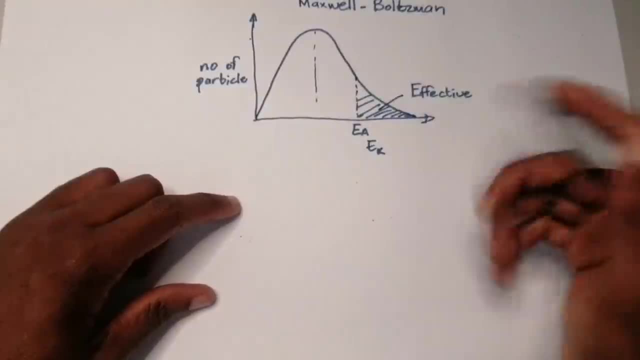 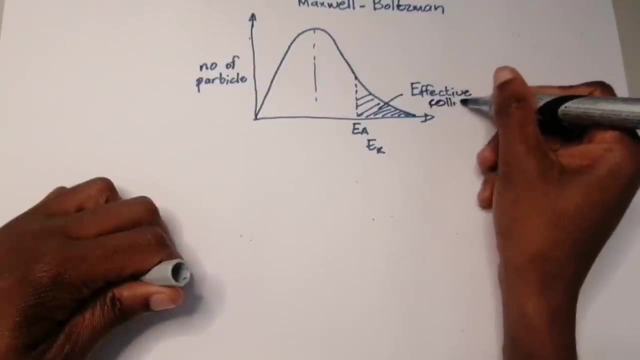 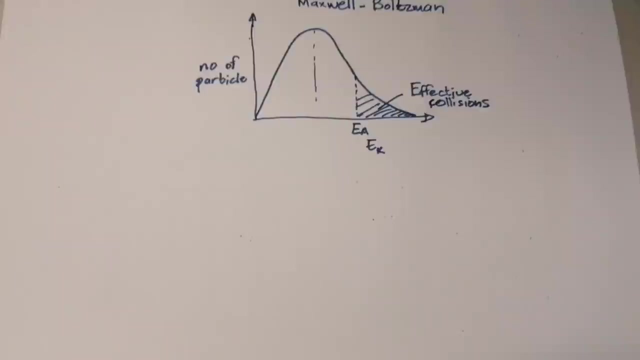 amount of energy and more that are able to form. what Effective collisions that can form products. okay, So these are effective collisions. Now look, ladies and gents, I don't know if I want you to spend as much time on this one here, um, but let me just explain something quickly about. 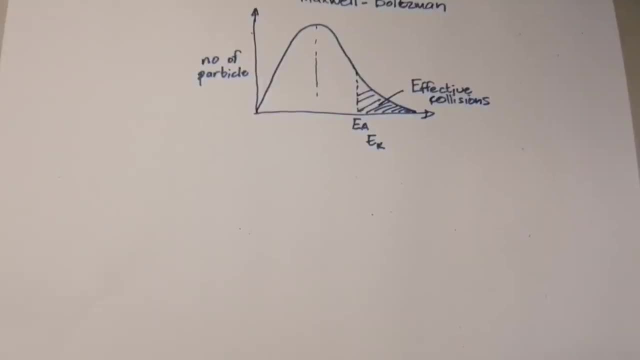 the Boltzmann distribution. Now, let's say temperature one: uh gives you uh that temperature there. okay, I mean that, that that shape of a curve. What if I give you uh the same reaction but at a higher temperature? 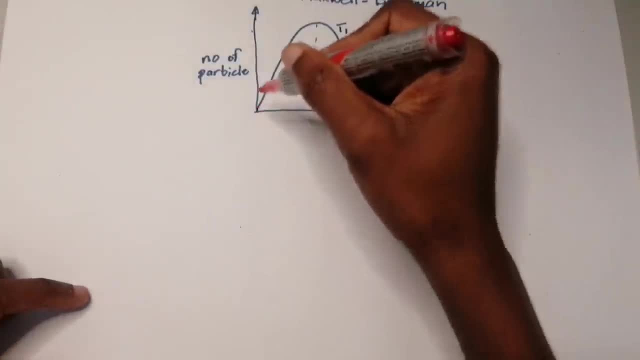 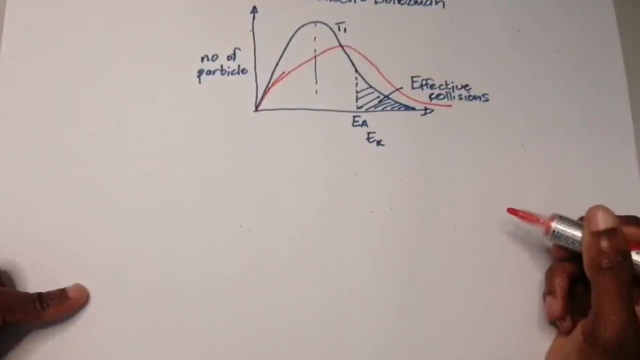 What happens So when I raise the temperature? well, I'll still get the same thing, but I want you to please note what happens. okay, This is what happens when I increase the temperature. Note what has happened. So it means this curve here, that is, at temperature T2, where, by the way, I am actually saying that the 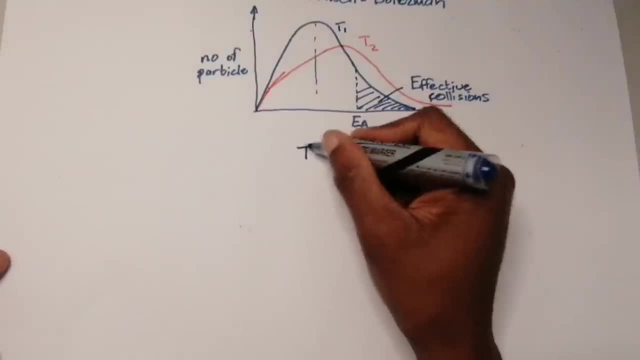 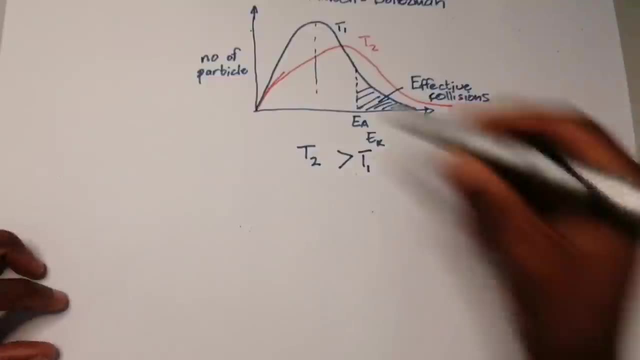 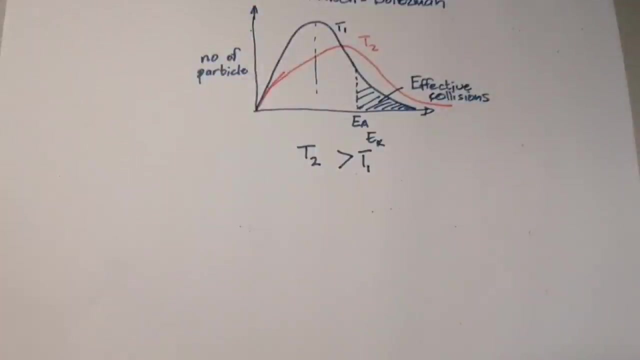 temperature T1,, or rather temperature T2, is greater than temperature T1.. Now, all of a sudden, what happens? um to the distribution? Well, the dis-, the distribution widens up. First of all. uh, your distribution, your graph gets wider. 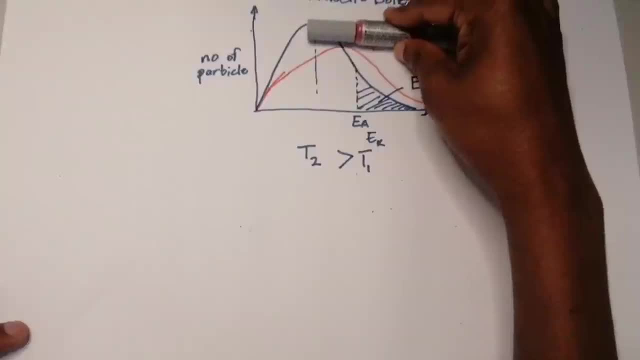 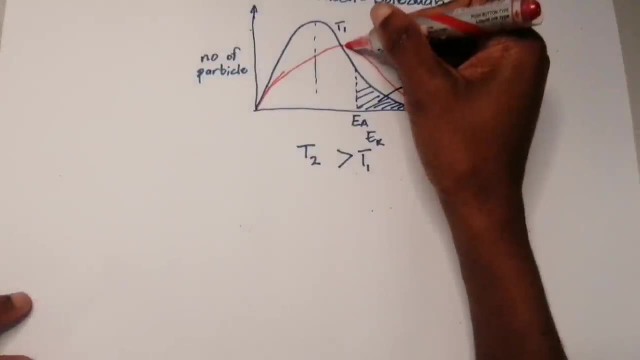 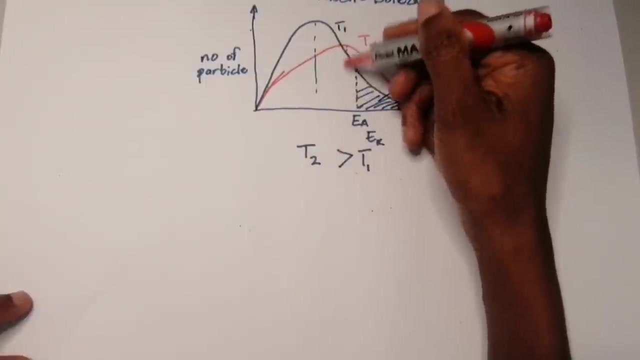 and then notice the peak of that curve got lower right. Um, sorry that my graph is not really the best. And then, secondly, what happened? The average kinetic energy? do you see that it's shifted now? My average is right here now. okay, So when you increase the temperature, 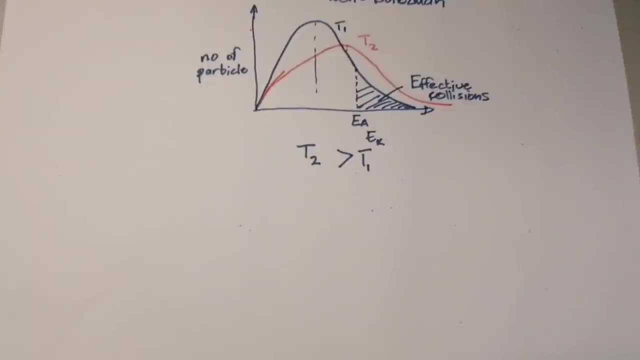 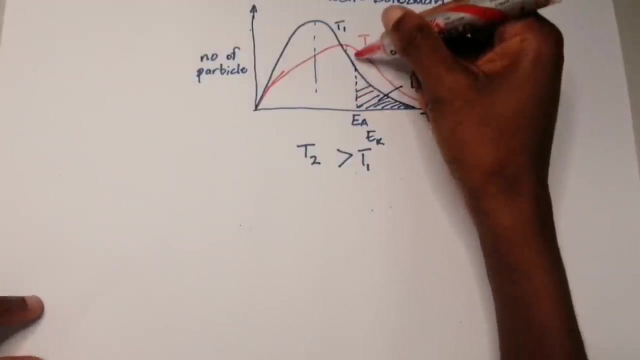 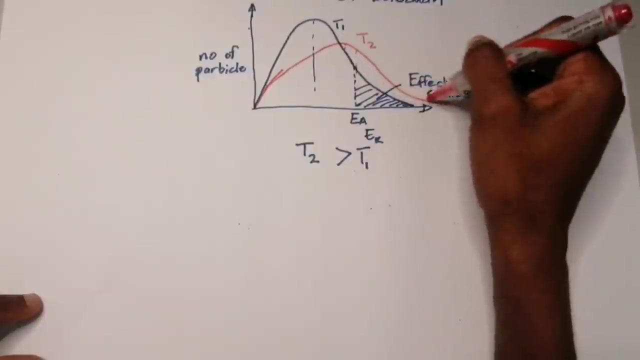 it increases your average kinetic energy and, as a result, because your average has increased. in that case, all right. Now I want you to note: we said this is our activation energy here. So now, when I increase temperature, can you see that more particles now are able? 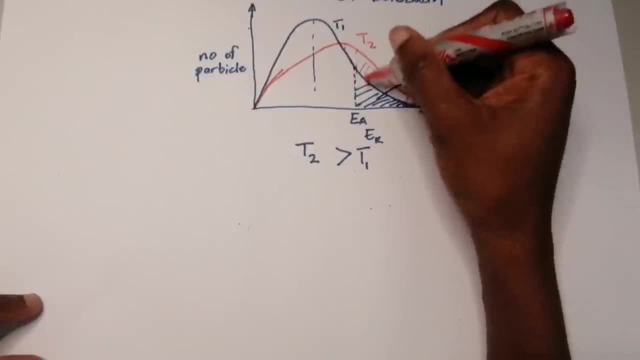 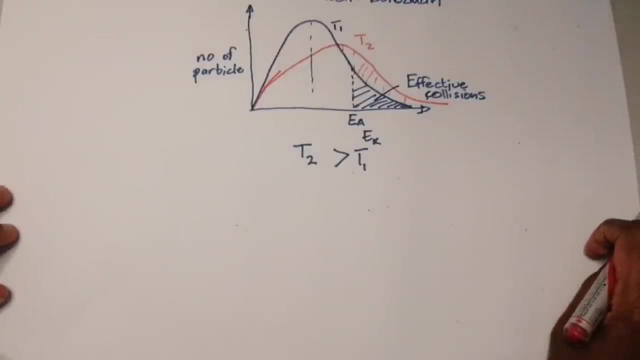 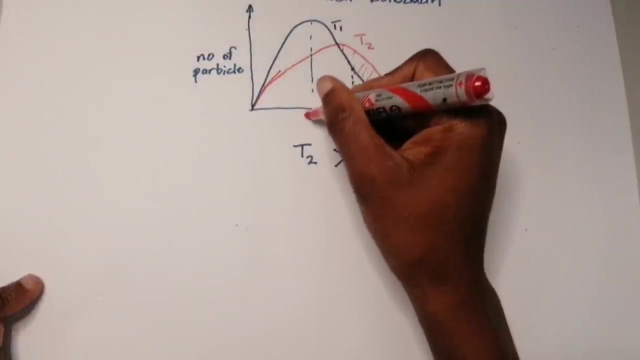 to have effective collisions, That that area there has become greater right. So in this case it means that more particles are able to have effective collisions. all right, So, uh, here's our kinetic. uh, um sorry, we say. uh, we said that's our average kinetic. 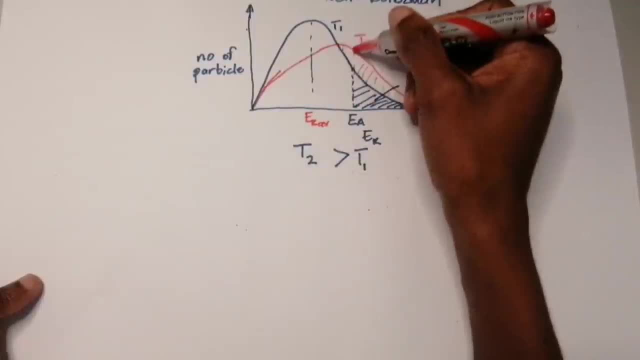 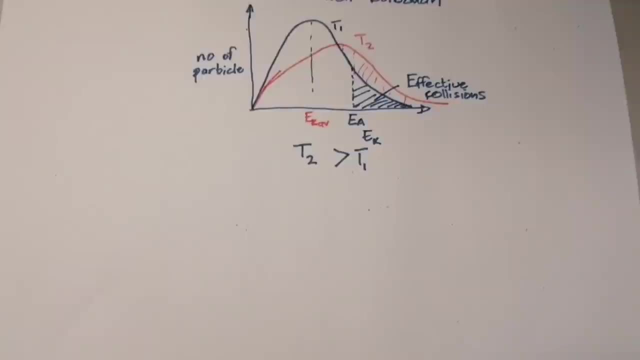 energy. So that's EK average. now, right, But when we've got temperature two, which is greater, our average kinetic energy is now much higher. all right. So as a result, ladies and gents, as I said, I don't want us to spend as much time on this, right, Uh, but nonetheless. 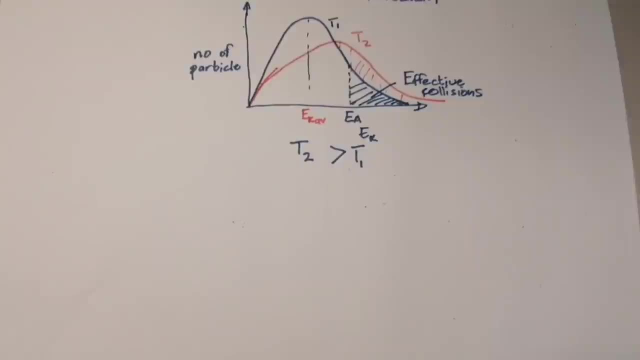 I want you to know how to explain it, and I want you to know how to um uh, to make your argument, to know the difference when they give you different types of distributions or shapes. right, And then just one last thing: What happens when I add a catalyst? Remember. 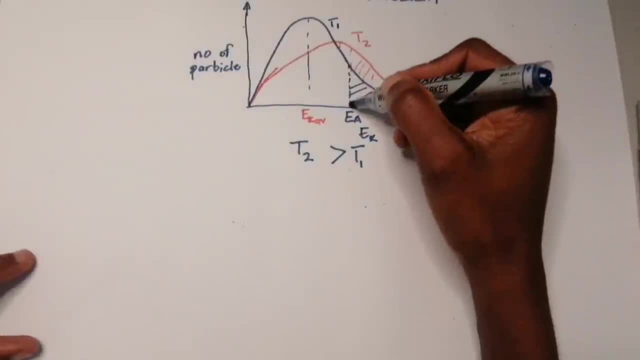 you remember what we said about a catalyst? We said what it does is that it decreases this value here. So if that was my minimum uh uh kinetic energy required, so a catalyst would now shift this value here. Now what happens When I shift the kinetic, when I 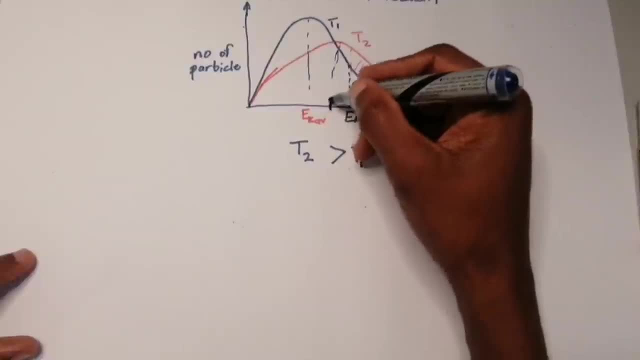 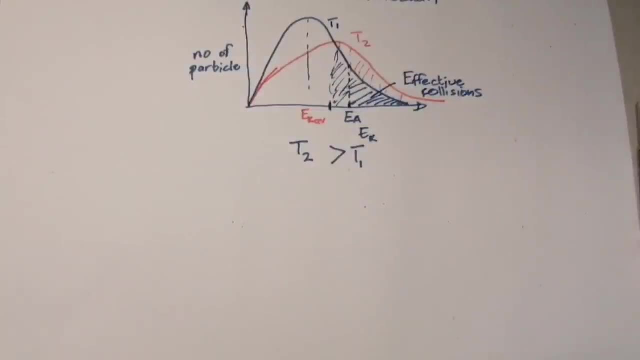 lower the activation energy. by the way, when i lower that activation energy, it means now more particles are able to react. okay, right now, here's what i want us to do. ladies and gents, i know that this is quite a a a big chapter. i know that it has quite a lot of things that i can explain. 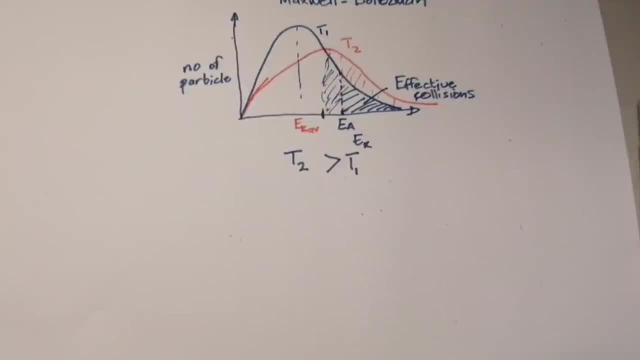 but what i want us to do is just to try and delve in as much- um- uh, you know past exam questions as we possibly can, and then what i'll do is that i'll explain some of the things as i answer questions. i hope that's fine with you, right? okay, let's get into it all, right? um? so i take this question from: 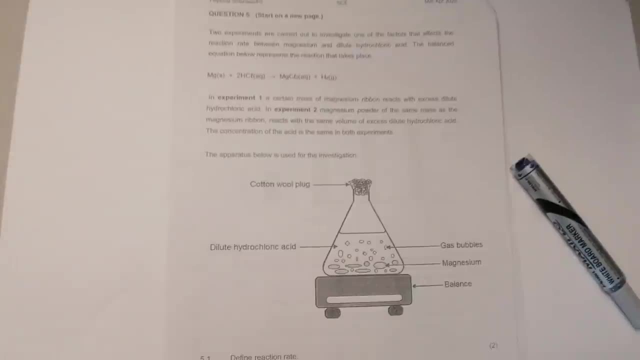 the march- april paper of 2020. uh, this was for the senior certificate exam, but, um, i'm sure you can get this paper, uh somewhere else. um, let's try and look at, uh, what this paper, this question, entails. so they say we've got two experiments that are carried out. 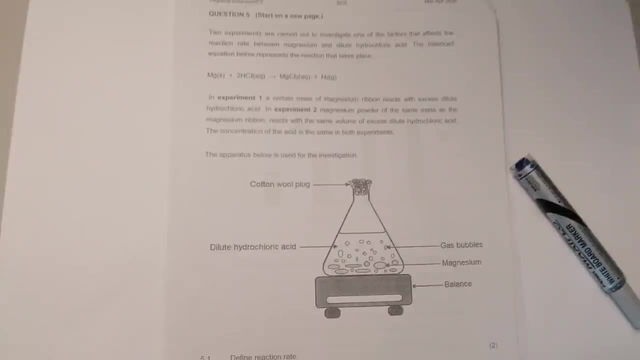 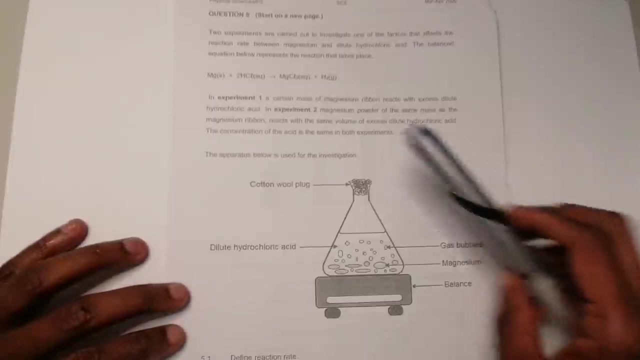 to investigate one of the factors that affect their, their reaction rate. you remember we've got five factors right between magnesium and dilute hydrochloric acid. right, they say the balanced equation, uh, below represents the reaction. so they've given us uh the uh, the reaction they say in experiment one, a certain mass of magnesium ribbon. can you see? 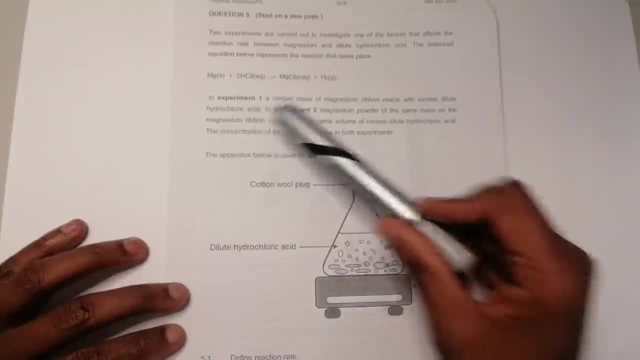 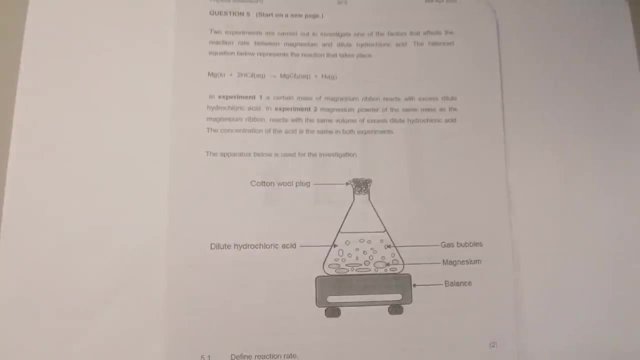 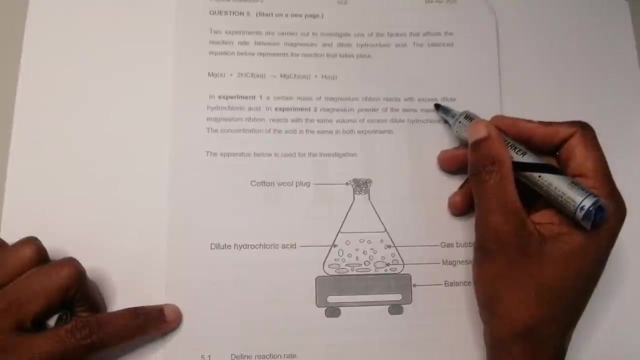 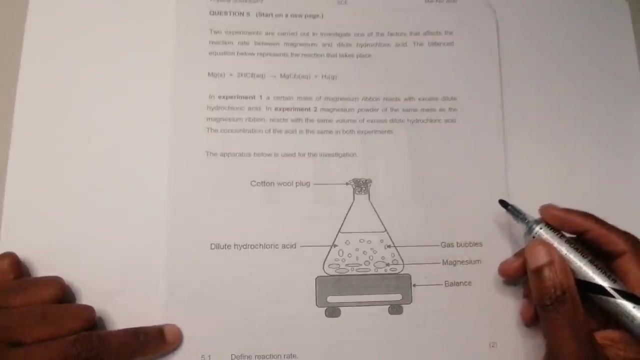 reacts with excess dilute hydrochloric acid. now, ladies and gents, i know i haven't gone through this with you yet, but i want you to note: once they tell us something is in excess, then it means that, um, the other one immediately remains, becomes my what we call the limiting reactant or the limiting reagent. right, so it means. 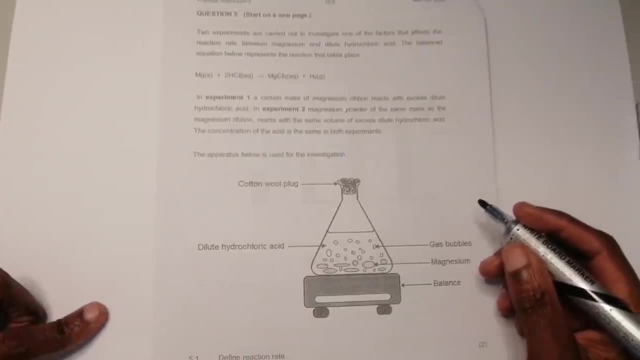 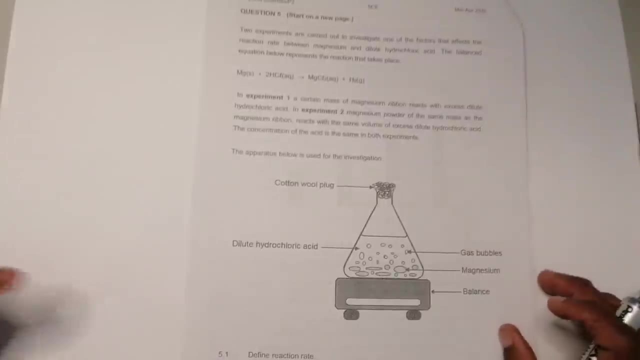 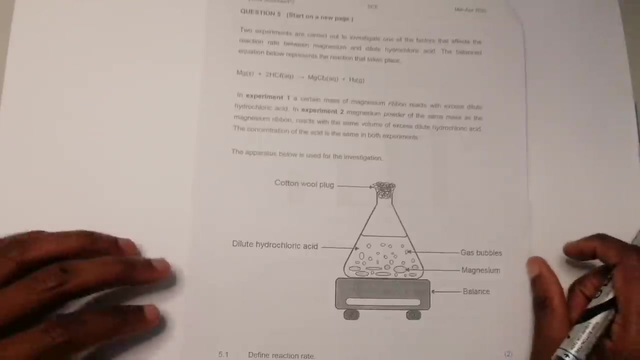 the other one that is not in excess is the one that's going to actually limit the extent of my reaction. so it means it's going to run out first, right, and so if it runs out first, um, it's going to determine the amount of products that i'm going to form. okay, right now, let's continue. okay, they? 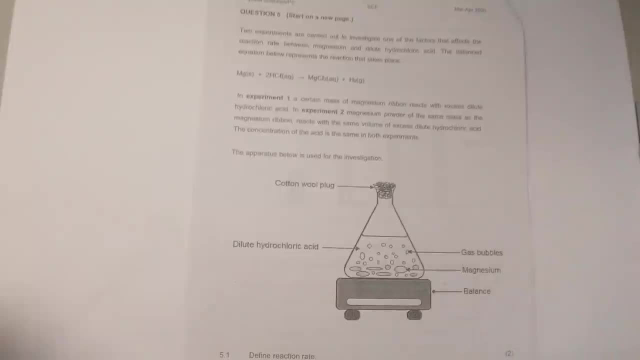 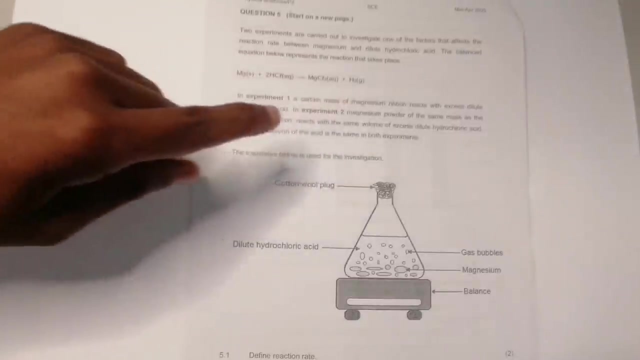 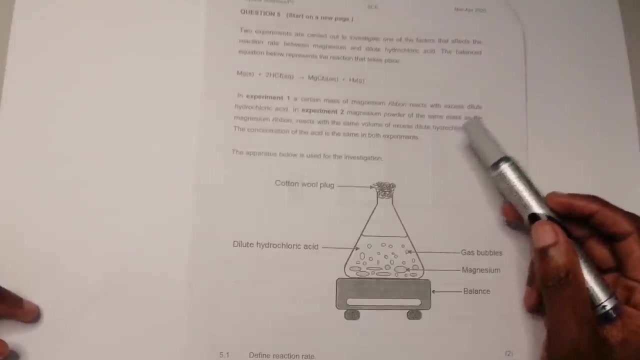 say, in experiment two, magnesium powder. now notice what they've done. in experiment one they used magnesium ribbon, can you see right? and in the next one they use magnesium powder, right? so in this case, what they are simply doing, they are changing something between the two reactions. okay, now of course we should already. 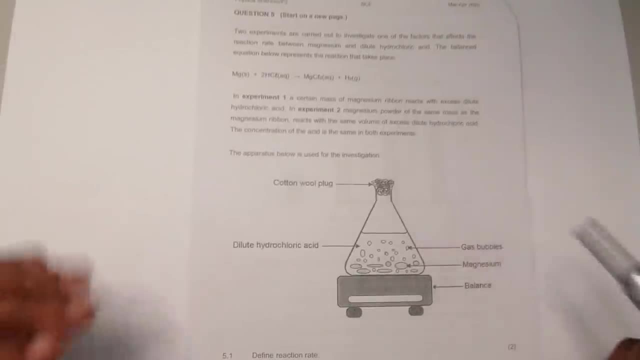 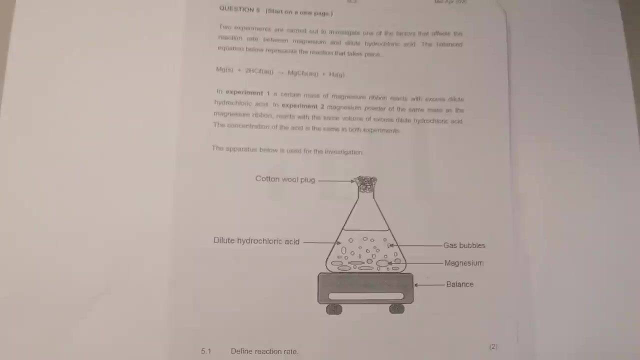 note that the one that's in powder form. what have they done? they have now divided it up even more. they have changed what we call the state of division. all right, right. so they say magnesium powder of the same um, of the same mass as the magnesium ribbon right reacts with the same. 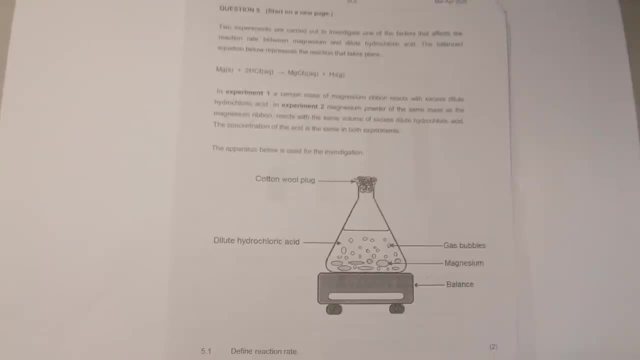 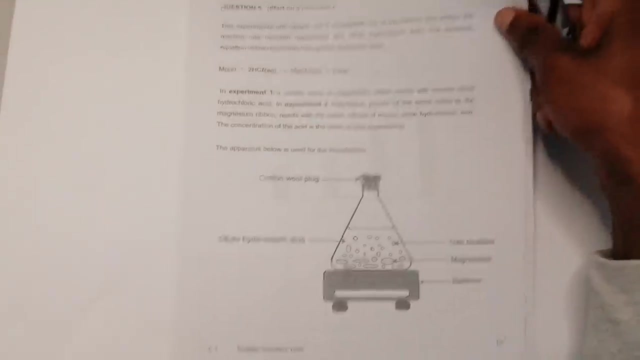 volume of excess dilute hydrochloric acid. the concentration of the acid is the same in both experiments. now let's get into it. they say the apparatus below is used for the investigation. so there's our apparatus, okay, um, of course the americans would say apparatus. 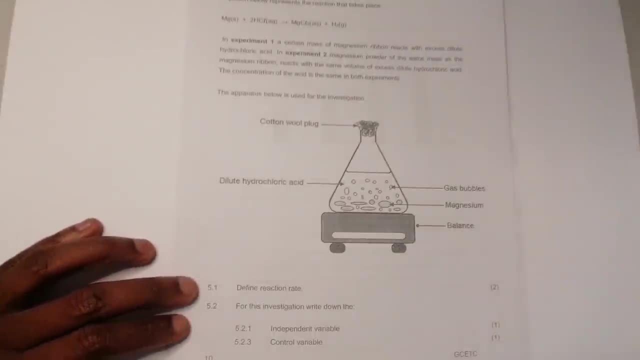 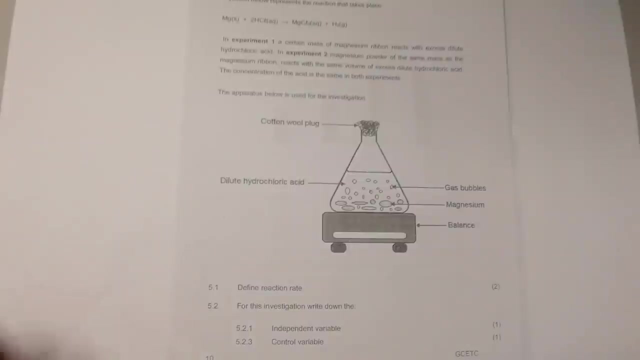 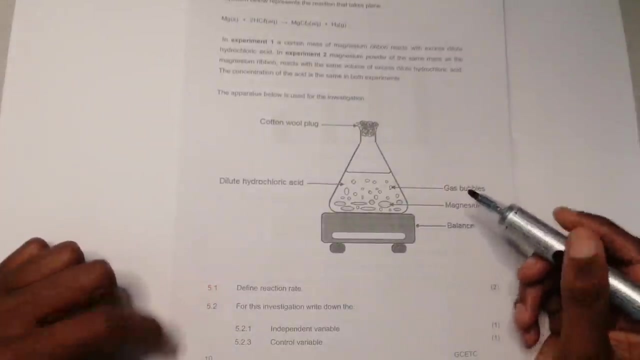 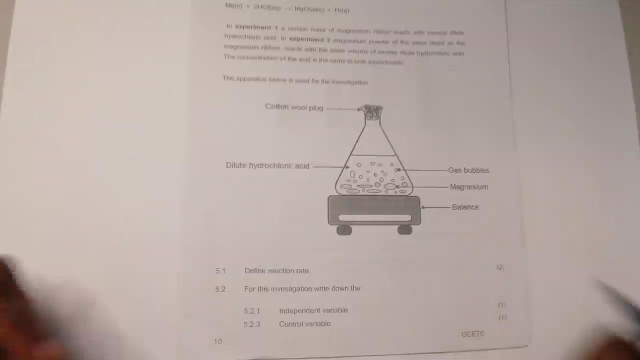 okay, so, um, so that is happening there. you can see some gas bubbles forming. but why are those gas bubbles forming? it's because we are also producing, or rather we are producing hydro hydrogen gas there. okay, right now they say: for this, uh reaction, now uh, defined reaction rate. remember we said it is the change in the amount of products formed. 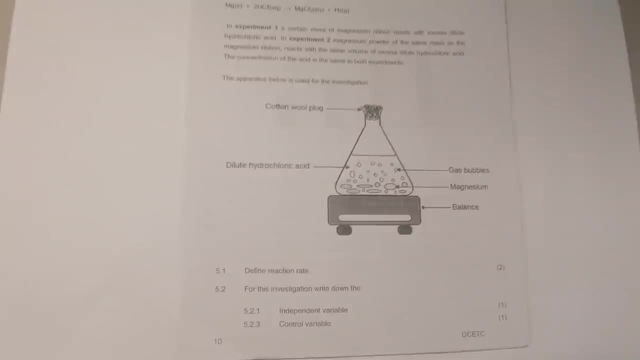 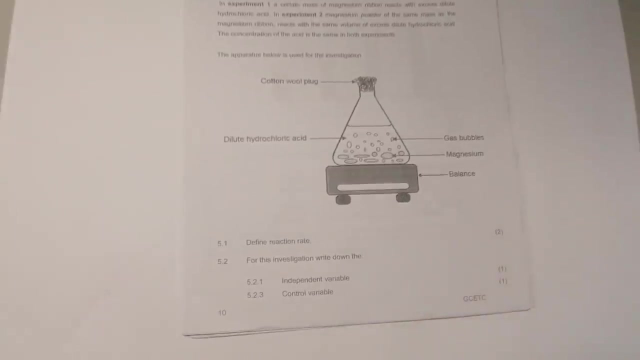 per unit time, right, okay, so it's the change in the amount of products formed, or you can say it's the change in the amounts of reactants used per unit of time. okay, and then they ask us this very important question. they say: for this investigation, write down the independent. 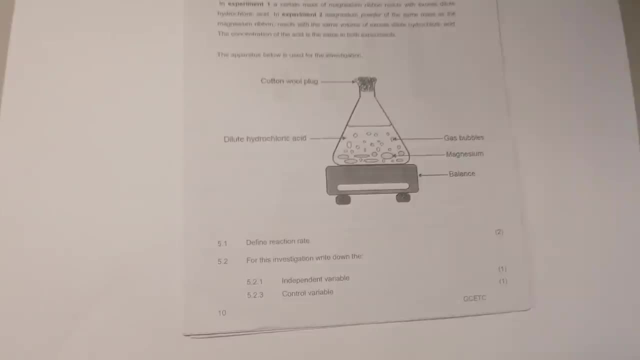 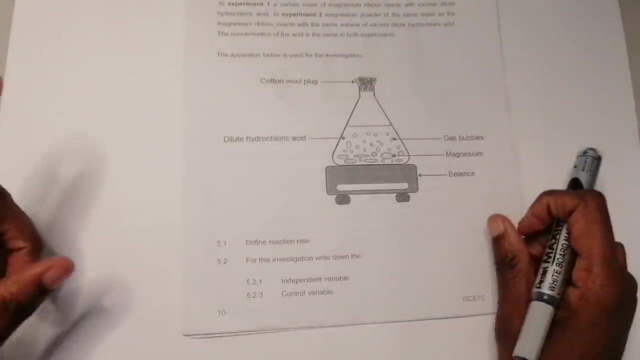 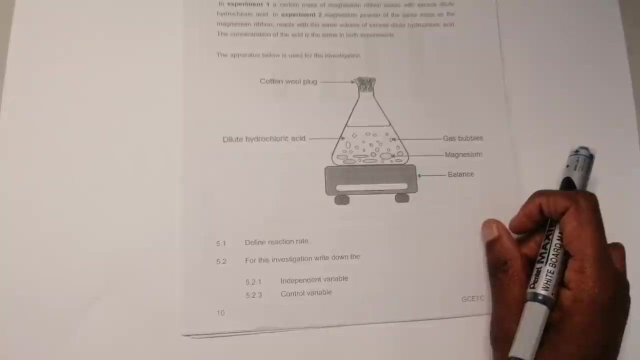 variable. ladies and gents, i want you to please note what is an independent variable? so, between the two reactions when they took place, we've got experiment one and experiment two. there's something that we changed in the two experiment, isn't it? what is it that we changed? right, remember, in the 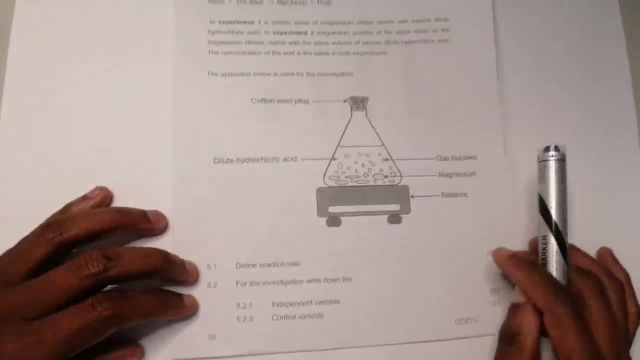 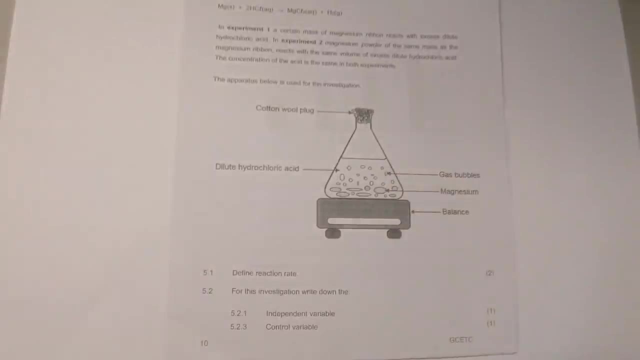 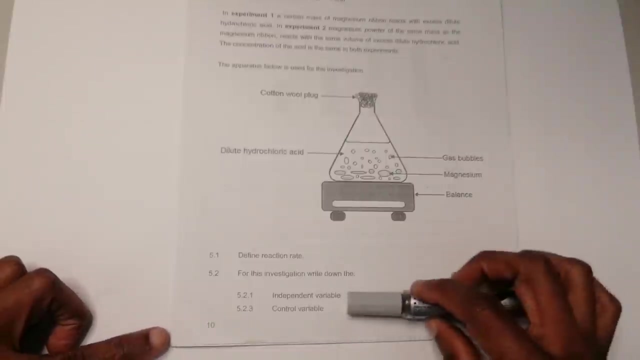 one we were using magnesium ribbon right, and then in the other one we were using magnesium powder. so what did we change? everything else remained the same, except the state of division of what magnesium there it is. so in this case, what we we change between the two reactions is called our independent. 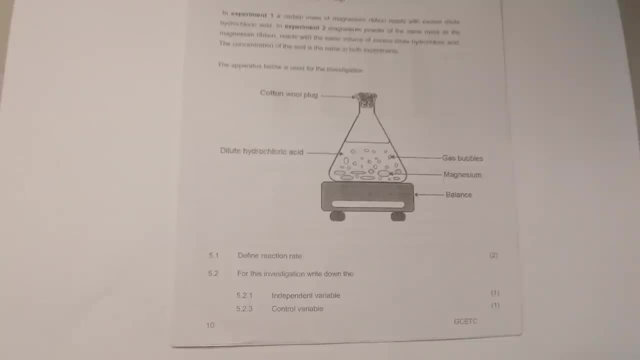 variable. what did we change? the state of division of magnesium. all right, so our independent variable is the state of division of magnesium. now, i know they didn't ask us this, but let me just say it whilst i'm edit. so what would be my dependent variable? now, think about it when i change the 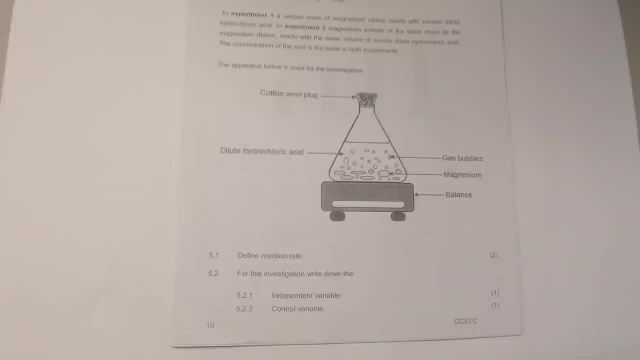 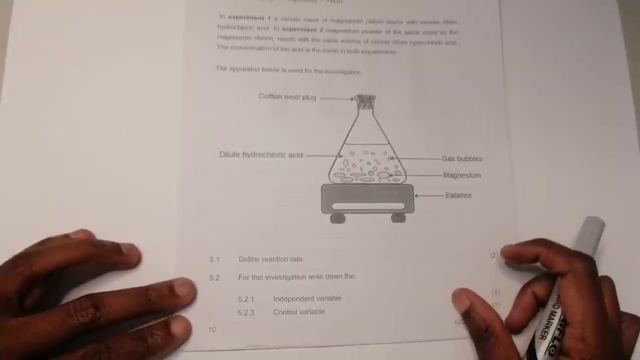 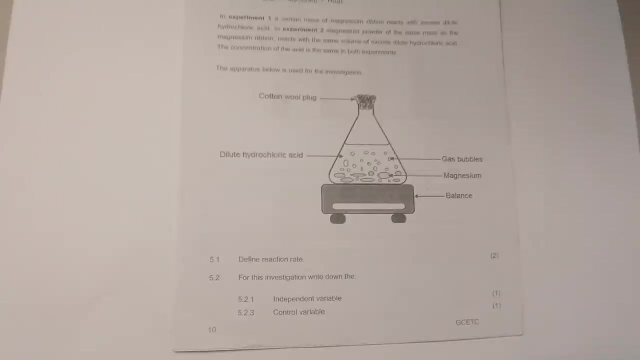 state of division. it affects the rate of reaction. so it means that rate of reaction- okay would be- would be my dependent variable and please, i want you to always note when we're doing rates of reactions: uh, rate of reaction- okay would be my dependent variable all the time. okay, now. and then they ask: 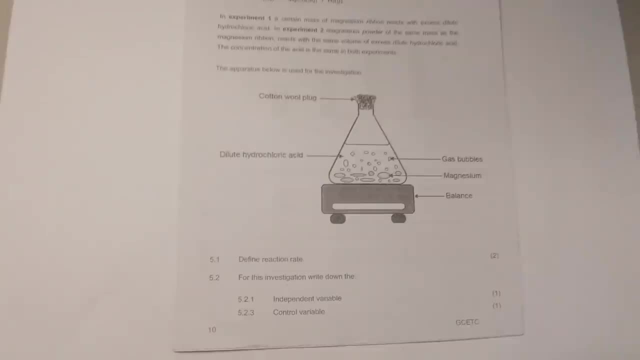 us, um, write down the control variable now, please. i want you to note we've got several of them. okay, i suppose in this case, they want you to um the uh, to, to, to actually just write one control variable. but think about it: what, what is a control variable? it's something that you need to make sure that you. 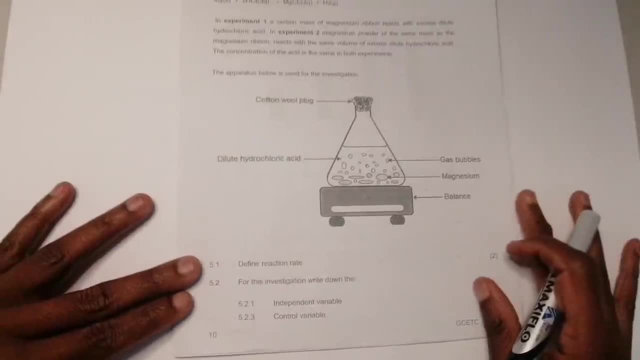 keep in mind when you're doing a control variable. it's something that you need to make sure that you keep in mind when you're doing a control variable. it's something that you need to make sure that you keep the same now in order for this to be a fair test, in order for it to be a fair experiment. a. 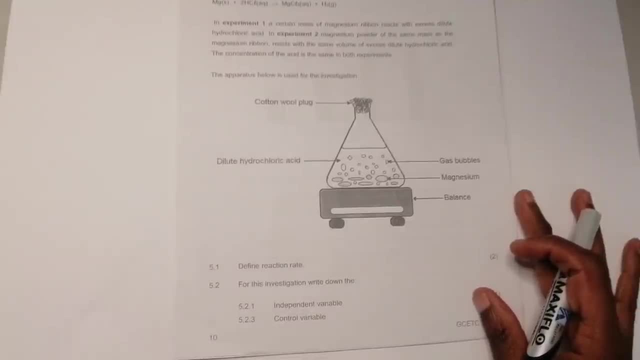 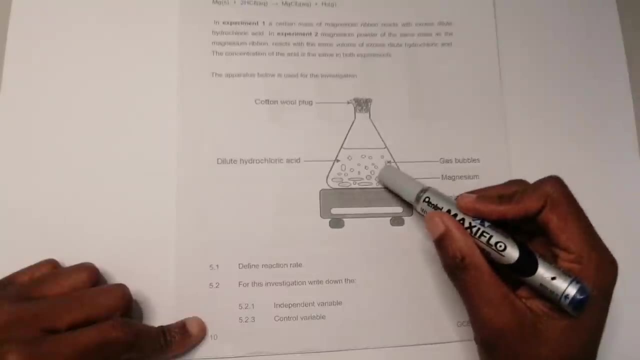 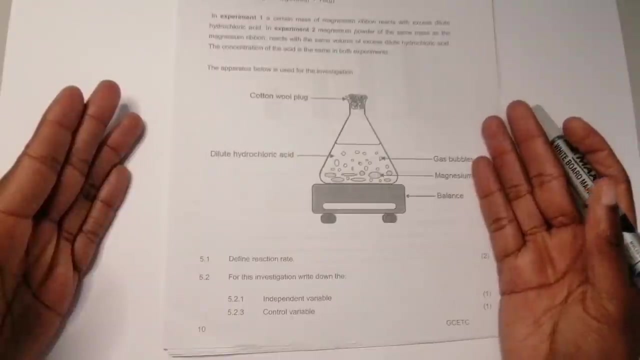 fair test between the two. you only have to have one independent variable. so what do i mean if we've changed the state of division? um one we are using ribbon and in the other one we are using powder, right, you can then have powder here plus a higher temperature. okay, so the need for a higher temperature? 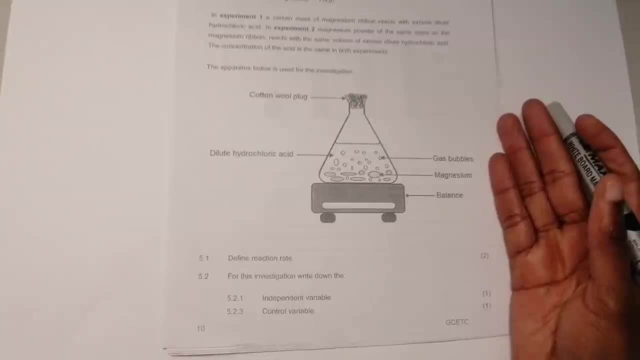 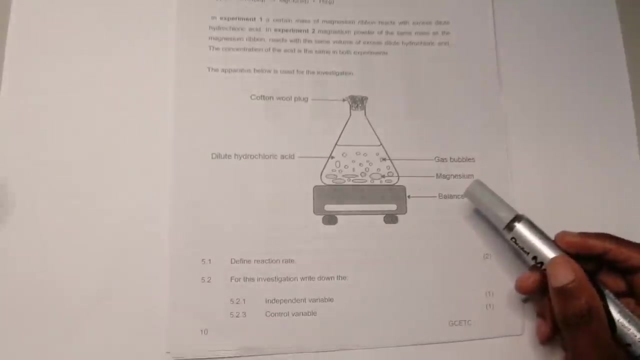 to be only one thing that is different between the two, so that when we make our conclusion, we know for a fact that it's definitely the state of division that affected the rate of reaction. okay, so control variable would be something that stays the same, okay, between the two reactions, right so 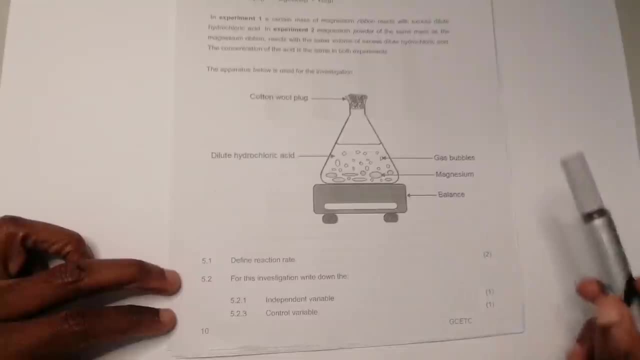 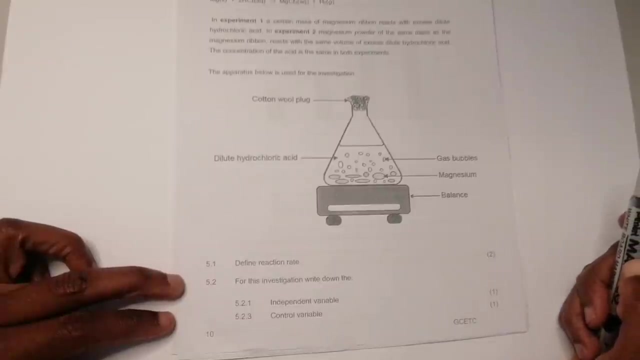 what stayed the same? i'm sure you've guessed it by now. we saw how they actually told us. it's the concentration of what? hydrochloric acid, right? um what else? it would be the volume of hydrochloric acid. um, what else can we keep the same? it could be the type of beaker that you use. 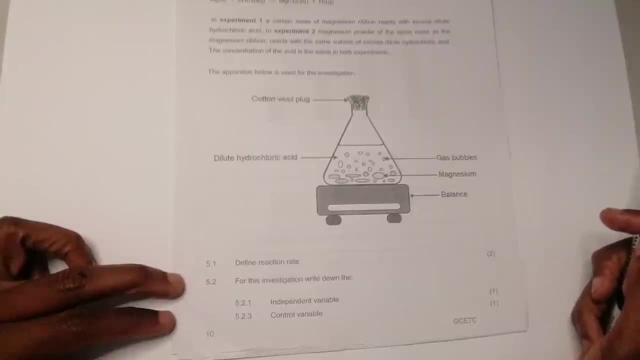 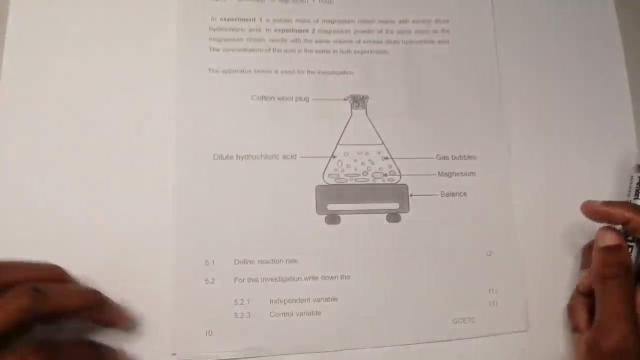 right, um, what else can we keep the same? the temperature at which you conduct the experiment? you need to definitely make sure that you keep those the same. so, in this case, you can mention any of those and if you are able to think of, you can mention any of those and if you are able to think of, 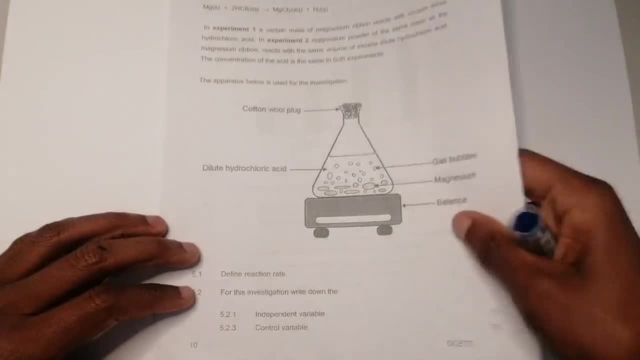 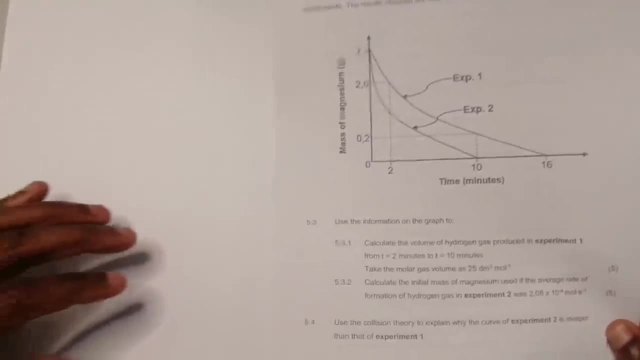 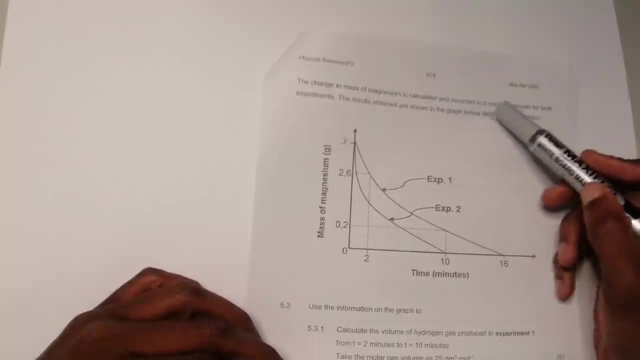 more examples. you are more than welcome, ladies and gents, right now. let's get to the next part of our question. right now they say to us: the change in mass- okay- of magnesium is calculated and recorded in two minutes. uh, two minute intervals for both experiments, okay, so here's. 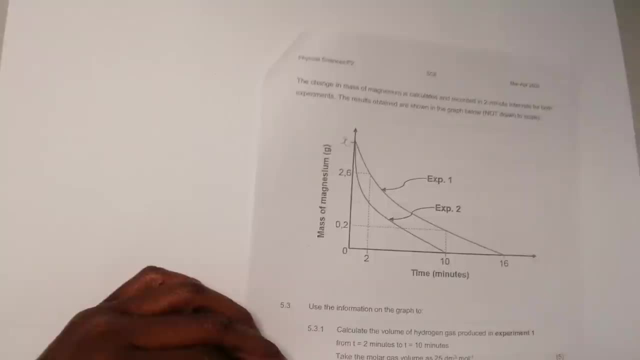 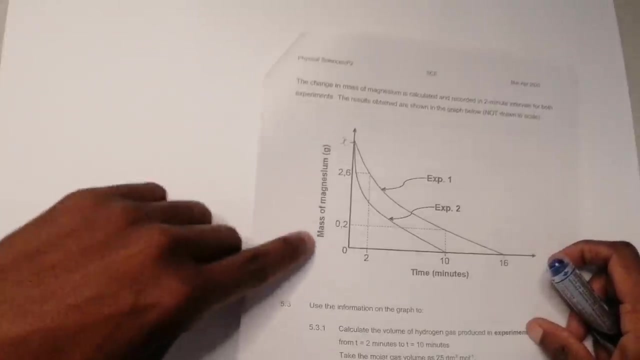 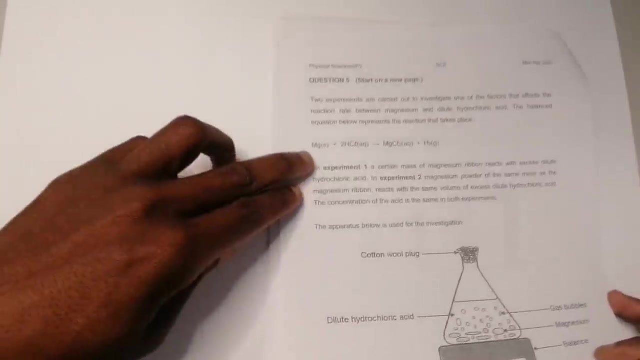 the graph and the results obtained are shown in the graph below, and it's not drawn to scale right. so now, what is this change? showing us? the mass of magnesium? obviously, magnesium is reacting. you remember that. so magnesium is reacting, and what is it forming? it's forming magnesium chloride and 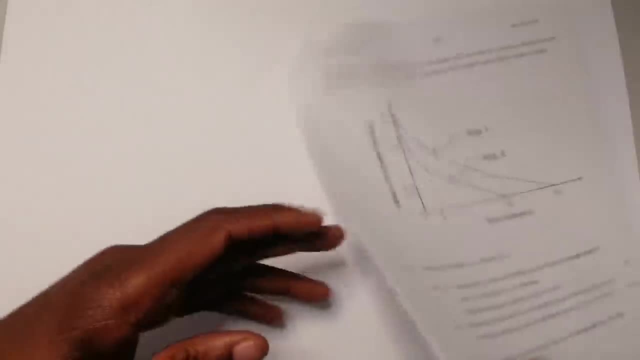 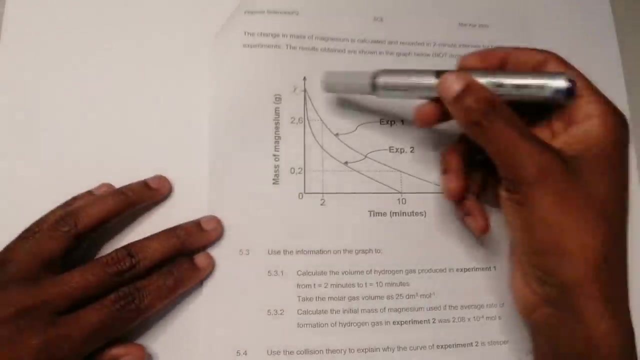 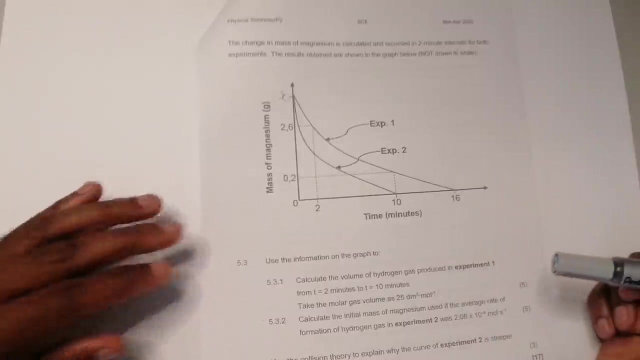 it's also forming hydrogen, so obviously, as it reacts, what would happen to the mass of magnesium? it would actually decrease, right? so it means that the mass of magnesium would keep decreasing until- remember, it's our limiting reagent- until it runs out, right? so the experiment would stop. 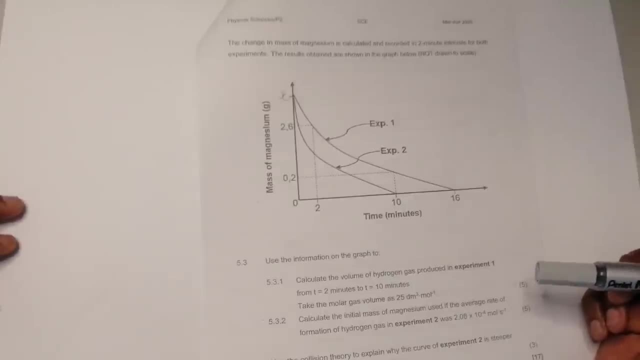 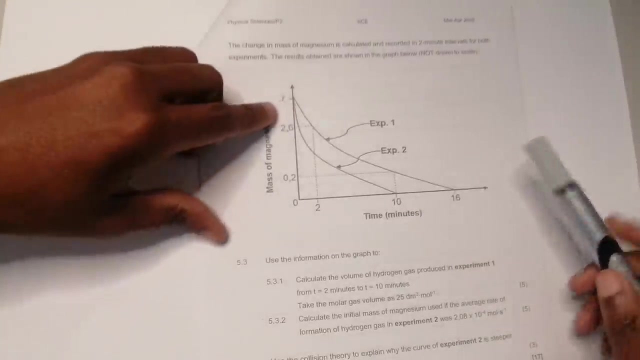 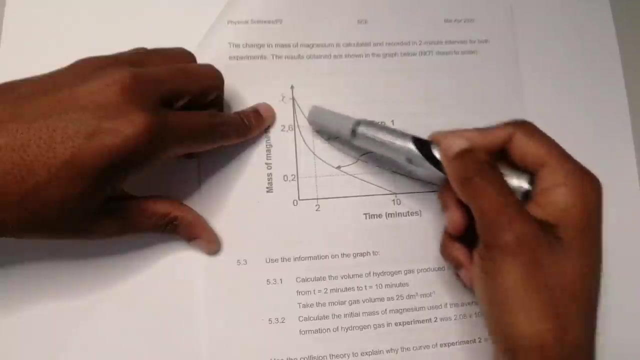 immediately when we run out of magnesium. okay, right now- this is for experiment one- i want you to notice something. so this is the magnesium decreasing the mass of magnesium, and why is it decreasing? because it keeps reacting and reacting. so you are forming less and less. or rather, you are decreasing the mass of magnesium, and why is it decreasing? because it keeps reacting. 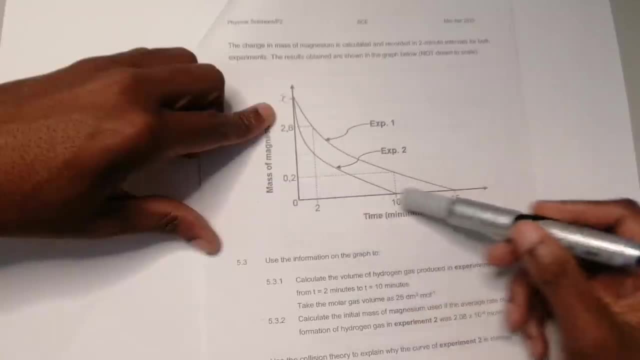 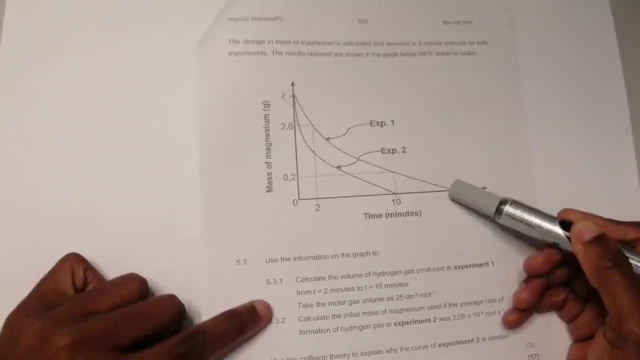 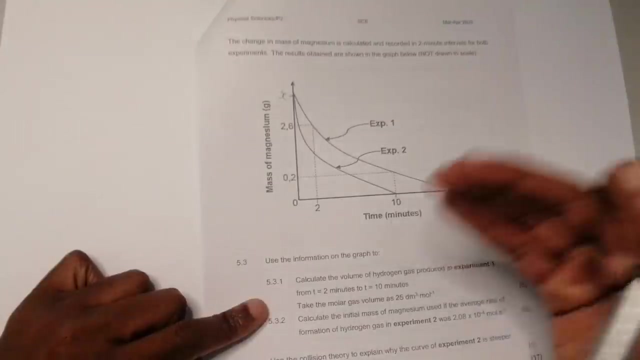 you have less and less magnesium until it becomes zero, and it does so after 16 seconds in experiment one. but then in experiment two, you remember we had magnesium powder. okay, so what happened? of course, i'm expecting that the one in powder would actually um, um, you know, um, get to completion. 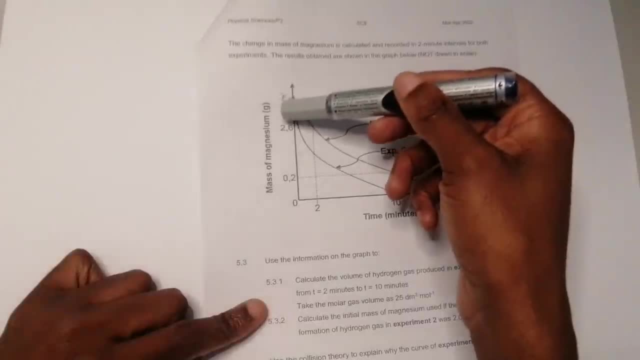 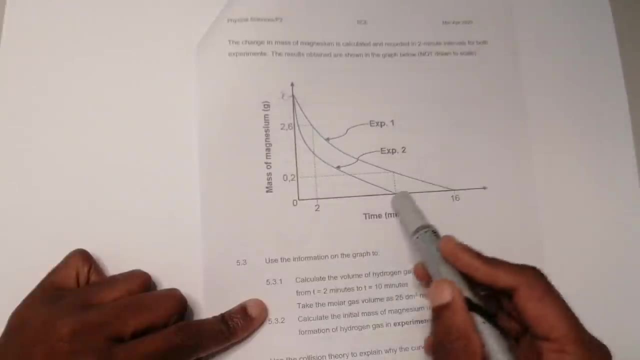 much faster, isn't it? so in this case, look at it, it's decreasing. it's got a very sharp decrease and in this case it actually it reaches completion at 10 seconds right. so it's actually six seconds less than the first one. so, in this case, what is it showing us? it's showing us. 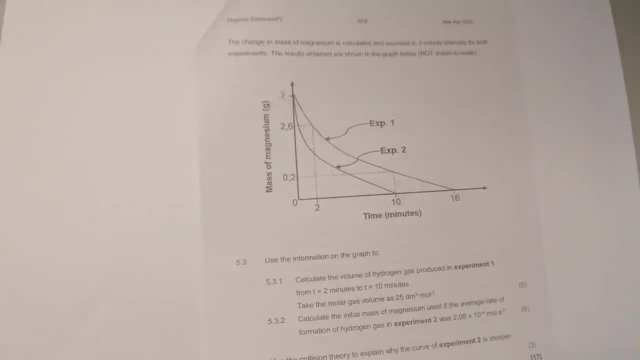 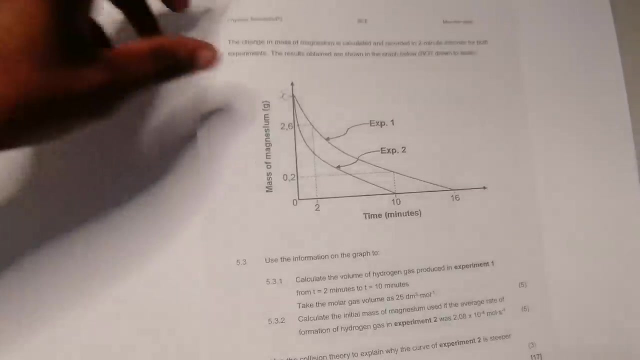 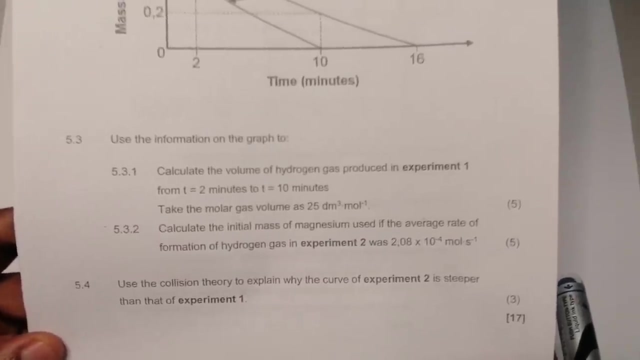 that when we increase the surface area, or when we increase the state of division, then it obviously increases the rate of the reaction. now let's get to the question quickly, right now. what do they say to us? they say: use the information in the graph right, calculate, uh, the volume of hydrogen gas. 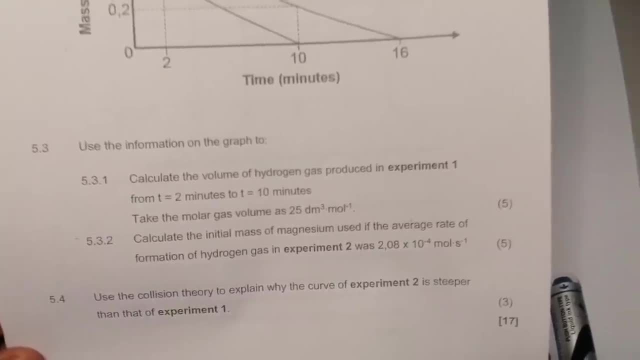 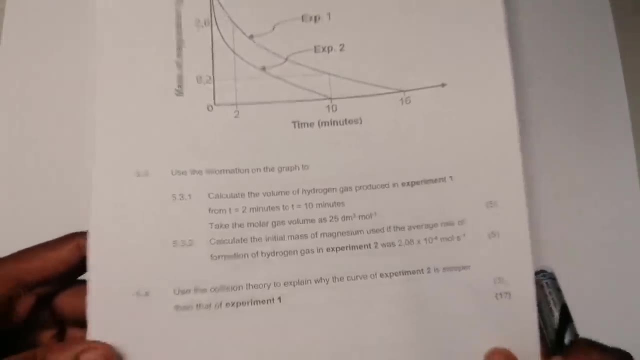 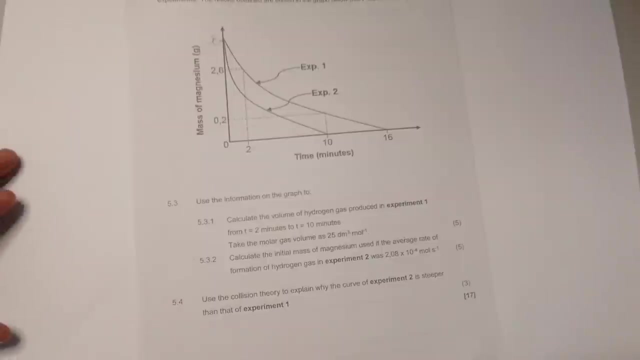 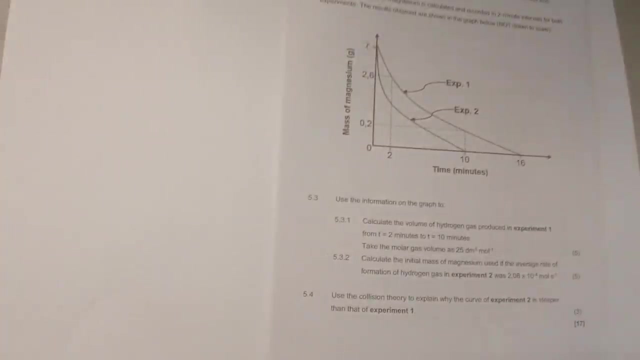 produced in experiment one. okay, right, so we're going to use the information in the graph, all right, to calculate, um the volume of hydrogen gas produced, right? um, at some point or the other, i'm gonna make a video on geometry, because i i really think that it is an important part um of what we must know, right? 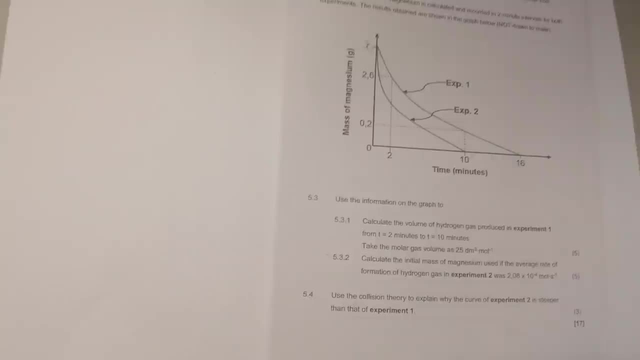 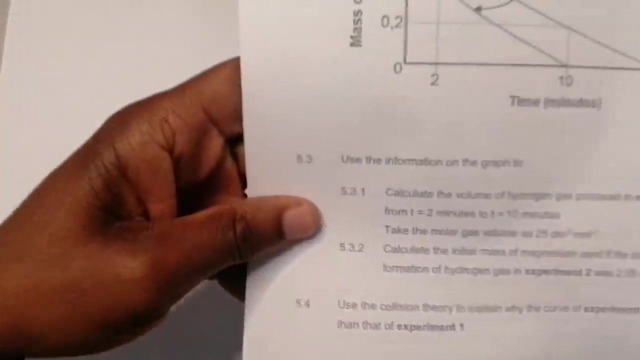 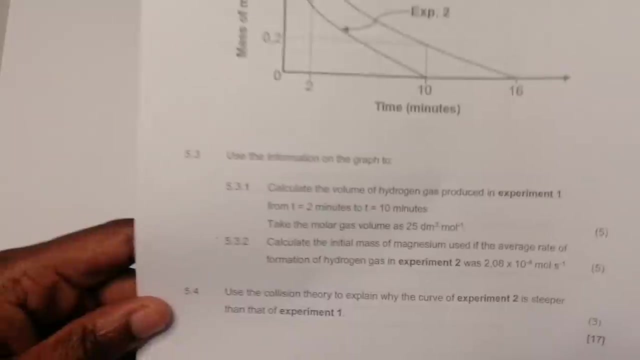 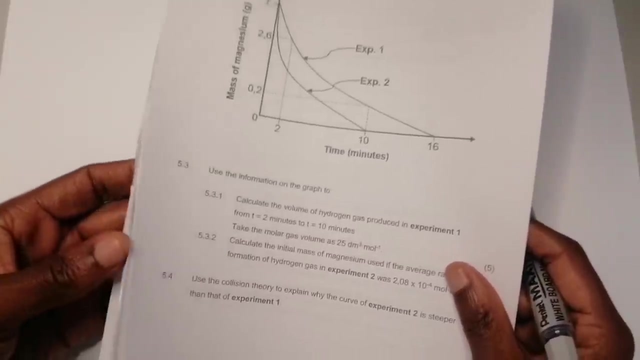 um right, they say to you: uh, take the molar volume, uh, the molar gas volume to be 25, uh cubic decimeters per mole, right? uh, so there's a molar volume there that is vm, right? so how do we conduct this? um this question, okay. 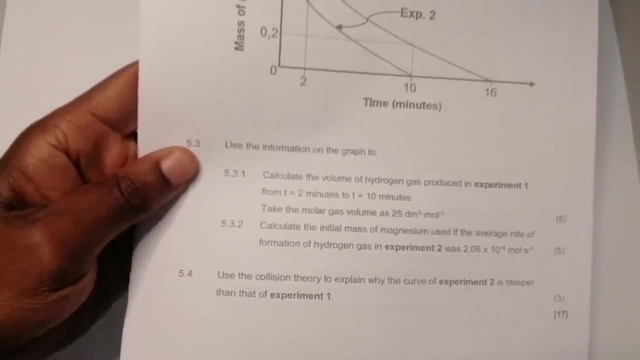 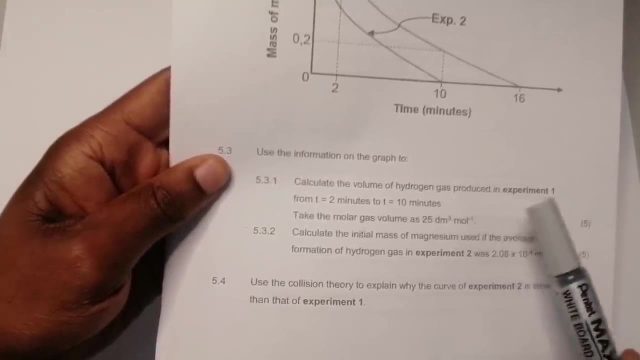 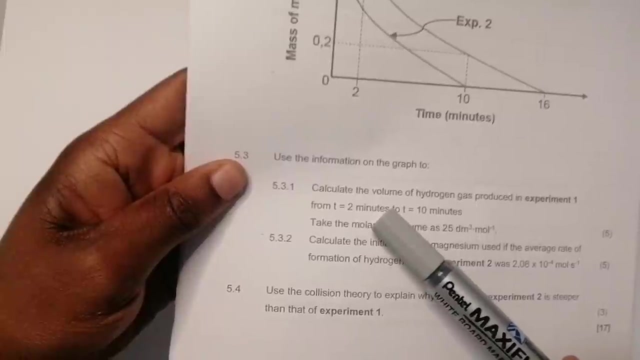 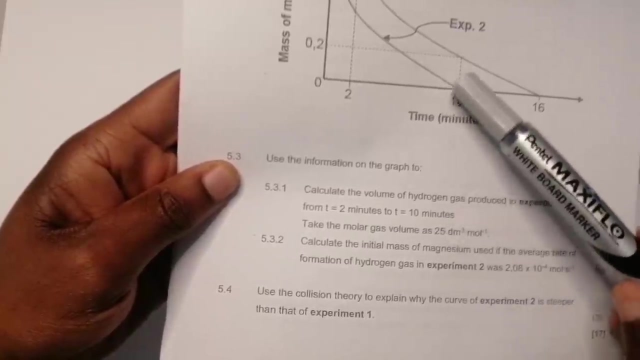 right. so one thing that i want you to notice is that we are now looking at um the volume that is produced, but not just at any particular place. they did say specifically: from uh, t is equals to two minutes. so from that point there, uh to t is equals to 10 minutes. okay, which is that point there? and they specifically said for: 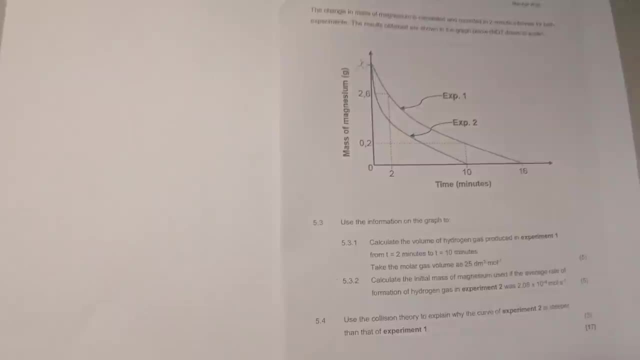 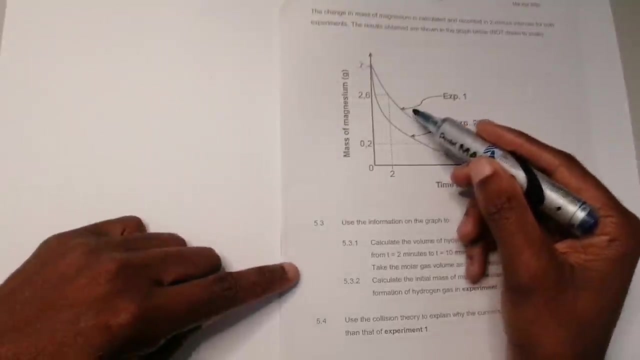 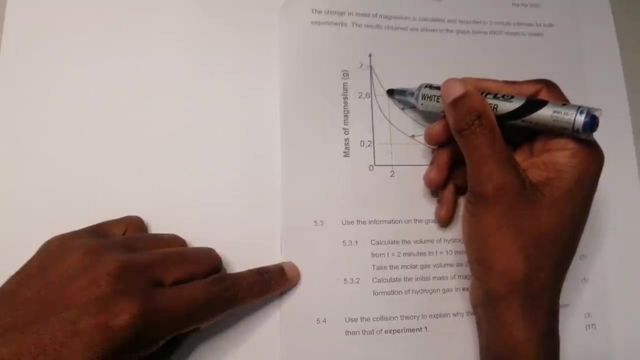 experiment one. so now let's look at it from the graph. okay, i want you to please stay with me, ladies and gents. so now experiment one: what is the volume? or rather, what do we know from the graph? we know that the mass of zinc at two minutes right was 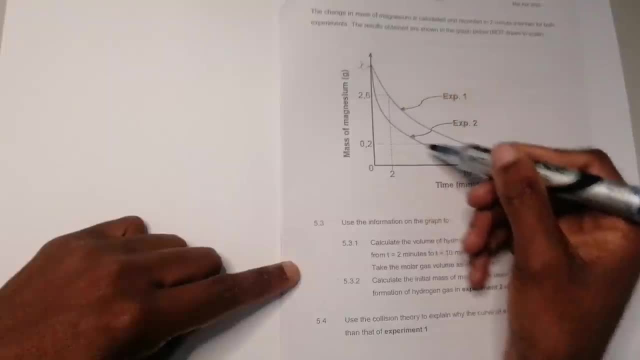 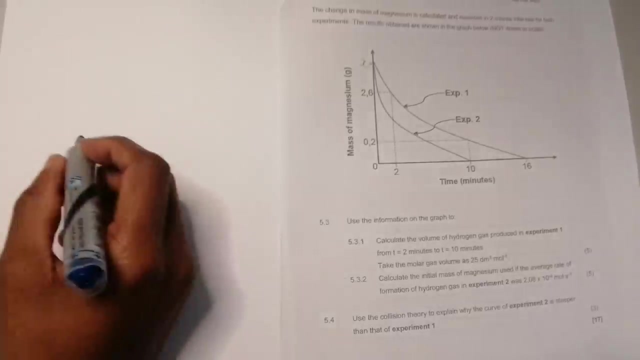 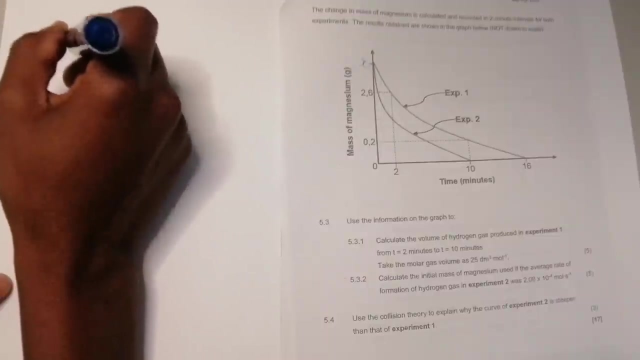 uh 2.6, and the mass of zinc at 10 minutes is 0.2. so what is the amount? what is the mass of zinc that was used between those minutes? so the mass of zinc- sorry, did i just say zinc magnesium, sorry about that- so the mass of